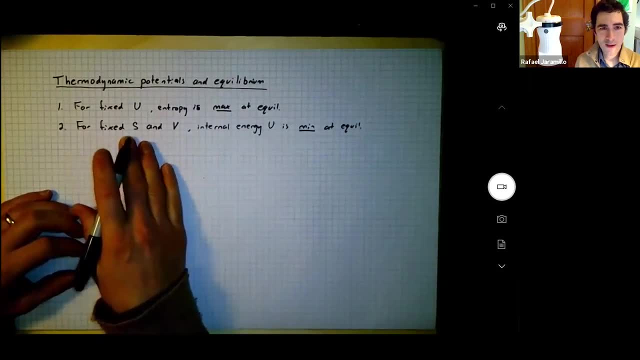 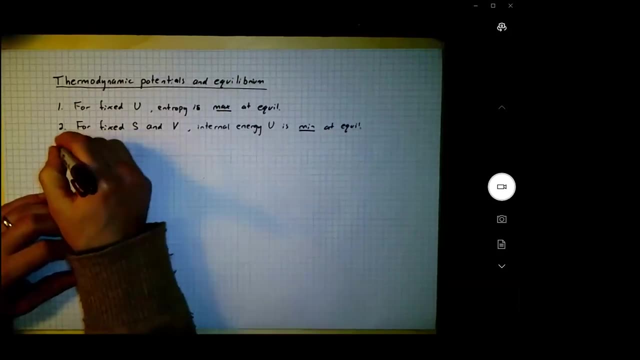 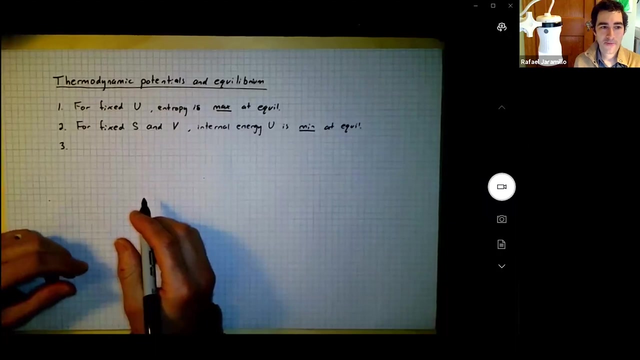 Anybody? is there any? is there ever really a way to fix the entropy their way? How can we fix the entropy? There's no entropy reservoir. We can't. we can't connect the system. We can't do an entropy reservoir like we can with a pressure reservoir or temperature reservoir. 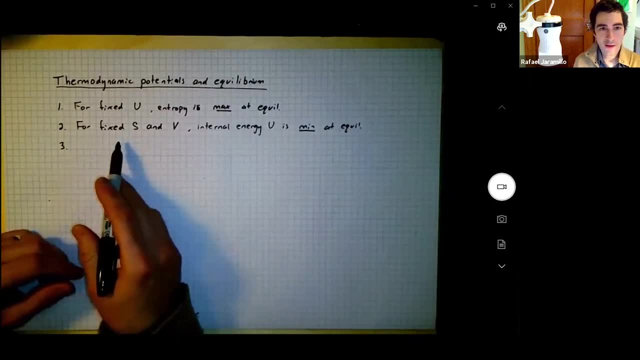 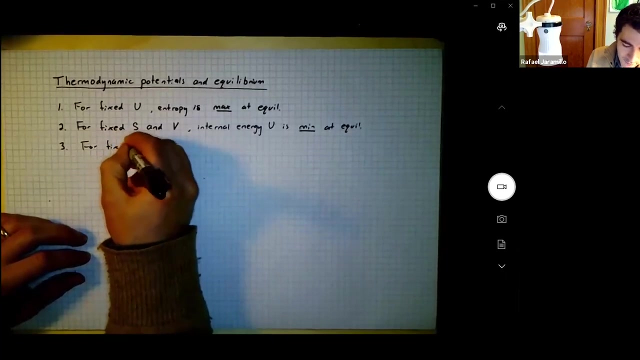 So I'll tell you it's a little bit of an aside, but the only way to fix entropy is to be at zero Kelvin. When you're at absolute zero, there's no entropy. So the physicists like it down there, But for the rest of us it's not terribly useful. OK for For fixed. 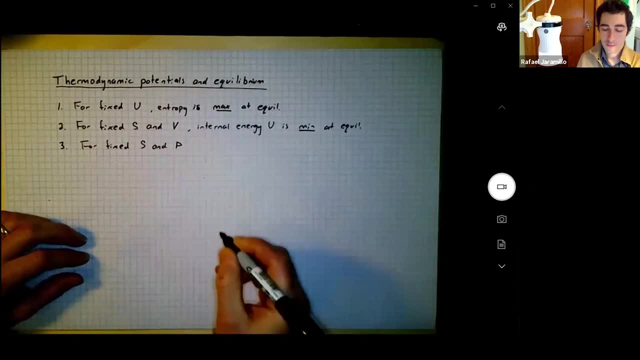 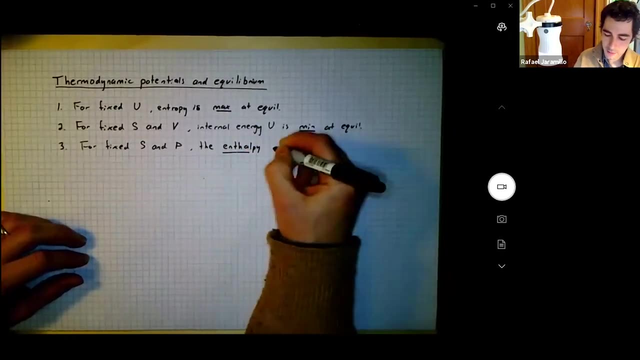 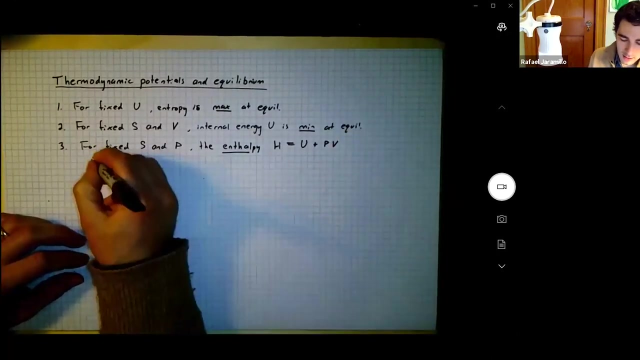 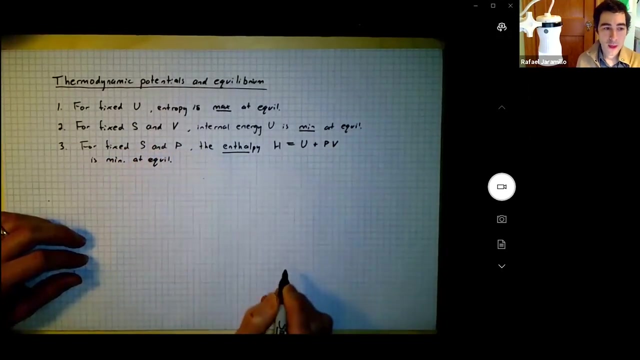 S and P- New term here- The enthalpy H equals U plus PV Is minimized Equilibrium, So that's enthalpy. This condition- minimum enthalpy and equilibrium- is not terribly useful, but the enthalpy. 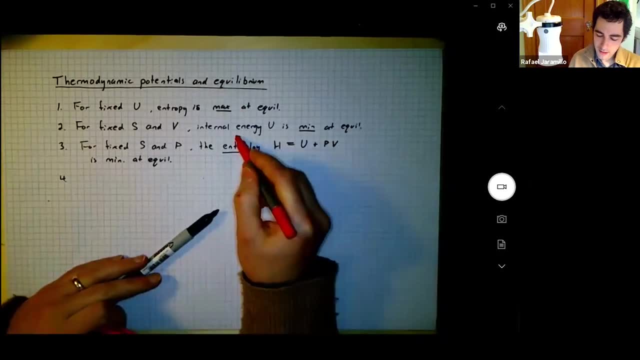 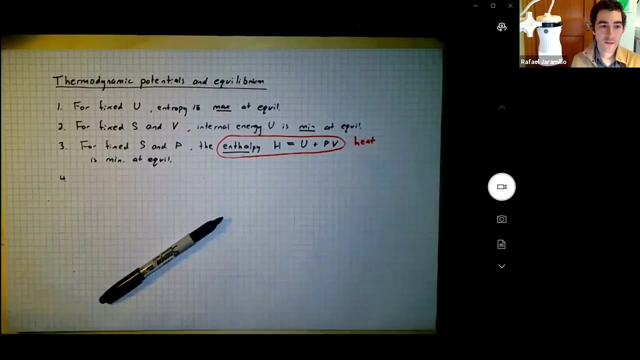 Is useful. It's a useful thing, And one of the problems on the current piece that is making connection between Enthalpy and the heat of a process. Sometimes those terms enthalpy and heat are actually used interchangeably. That's not strictly correct, but you'll see why. 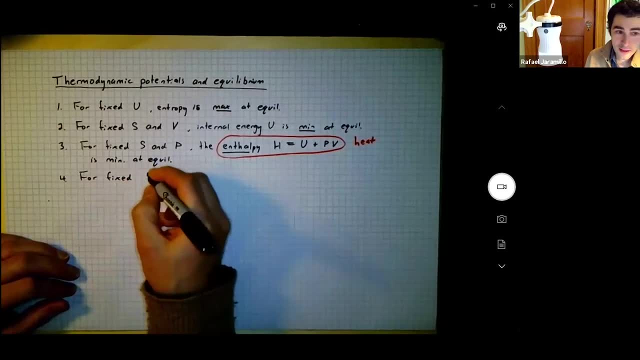 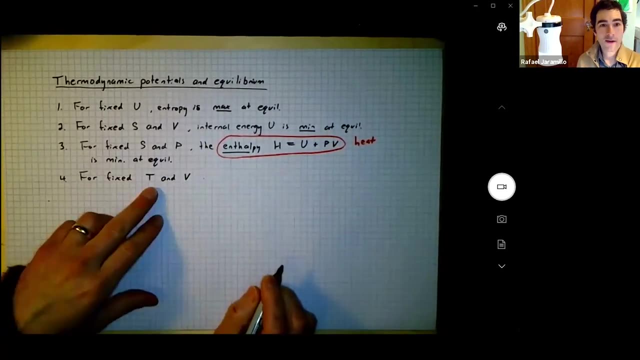 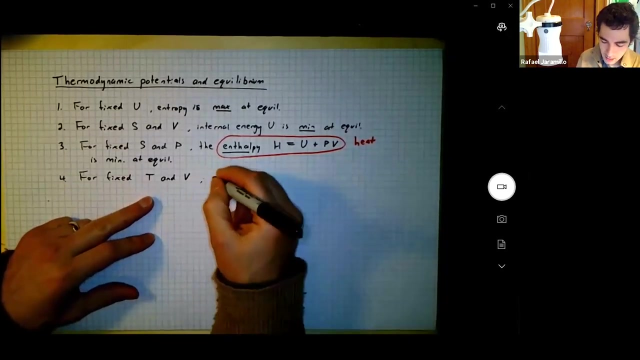 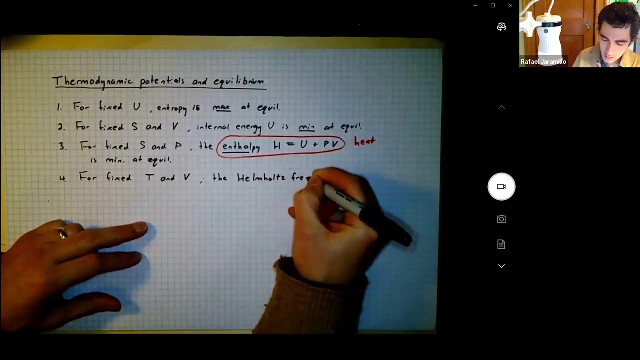 OK, More perfect temperature And volume, So. So now we're getting a little more practical right. Fixed temperature. That's something we know how to do. We all have thermostats. That's what your thermostat does, The Helmholtz. 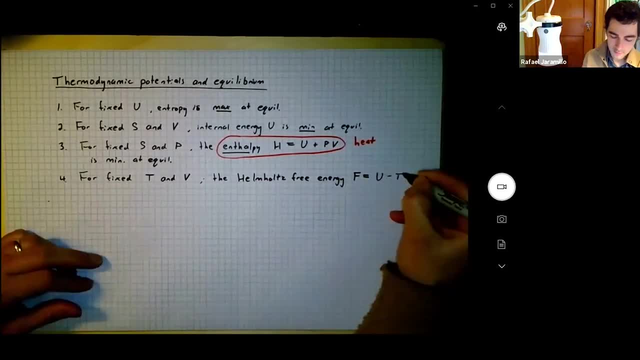 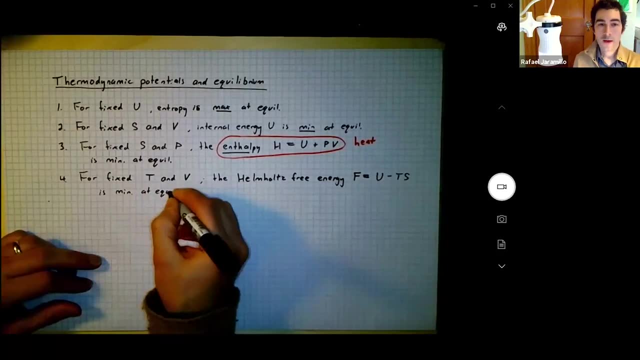 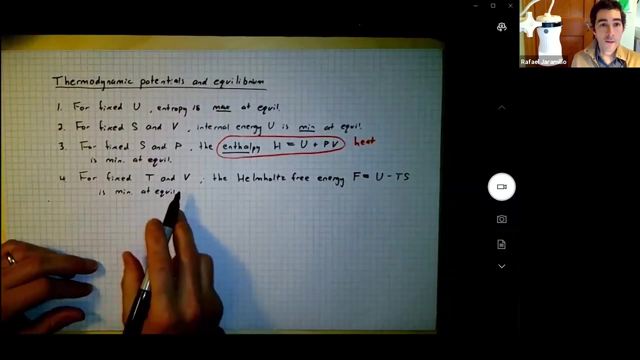 F equals U minus, TS Is min And equilibrium. So I'll tell you, we spend almost no time at all on Helmholtz in this class, because fixed temperature and volume Are much less practical and useful than fixed temperature and pressure. 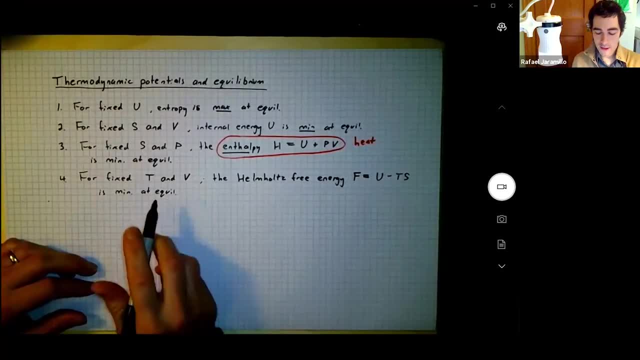 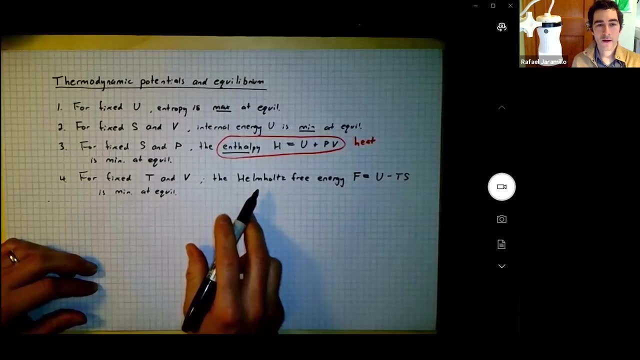 For materials processing. however, in other disciplines, especially in semiconductors and semiconductor physics, it's the Helmholtz free energy that matters, Because your your device is typically operated at a fixed temperature and your electrons are confined in the volume of the semiconductor. 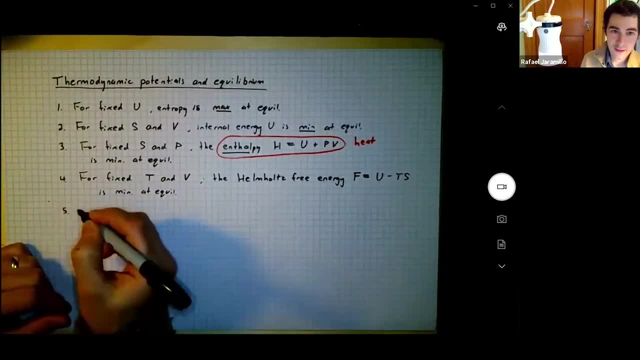 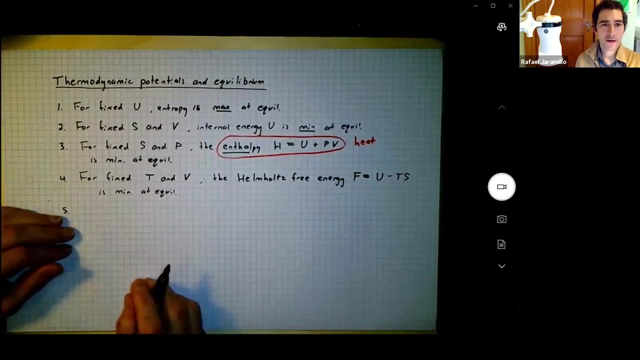 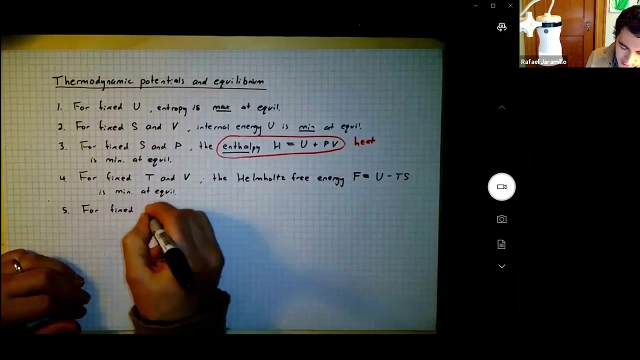 So if we were to do things like calculating the theoretical limiting efficiency of a solar cell, we'd be worrying about Helmholtz. But as it is, you'll almost never hear us discuss that at all in the rest of the class. This is the one that matters. 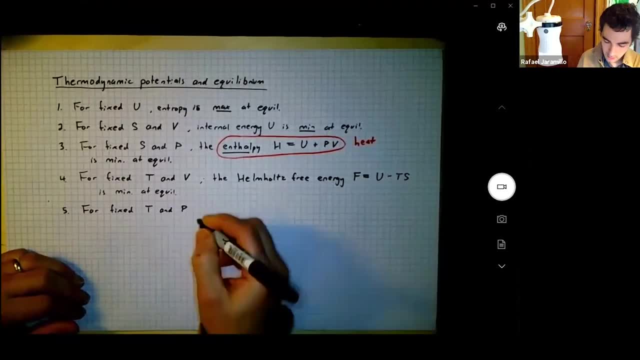 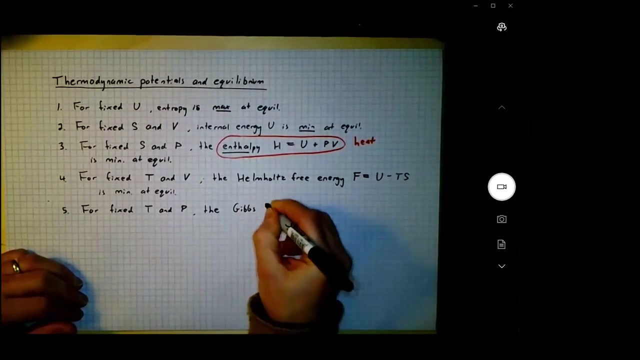 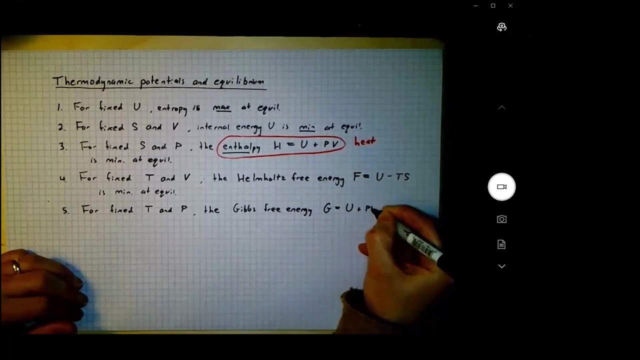 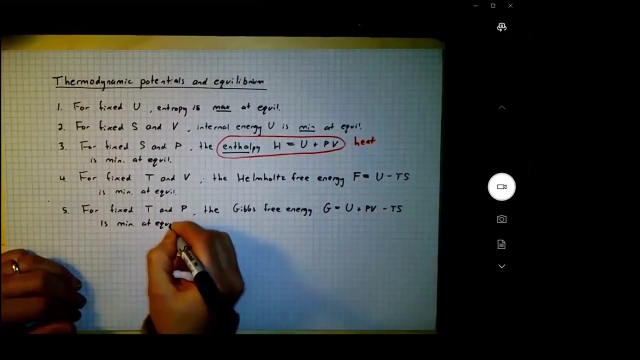 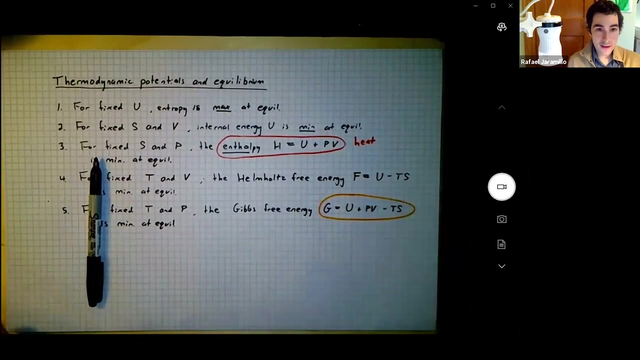 For fixed temperature and pressure. anybody know what's the relevant potential for these conditions? Who's right ahead? Yeah, Yeah, Yeah, Yeah, Yeah, Yeah, Right, So this is the one that matters for materials science, And one way to see the rest of this class, actually the rest of the term. 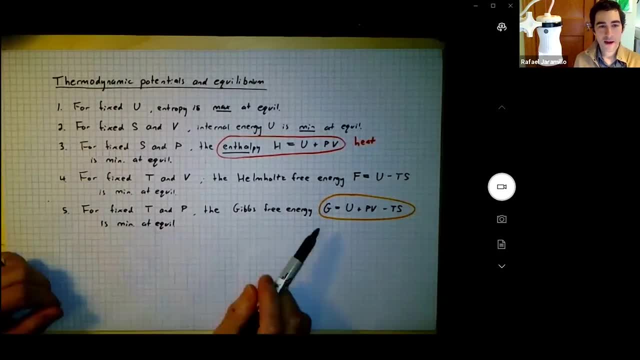 Okay is: we're just calculating the Gibbs for different scenarios And we're doing price shopping for Gibbs. I call it: We calculate the Gibbs free energy for different scenarios and we choose the lowest one as the equilibrium case. Okay, so that is. thermodynamic potentials. 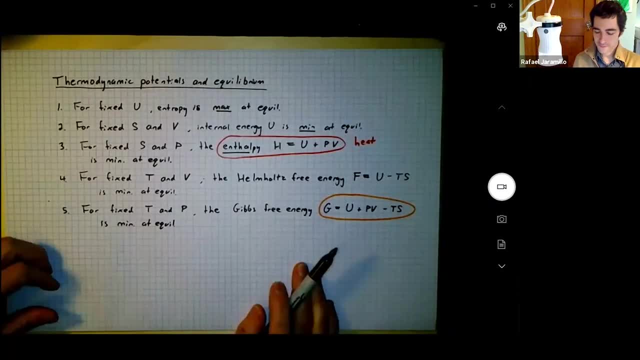 Now these are presented without proof. It's not worth the time here to motivate each and every one of those On the P set. you're going to convince yourselves that, given this, then this. So one of the exercises is going through a form of proof of this. 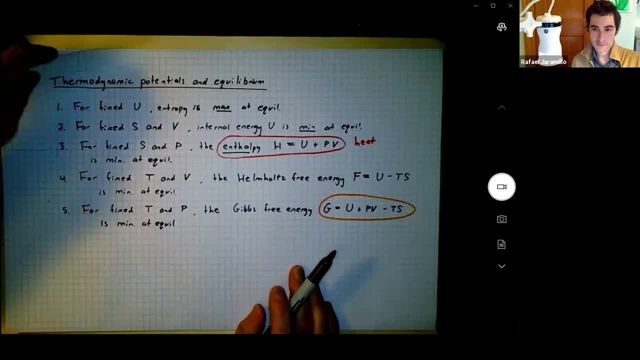 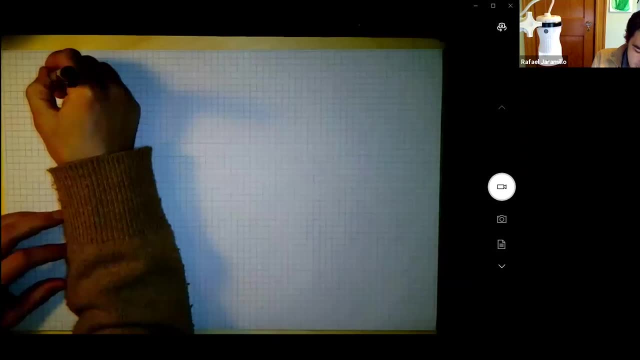 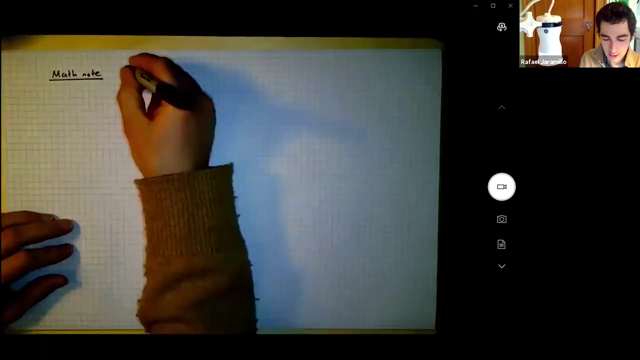 And that's useful, because Gibbs is the one we care about. Now I have to make some mathematical asides, because I don't know if you're familiar with this. I don't know if you're familiar with this. I don't know if you're familiar with this. 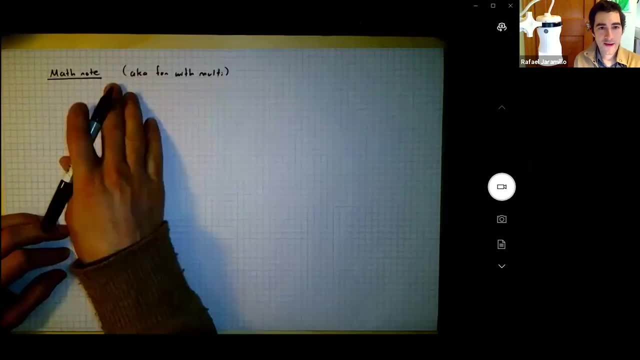 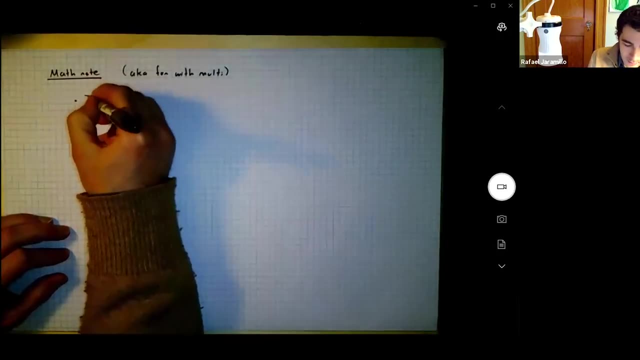 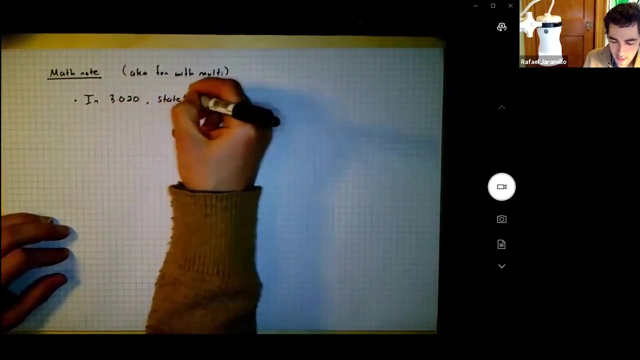 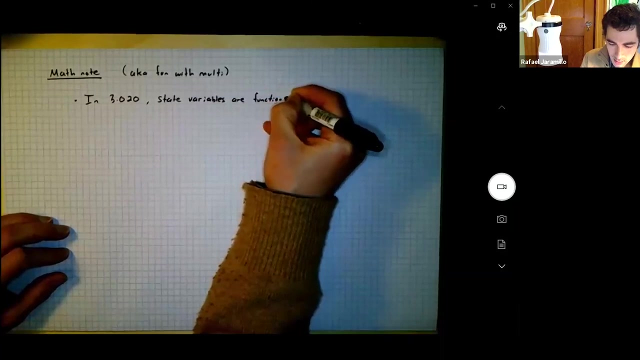 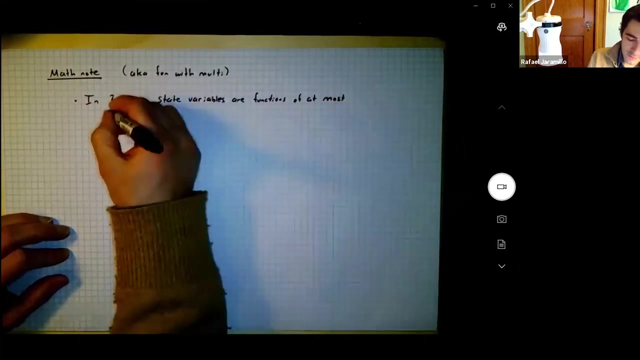 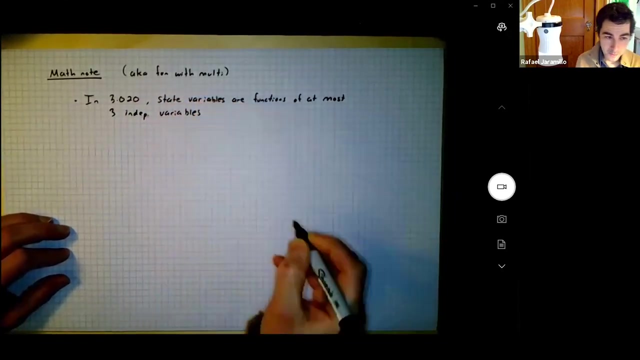 Without this, my math note, a lot of what comes is kind of weird and confusing. So in 3.0.2.0, state functions, state variables. They're functions of at most three independent variables And those three independent variables. 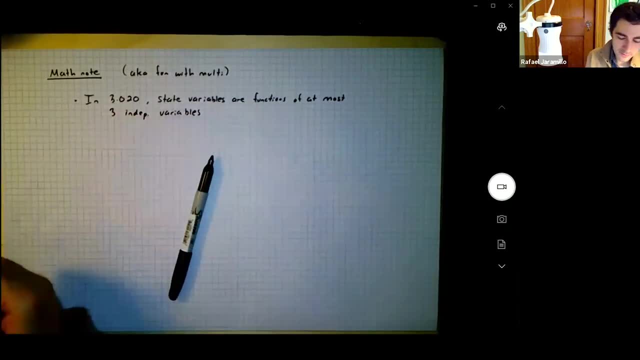 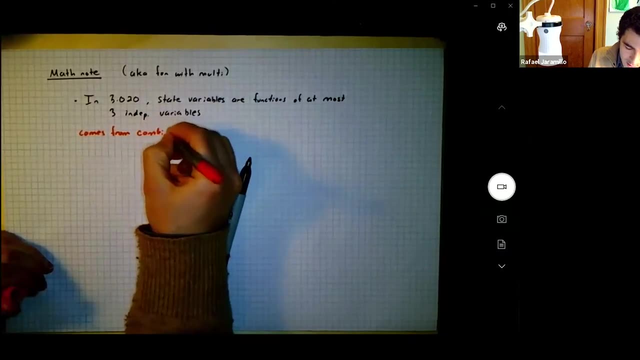 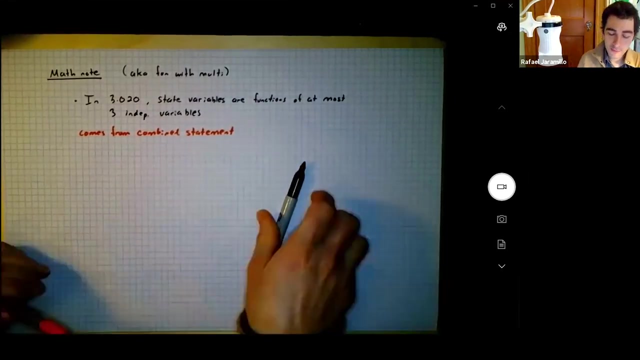 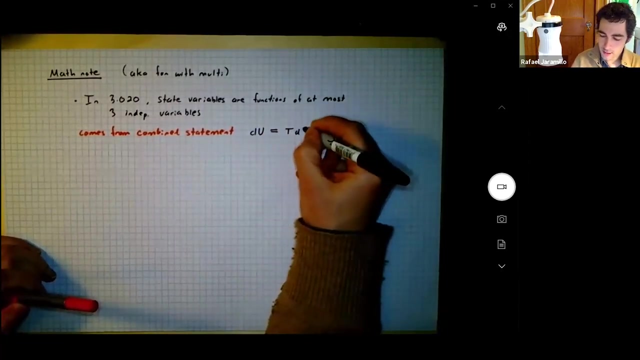 And this is where that comes from. It comes from- sorry, this pen is kind of smushy, It doesn't come from nowhere. It comes from the combined statement, So it comes from physical reasoning. All right, DU equals TDS minus PTD plus mu DN. 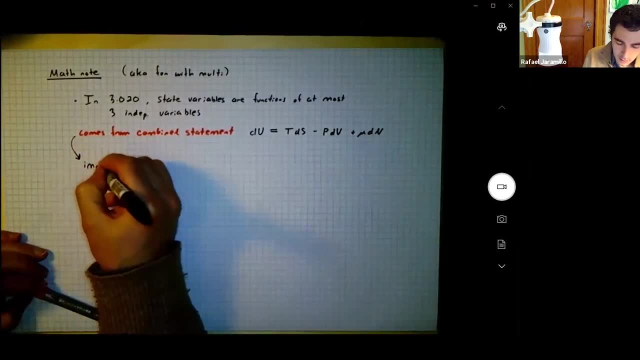 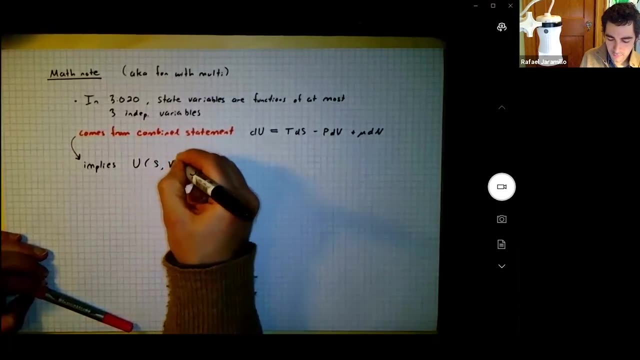 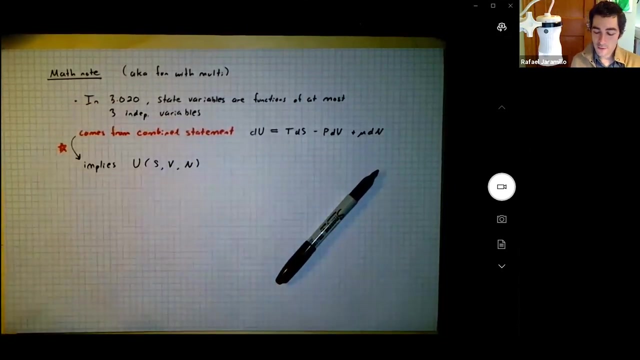 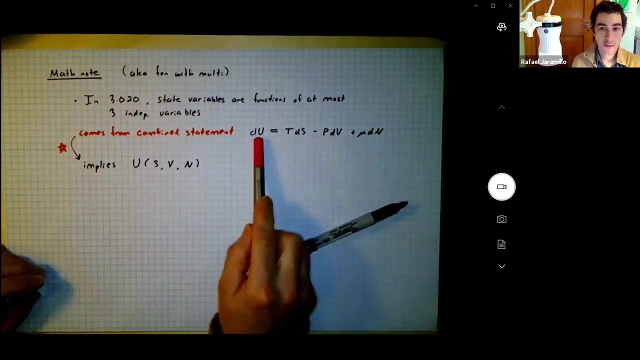 This implies the existence of a state function. U is a function of SV m. This is a critical link here. If you write down a differential form, we're going to learn how to identify the independent variables, the coefficients and the dependent variable. 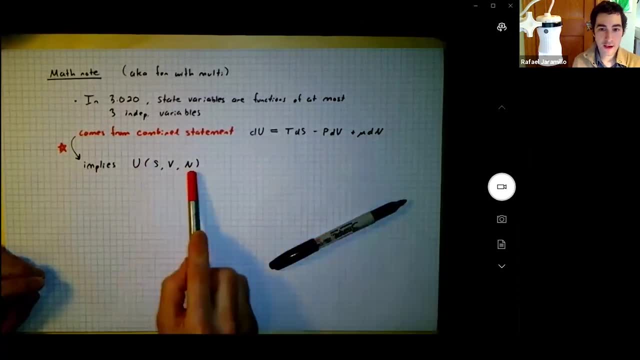 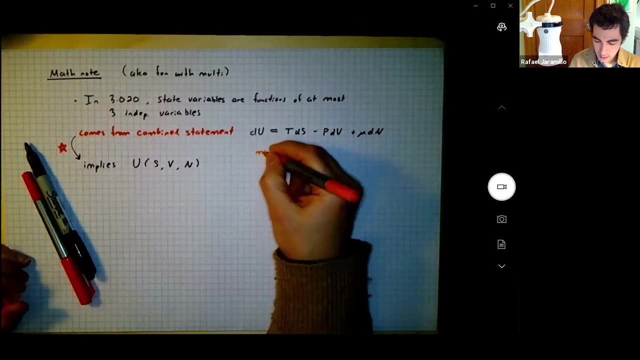 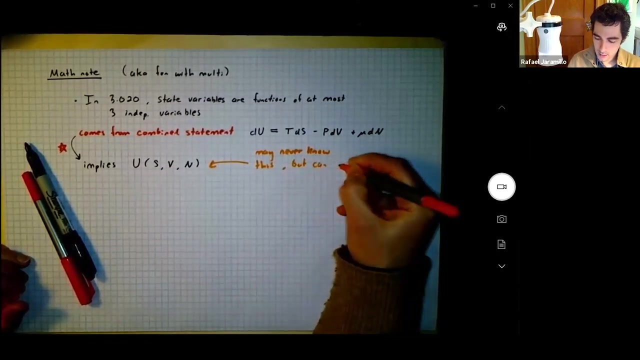 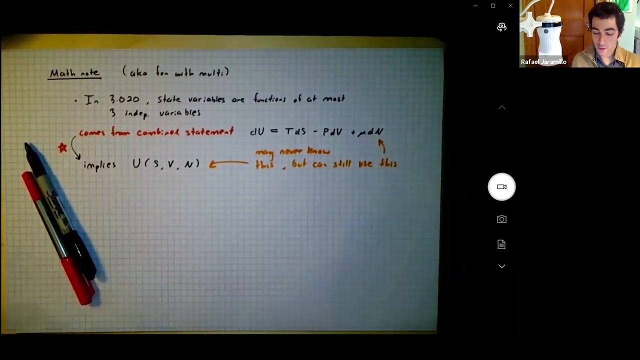 and the existence of this differential form implies the state function. Now, in most cases, we may never know this, but we can still use this. That is, we may never know the closed form of the state function, but we can still use its differential form. In fact, 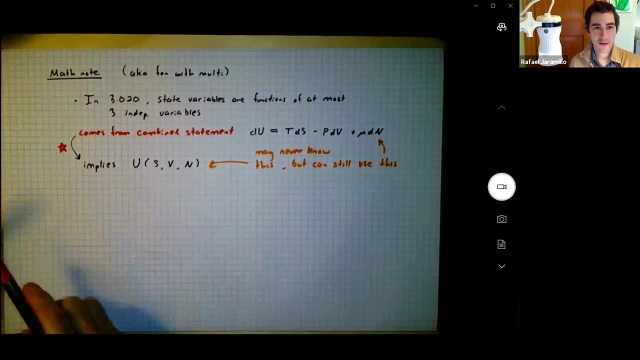 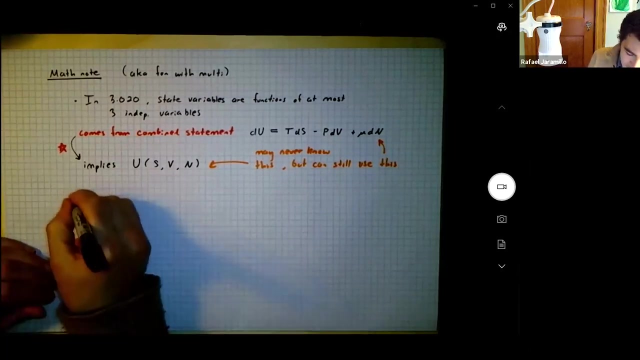 outside of the ideal gas situation. we almost never write down any state functions in this class. You can't find a complete state function for something useful like a high-entropy alloy. It doesn't exist, It's too complicated. A corollary of this is that thermodynamic potentials 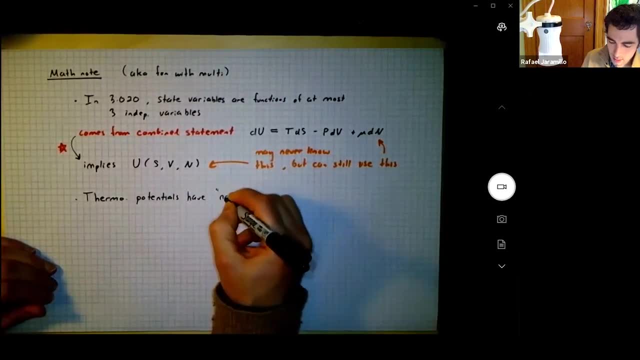 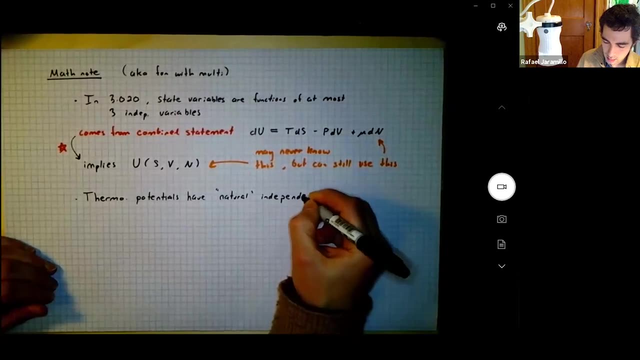 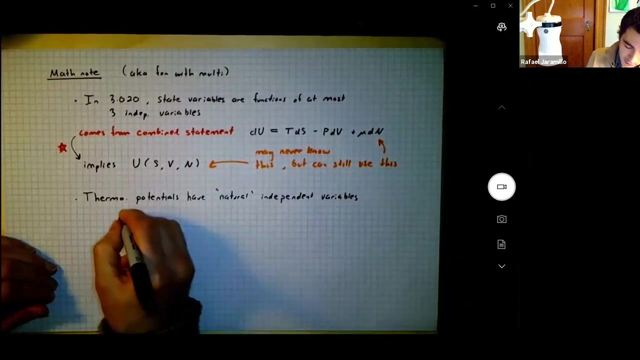 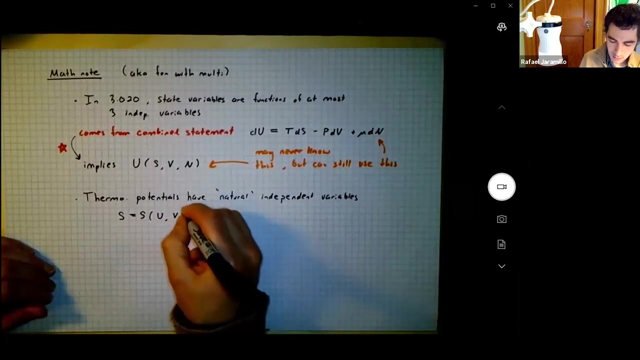 have what I'll call natural independent variables, which we will see aplenty in the case of Gibbs. So, for example, entropy is a function of energy and volume. If you remember, at equilibrium entropy was max for fixed energy and fixed volume. 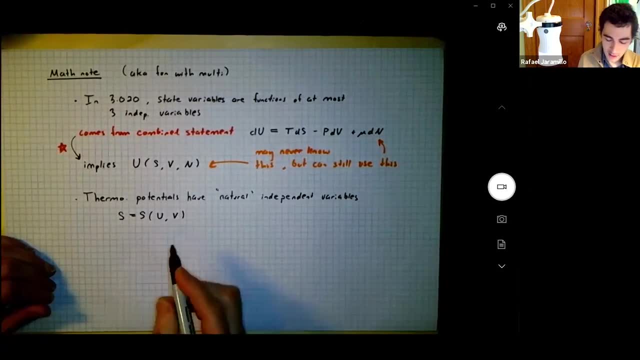 That tells you what you're going to get. Those are its natural variables. At equilibrium, internal energy was maximum for fixed entropy and volume. Those are its natural variables. Enthalpy was equilibrium for a minimum of equilibrium for fixed entropy and pressure. 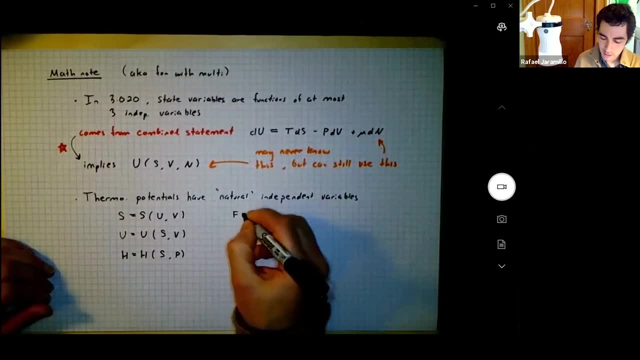 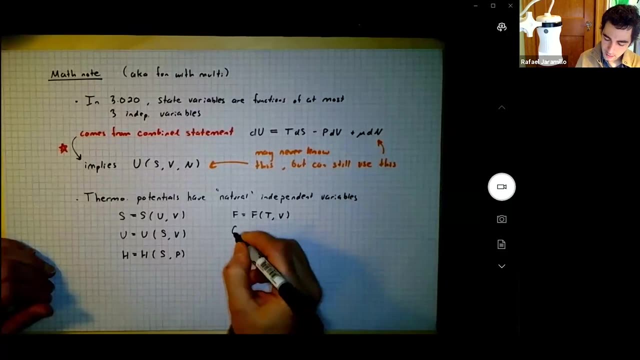 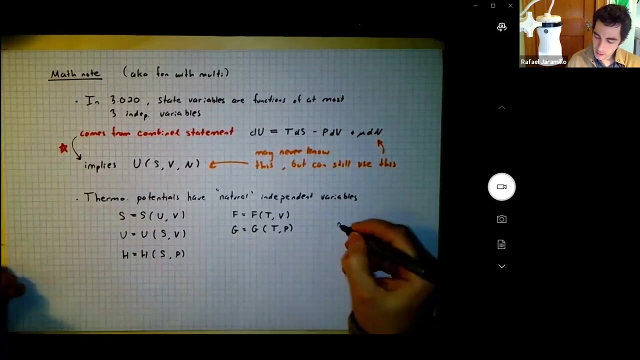 Those are its natural variables. For Helmholtz its natural variables are T and V, And for Gibbs its natural variables are T and P. Before you ding me here, I'm not writing the n's for compactness. So everything is also a function of the size of the system. 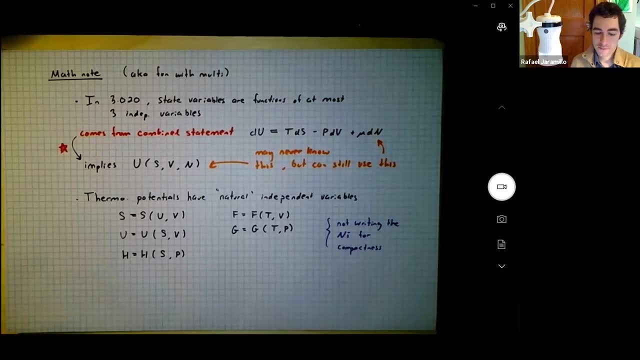 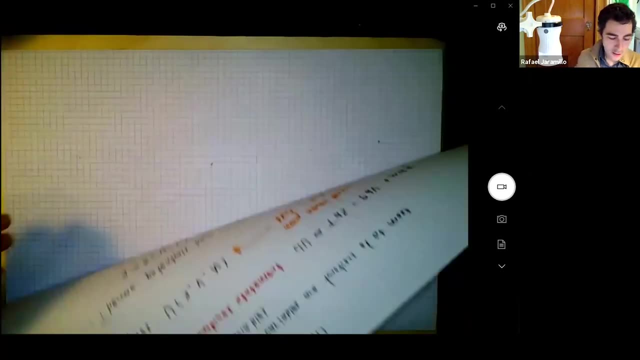 I'm just leaving that off to keep the lines short. I'm just leaving that off to keep the lines short. I'm just leaving that off to keep the lines short. Okay, one more note. Where on earth does this stuff come from? 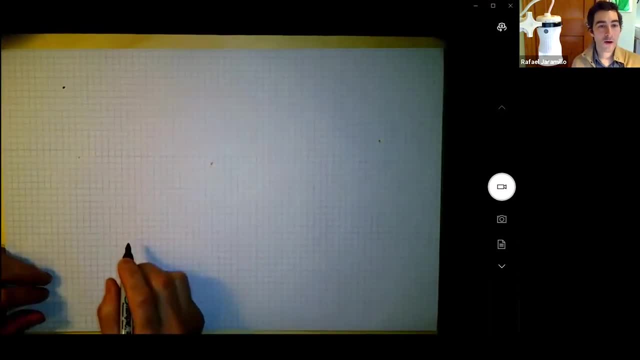 When I learned thermo, these potentials were just told to me the way I just told them to you, And I think in the back of my mind I said: where does that come from? And then I forgot the question and I didn't come back to it for years. 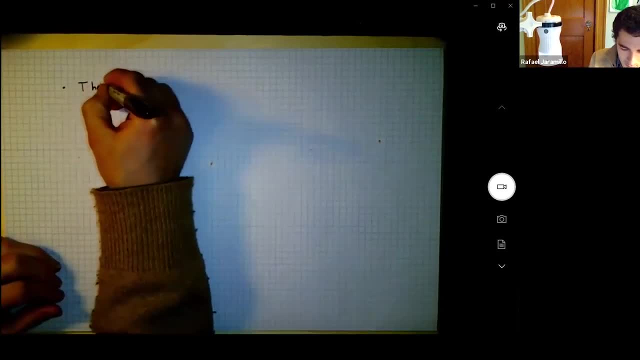 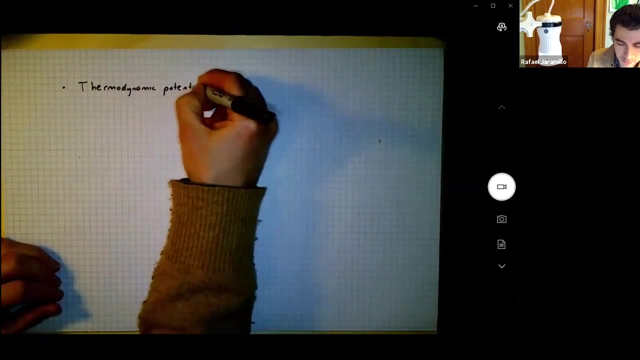 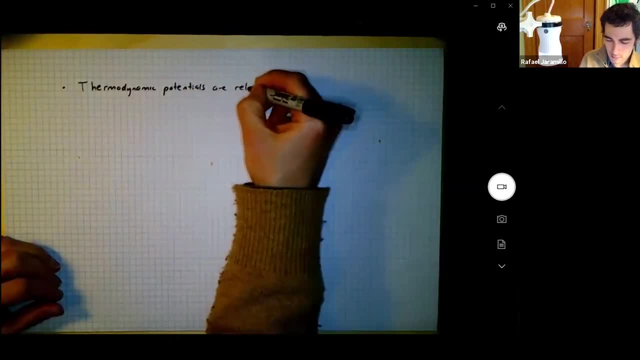 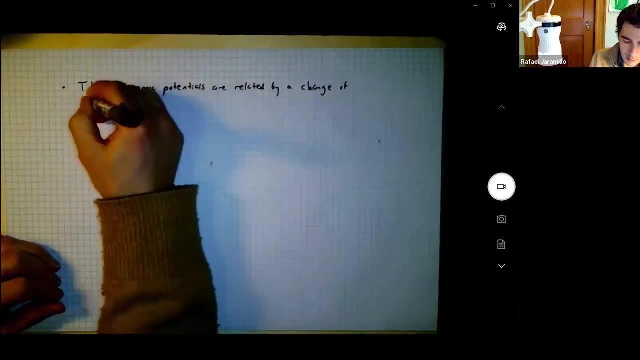 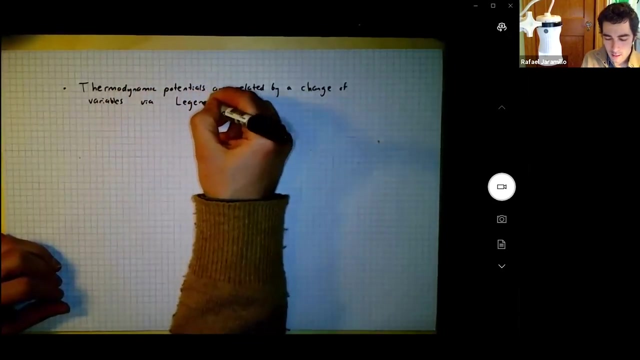 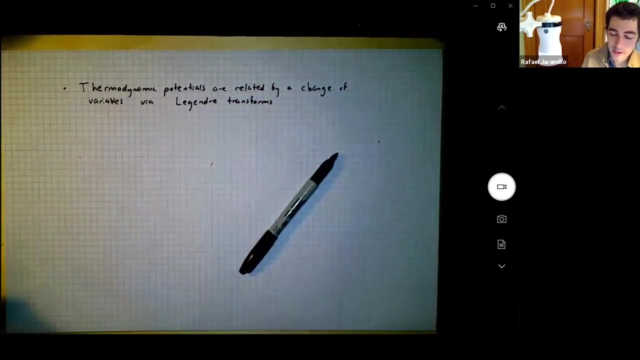 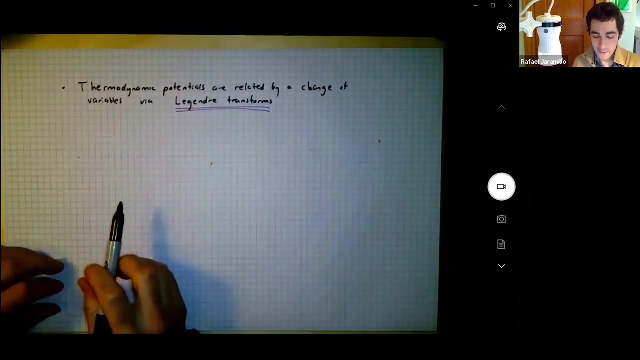 Okay. Potentials are related by change of variables via the genre transforms, So this is something we don't have time for in this class, and probably I wouldn't be able to teach very well anyway. This is the math concept, And so for those of you who've seen Legenda transforms in your math classes, that's great. 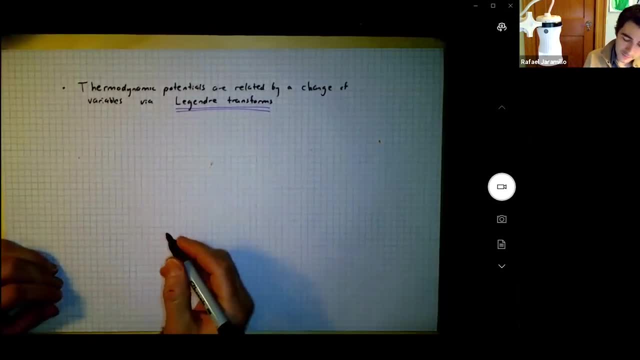 For those of you who are curious, you can start with the wiki entry. We're not going to cover it in detail. You can think of it as just one more type of a transform, like a Fourier transform or Laplace transform. The Fourier transform, for example, changes your natural variables from time to frequency. 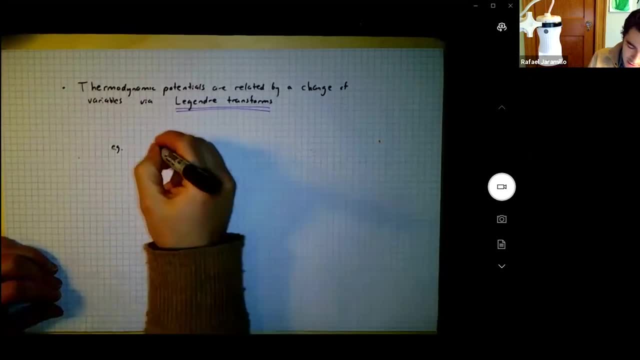 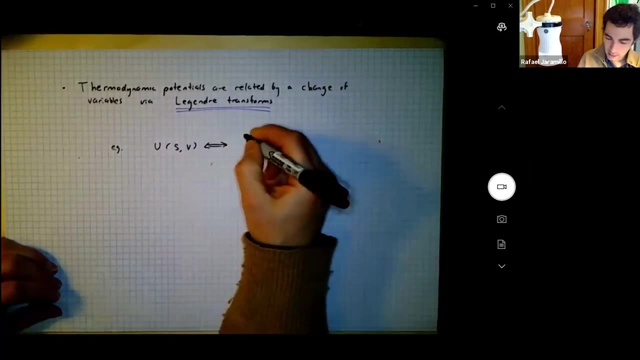 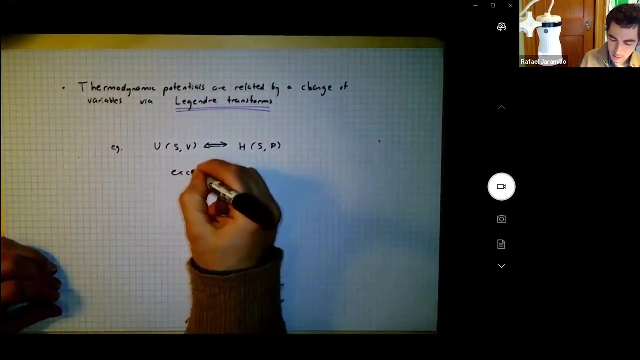 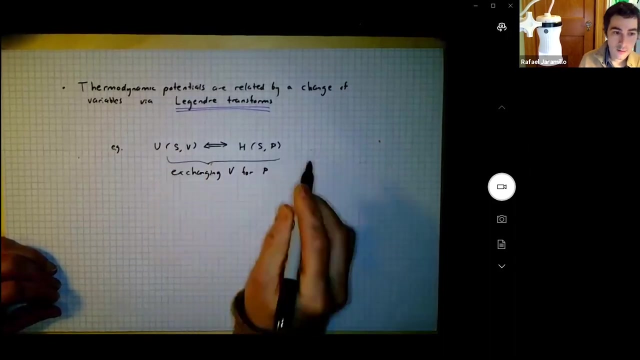 That's an example. Legenda transform will change natural variables, for example, from u as a function of s and v to h as a function of s and p, exchanging b for p. And, if you remember, h equals u plus pb. 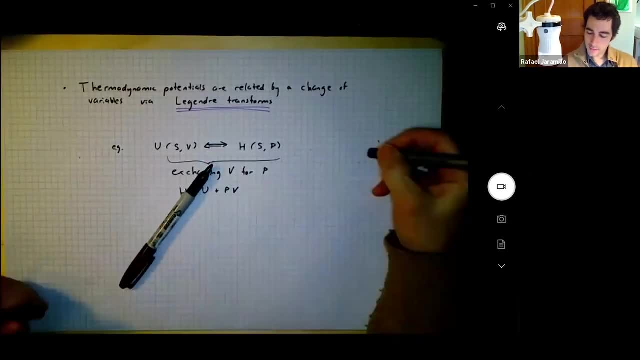 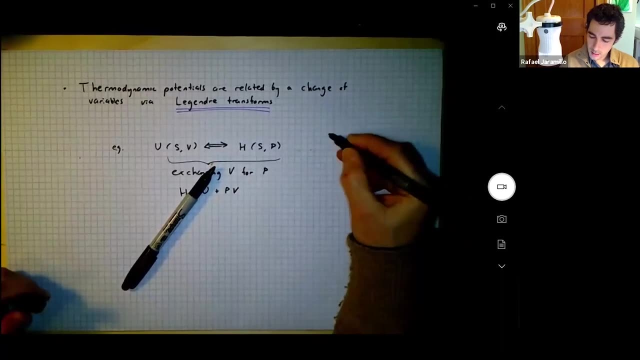 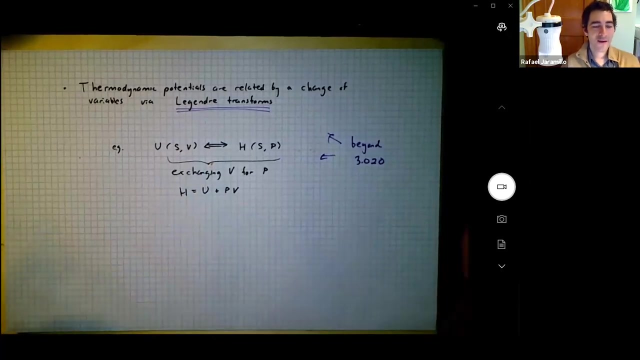 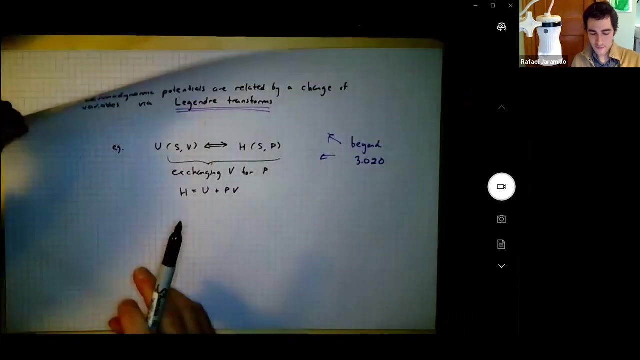 And this comes from somewhere. This is all beyond. This is beyond O2O. I just wanted you to know it comes from somewhere. It comes from somewhere For most of the class you can just memorize. OK, I'll dive in a little more. 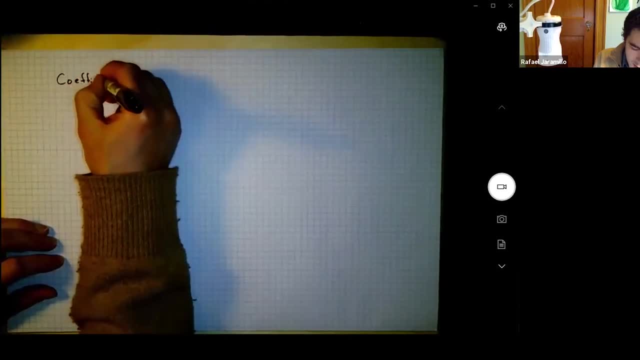 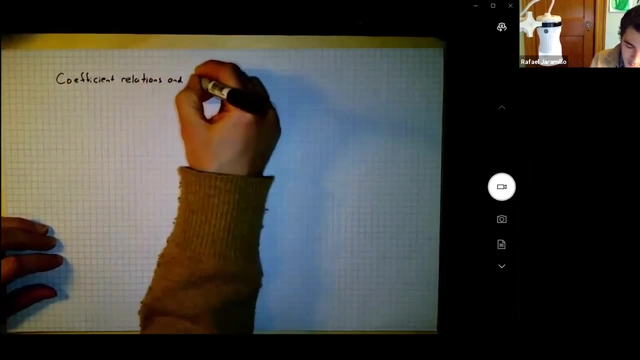 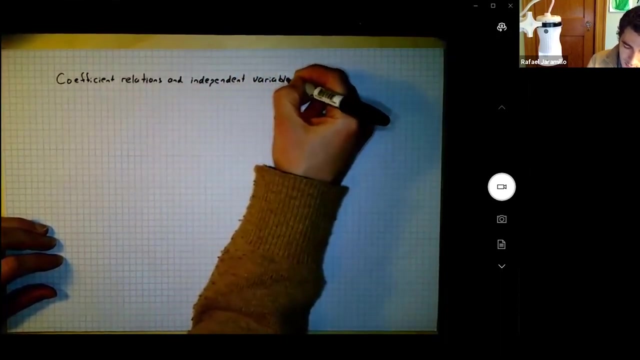 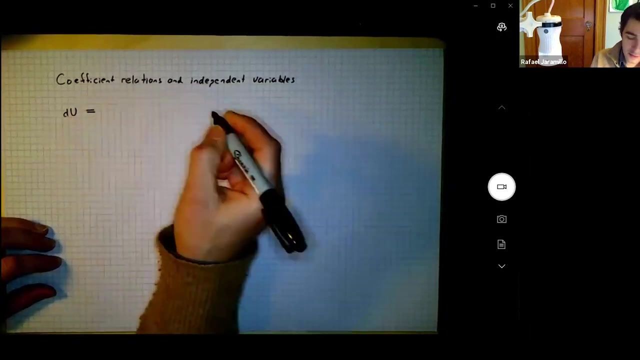 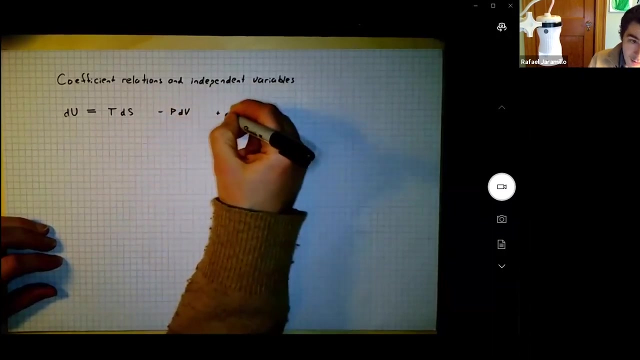 OK, I'll dive in a little more. All right, Let's start with the combined statement: du equals t, ds minus p, dv, dv plus mu. I'll let this be a multi-component system, so I'll keep the labels there. 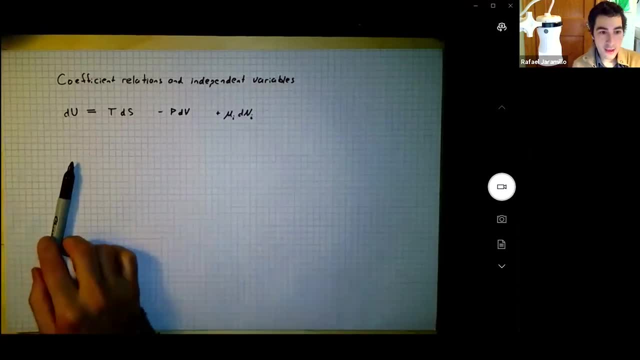 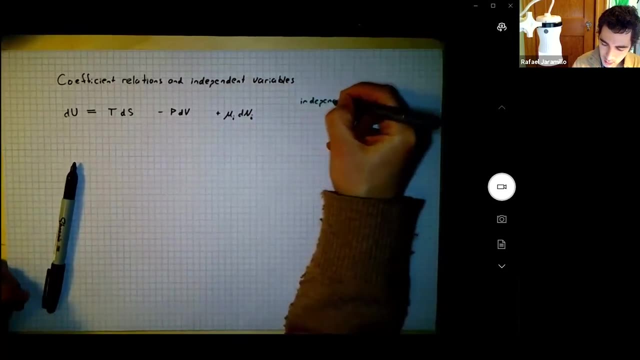 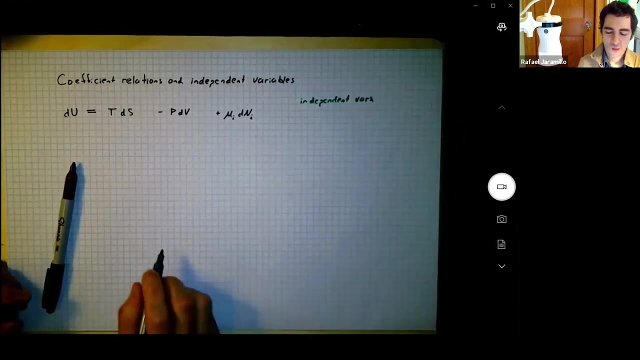 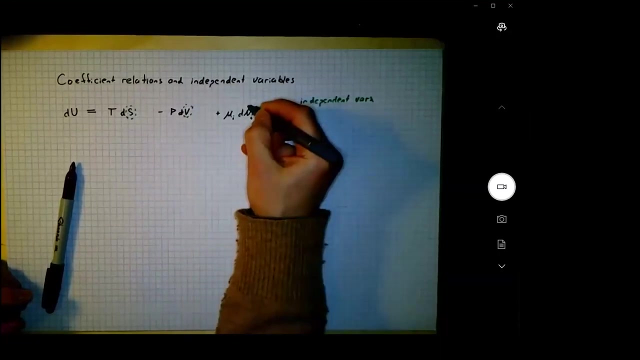 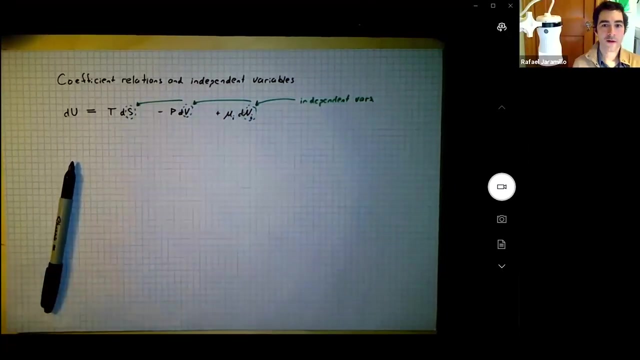 OK, Somebody please remind me what are the independent variables in this differential form: s? v and ni, s v and ni, Right? Those are the independent variables, right? The other things we call? I'm having fun with colors today. 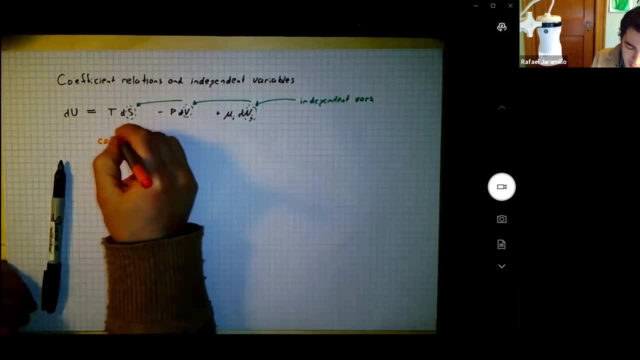 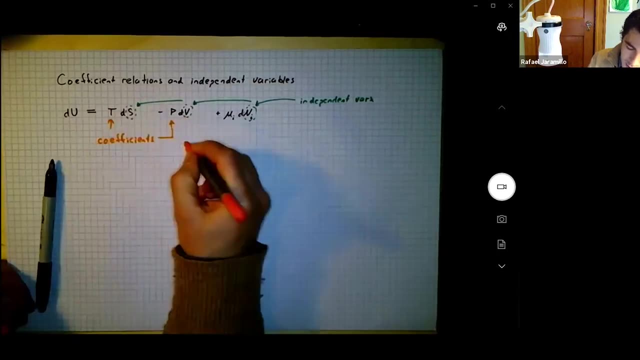 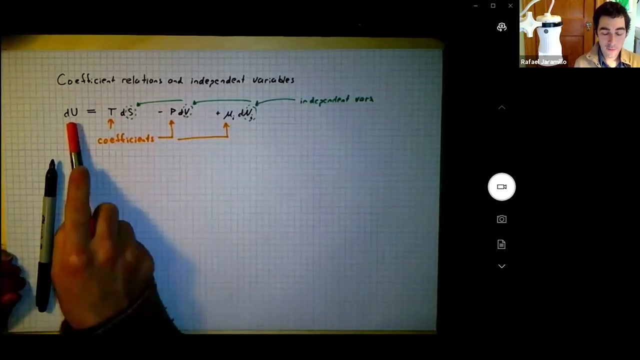 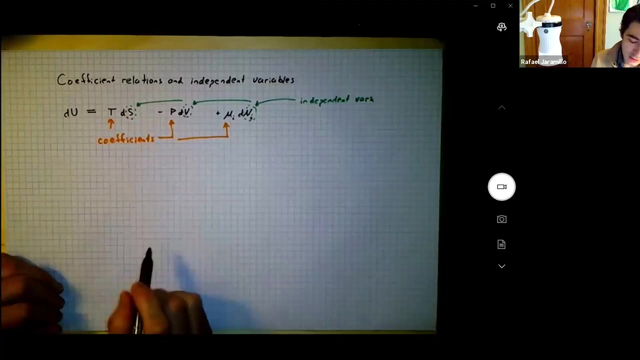 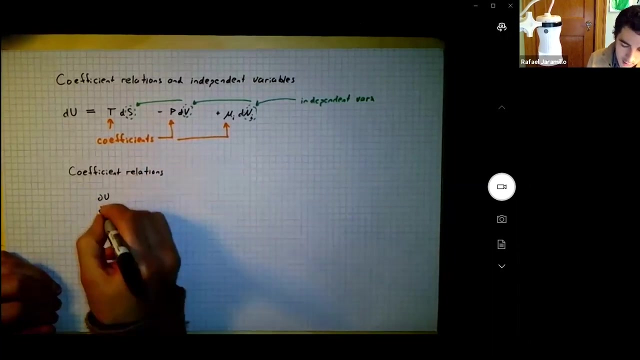 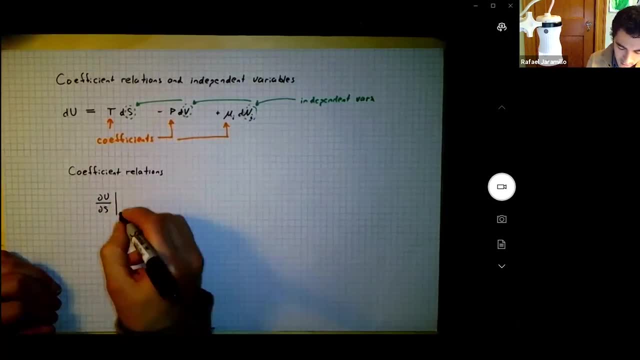 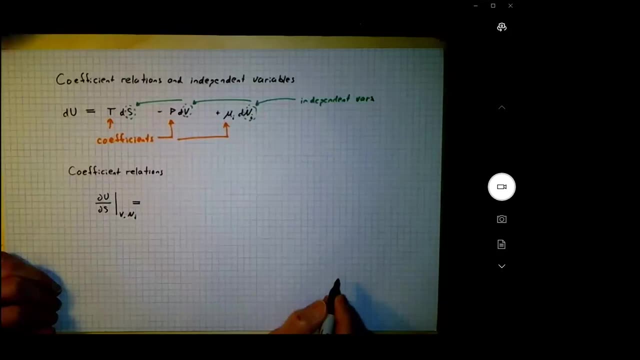 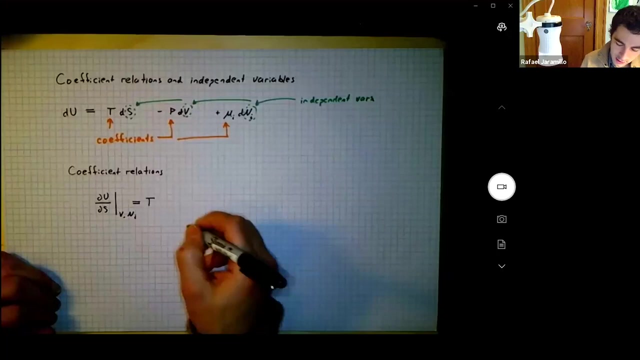 At fixed volume and fixed particle number equals what? What is partial U by s? You can pick it off of t, t. Yep, you just look at the equation sketch in front of time and it's off: du dv at fixed entropy and particle number equals minus p. 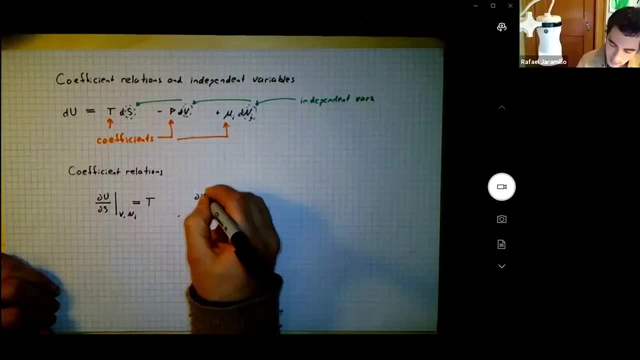 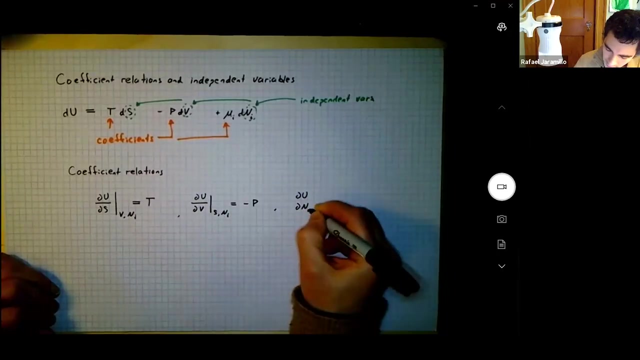 Yep, p and d u d n. i at fixed entropy volume and particle number j not equal to i equals mu, i. These are coefficients, They're called. you can call them O, I just picked partial differentials, but they're called coefficient relations. A lot of problem-solving in thermo comes down to calculating. 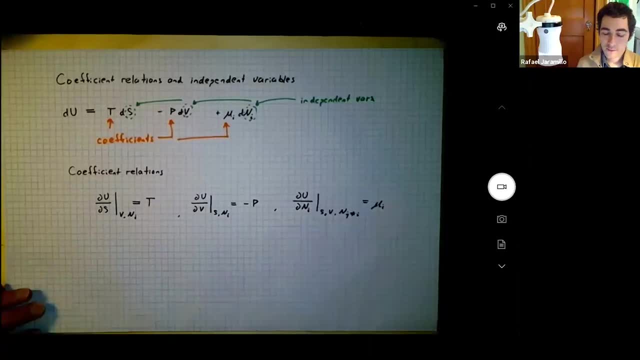 these coefficients. The most useful chapter- actually in the chapter 10 of the book, the most useful chapter- is chapter 4.. If you read only one chapter of this book, take chapter 4,, because it contains all the things we need to actually solve the problem. 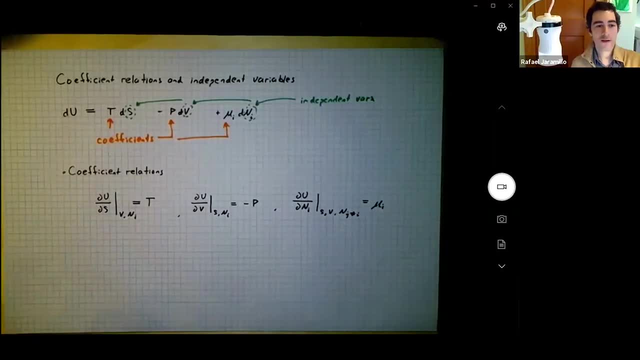 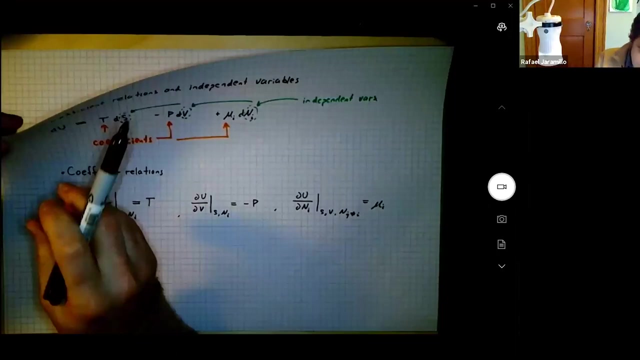 To actually solve problems. you just have to understand chapter 4.. And I say just, it's actually one of the hairier chapters, but there it is, And it's all about these coefficient relations and identifying independent variables and calculating coefficients. So let's see how to do that. I wouldn't call it a strategy. I think it's a little. 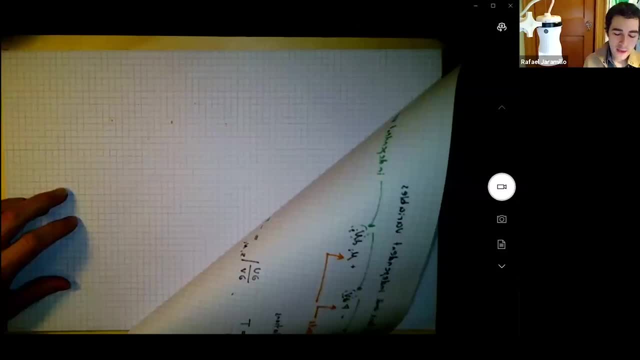 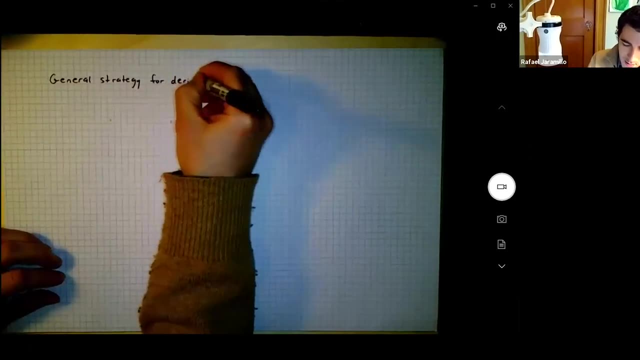 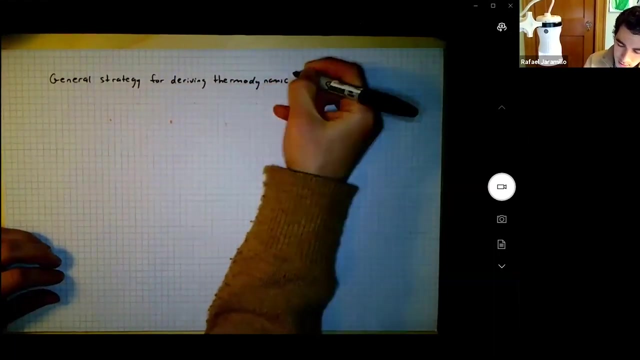 funny. besides, it's a tactic, not a strategy, but that's what it's called in DoHOP, so I'll stick with it. The general strategy for deriving thermodynamic relations is really best illustrated by an example, so that's what we're going to do. 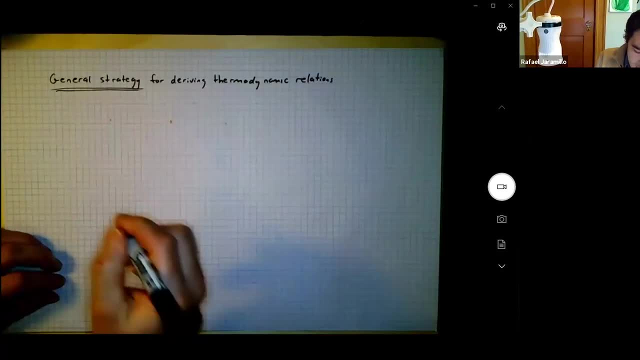 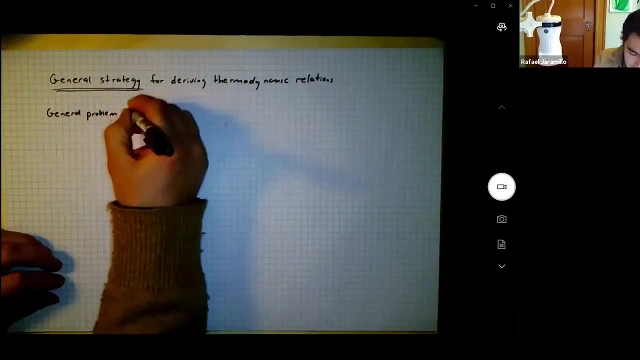 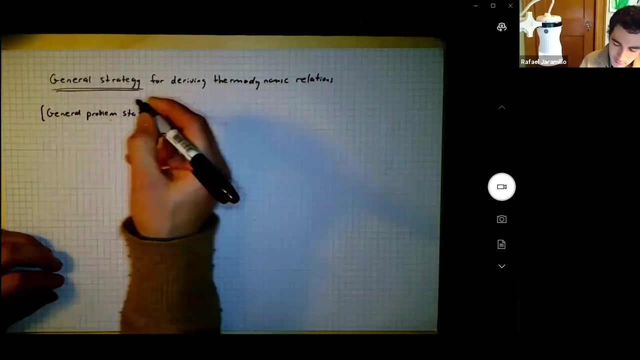 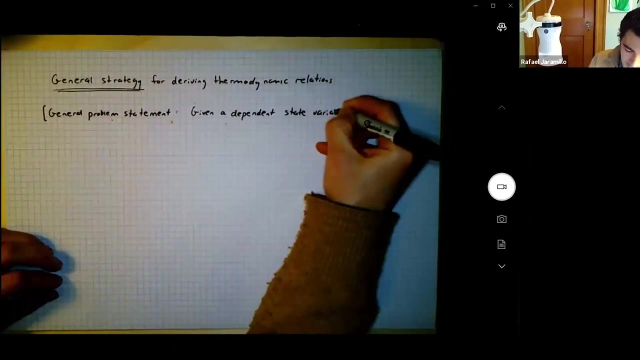 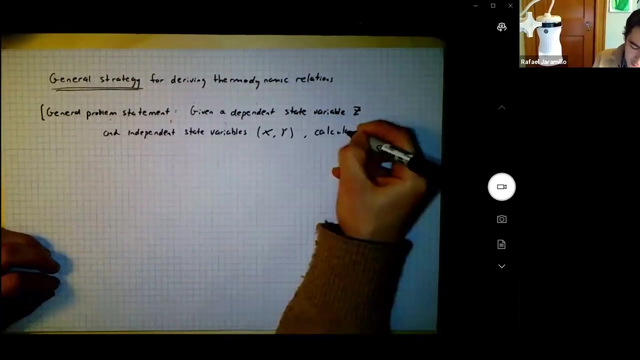 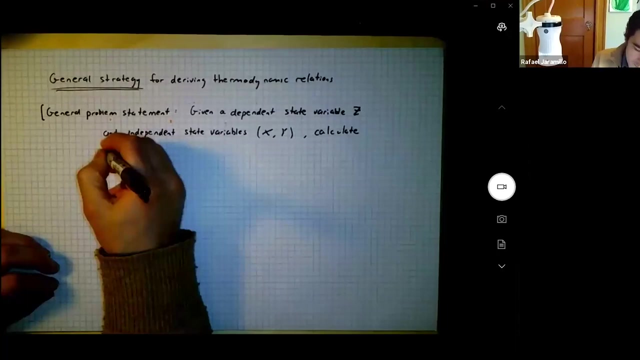 Here is the general problem, the general problem statement: Given a dependent state variable z, independent state variables x and y, calculate right. so this is a you know a word problem: delta z for a given problem. So this is like you know. 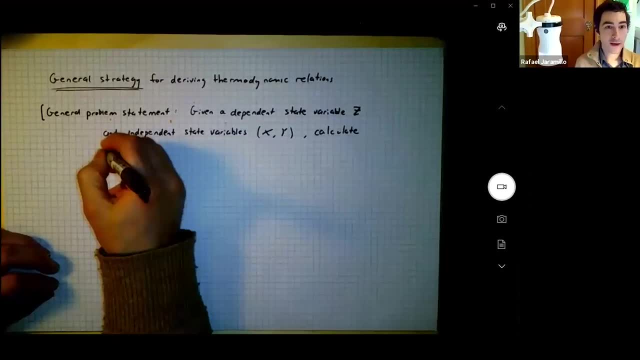 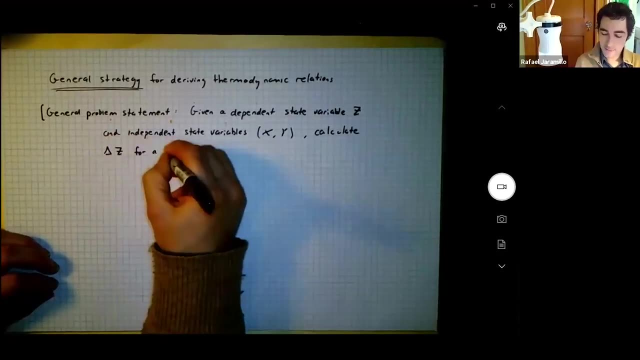 probably half of all thermal problems boil down to something like this: There's some dependent state variable which you identify through the problem statement. There's some independent variables which usually you're not told. You figure them out through the problem statement or the situation at hand and you want to calculate the change for a given process. 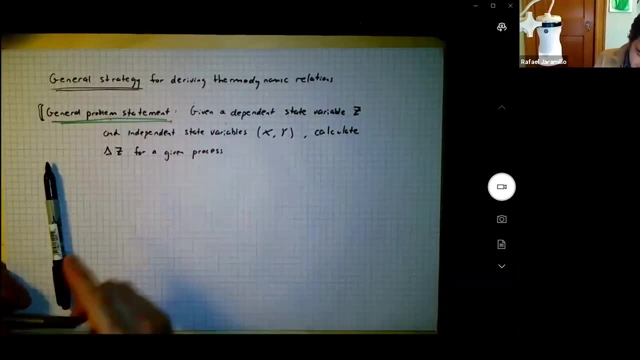 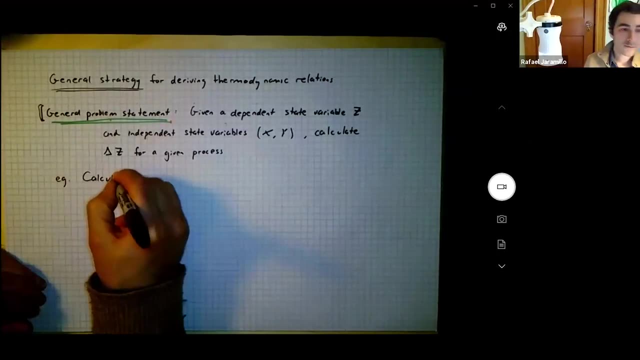 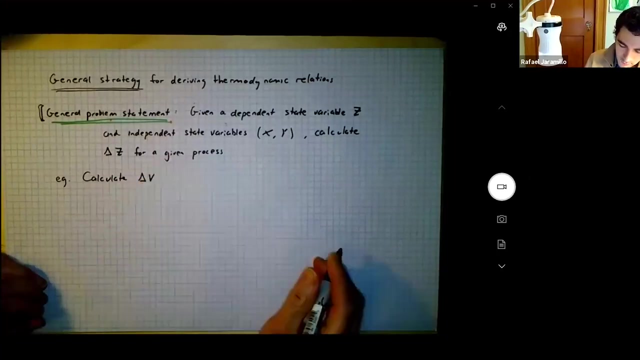 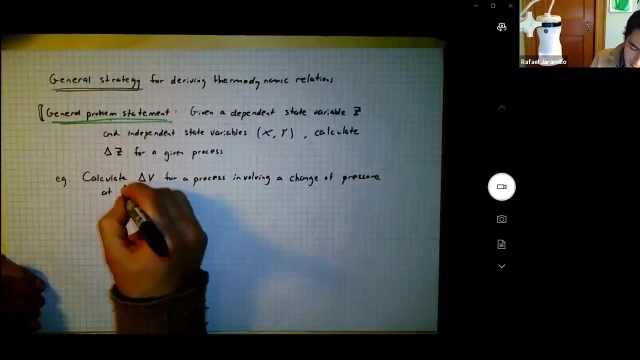 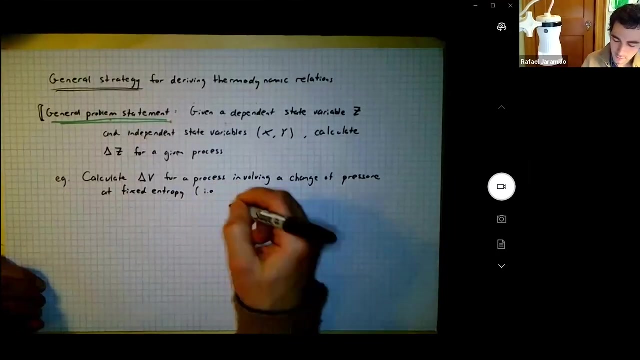 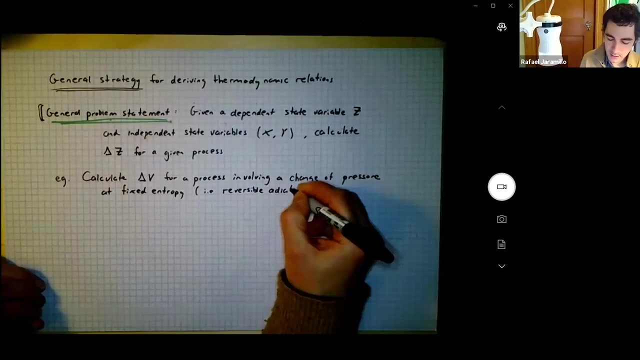 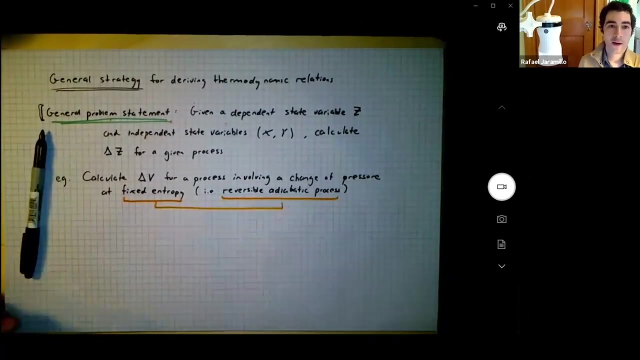 So what example are we going to do? Example: calculate delta v for a process involving a change of pressure at fixed entropy, which is also is a reversible adiabatic process. This is helpful, Remembering that fixed entropy and reversible adiabatic processes are related. that's really helpful. 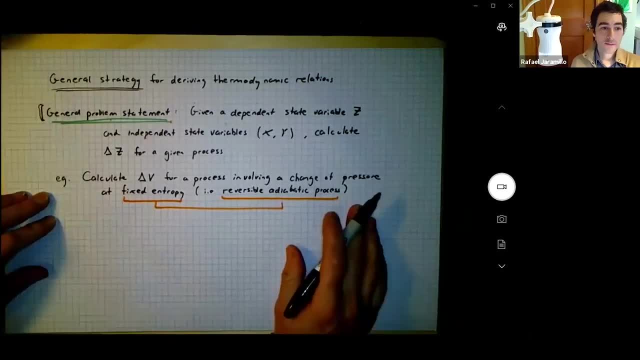 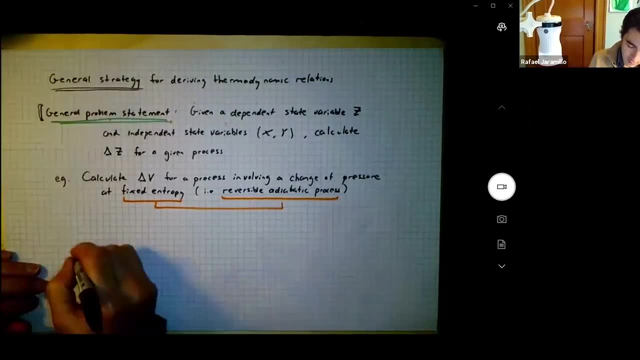 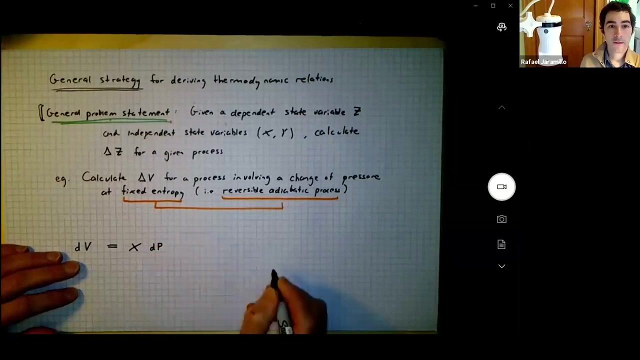 Okay, so now I'm going to step through this example. We want to write down the differential form of the change in the dependent variable, and this is going to depend on some coefficient times dp plus some coefficient times ds, And our job is to find. 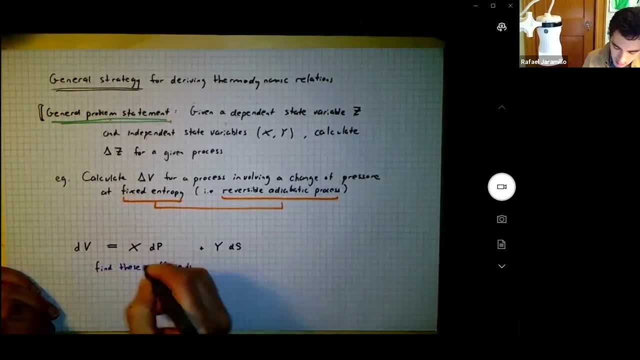 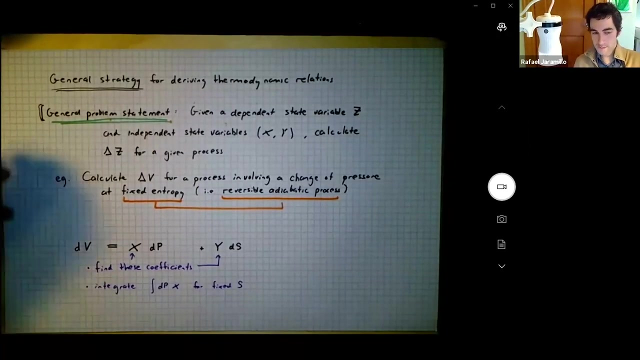 yang we want: to find those coefficients and then integrate. right, This is the. this is the approach. Once you find these coefficients, then you can integrate this term which, for fixed entropy, gives you the thing you're looking for, which is the change in volume. That's what we need to do. Questions before I go on to actually. 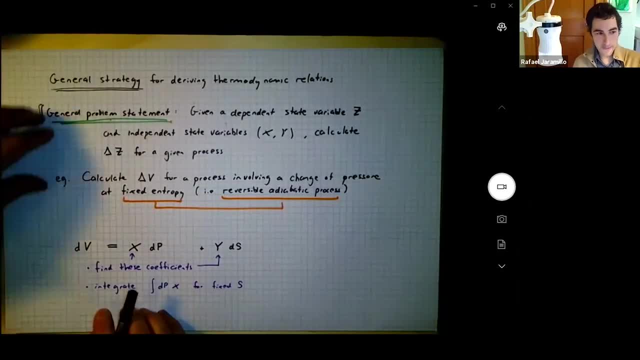 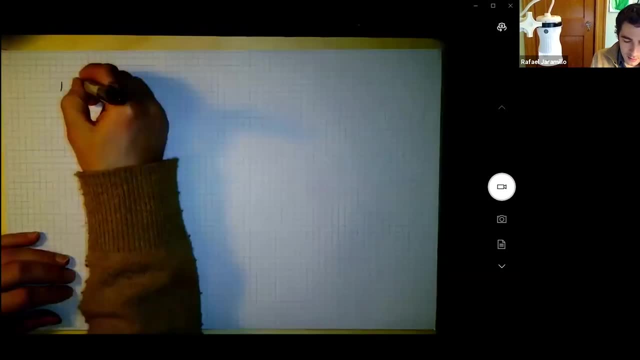 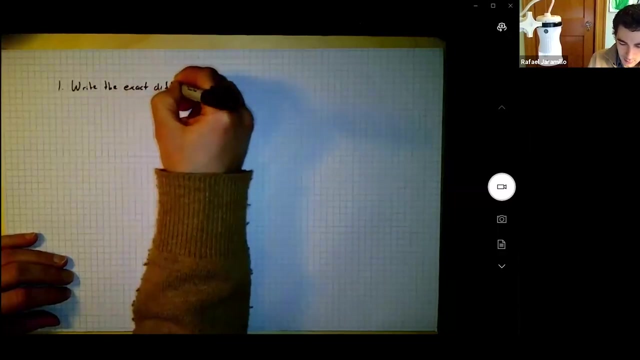 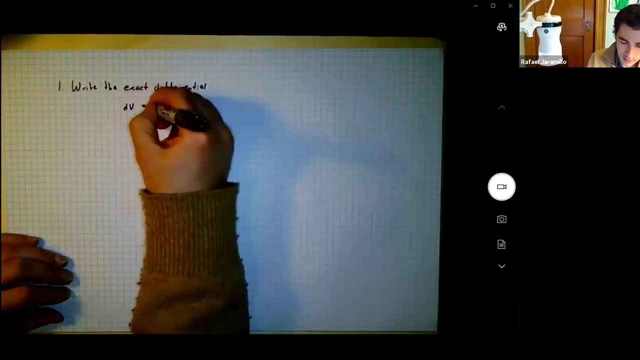 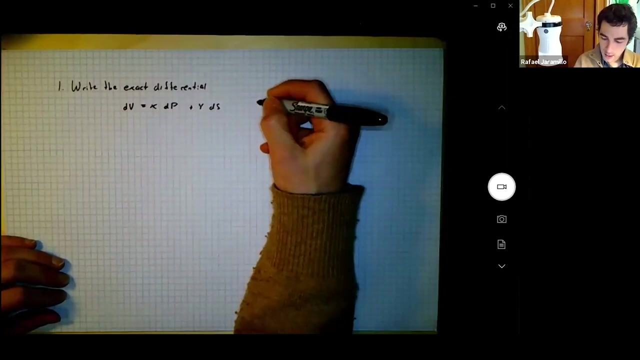 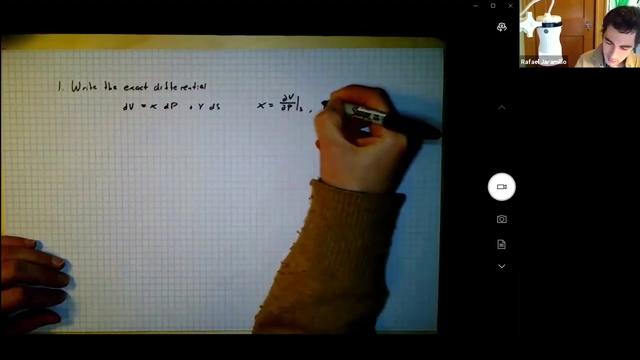 do that. Okay, We're gonna start One. We're gonna write the exact differential, Rewriting what we did right. DV equals x DP plus y E S. x equals DV DP at S, Y equal to be E years at P. Okay, Good. 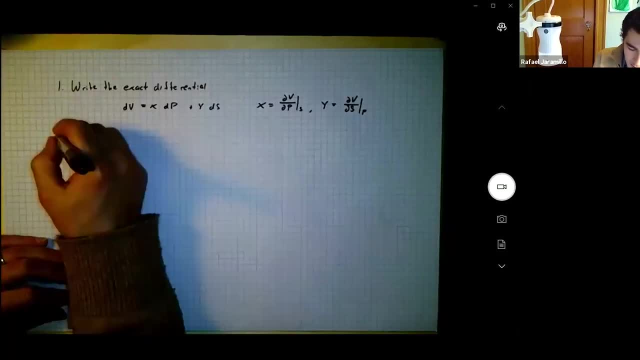 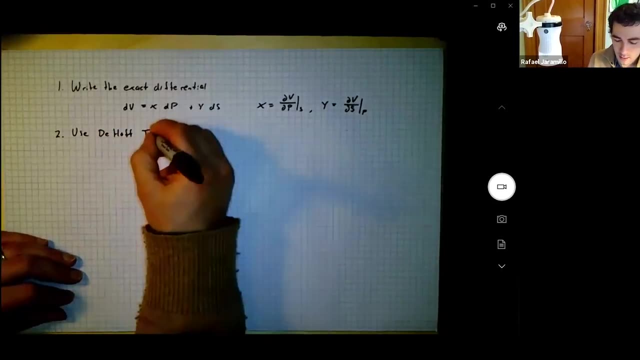 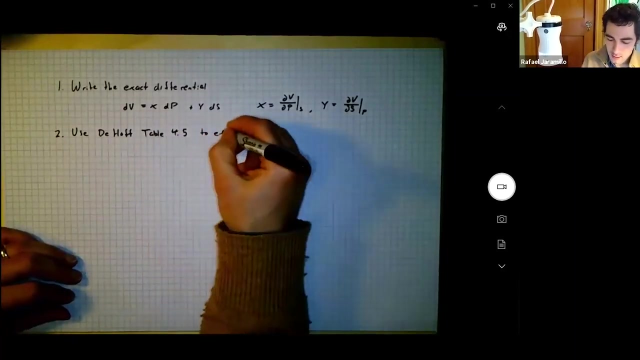 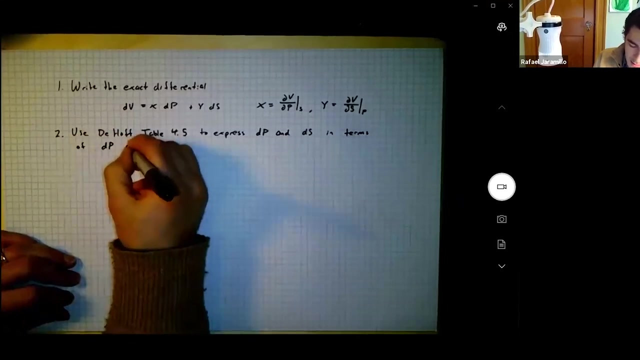 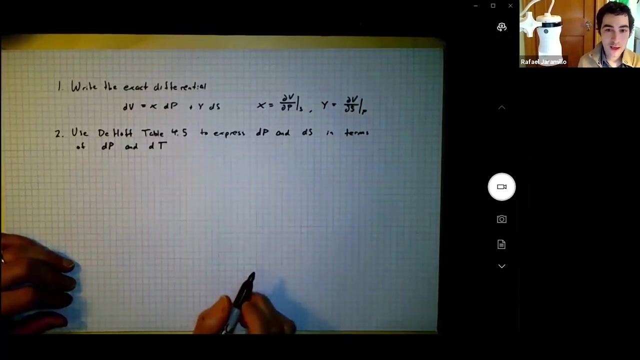 Then We're going to do a change of variables. There's a really useful reference to Hof, Table 4.5 to express dp and ds in terms of dp and dt To. Hof chooses p and t because it's a material science text. I know the text might have chosen a different two. 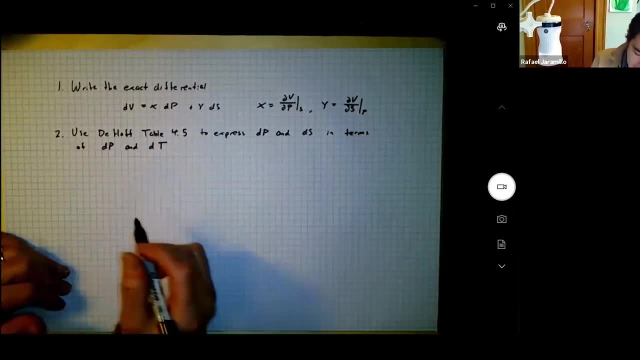 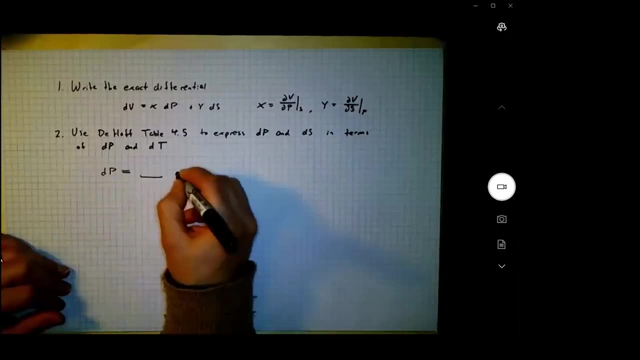 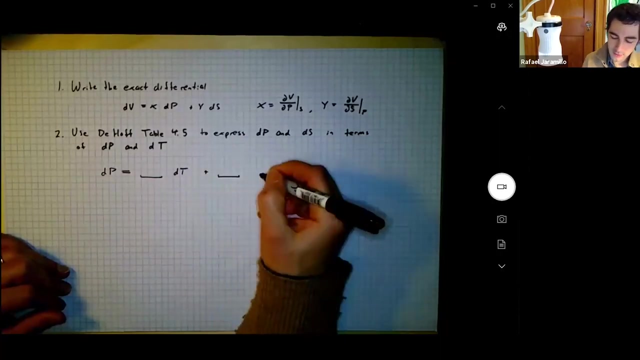 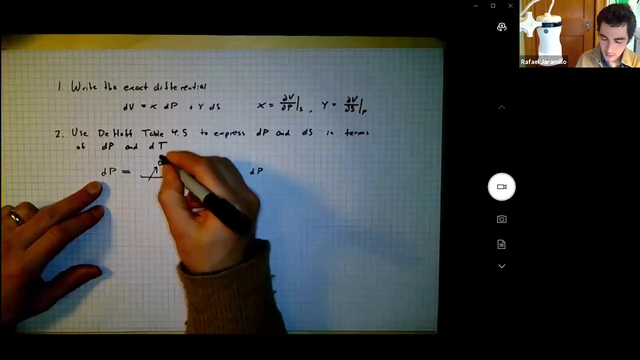 You can choose any two. So we're going to look up in Table 4.5, and it has the coefficients for every state, variable as a function of dp and dt. So here, this is trivial, right. There's going to be no, this is zero because dp equals dp. 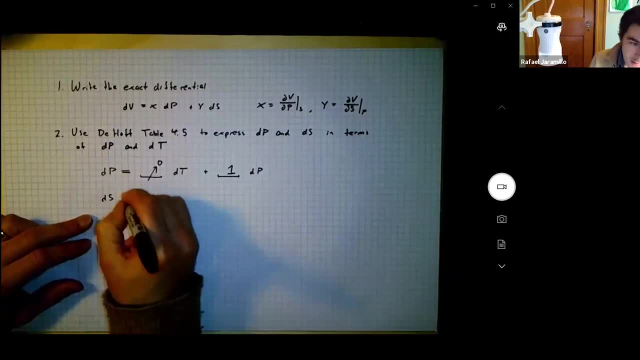 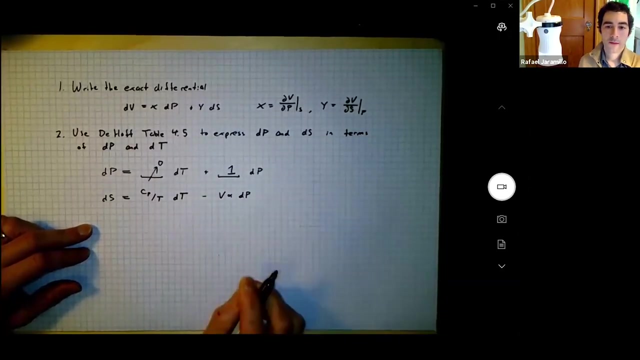 That's trivial. The entropy is non-trivial. We could derive this, but we're not going to take the time, We're just going to copy it from the table. It happens to be equal to cp over temperature times, dt minus v, alpha dp. 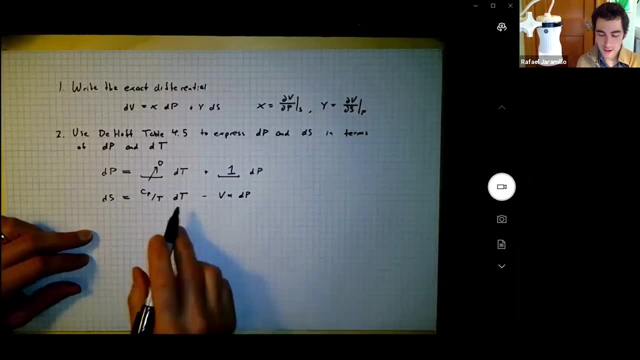 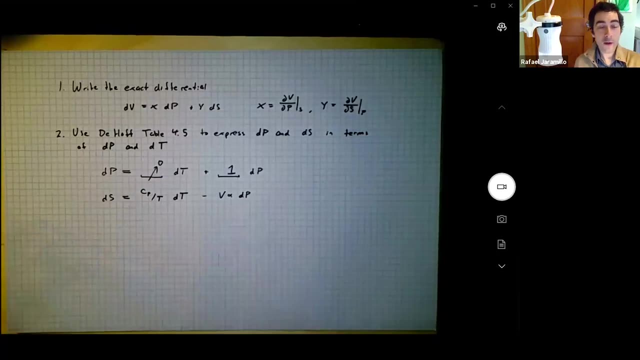 That's not obvious to me. I have to think about it. This I could figure out if I thought about it long enough. This doesn't make sense to me. I just have to derive it. But you don't have to derive it or think about it. 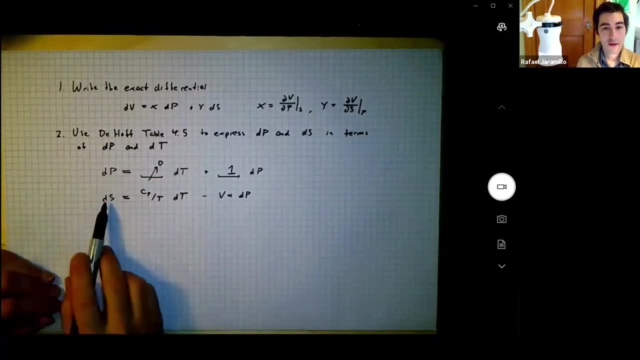 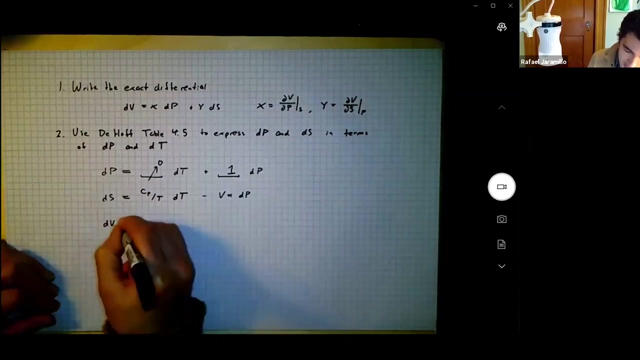 It's right there in the table. So here is pressure and entropy written now as dependent variables, dependent on temperature and pressure. Okay, so we're going to combine now and we get the following: dv equals x. I'm going to combine. 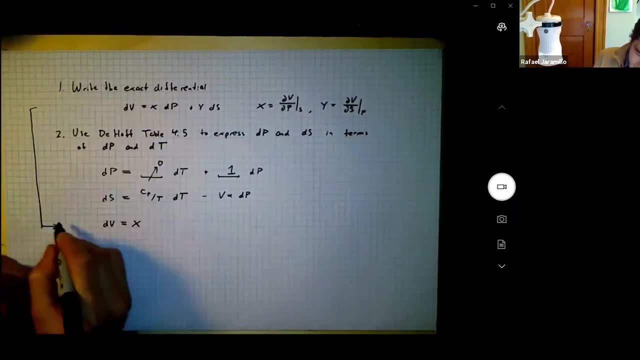 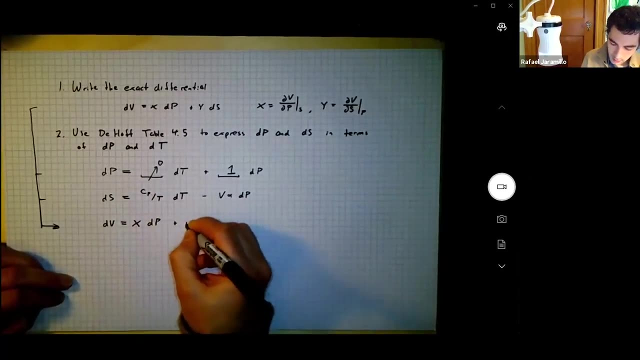 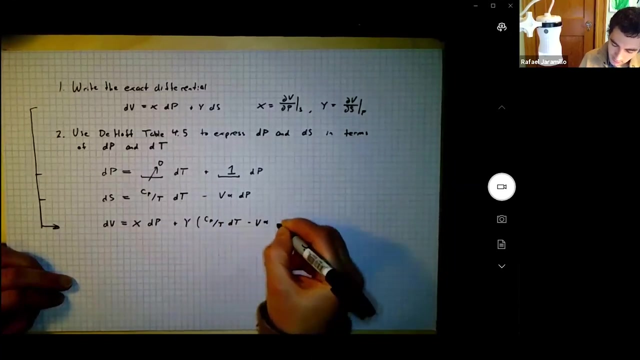 Okay, dv equals xdp- right, that's easy. plus y: What's ds? ds equals cp over t, dt minus v, alpha dp. I just plugged in substituted. substituted for ds here. Okay, so that's the second step. 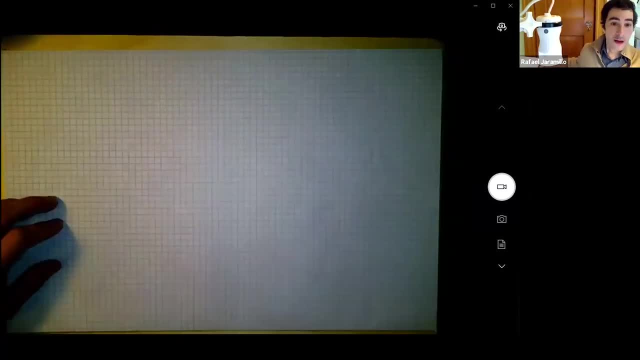 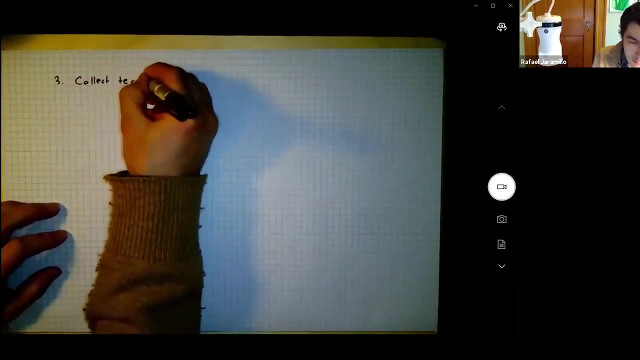 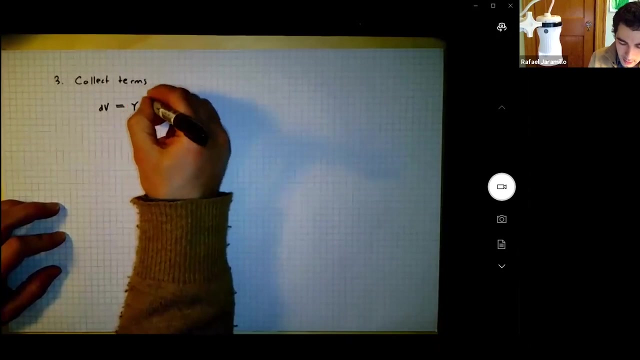 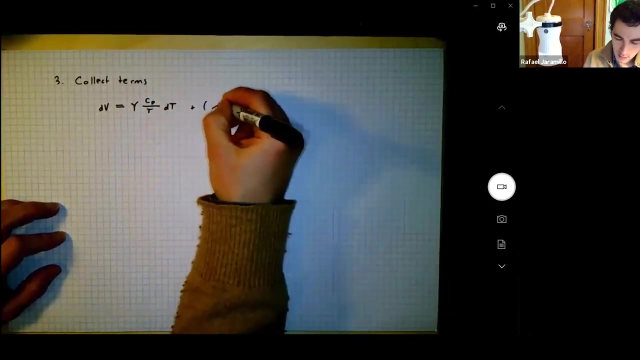 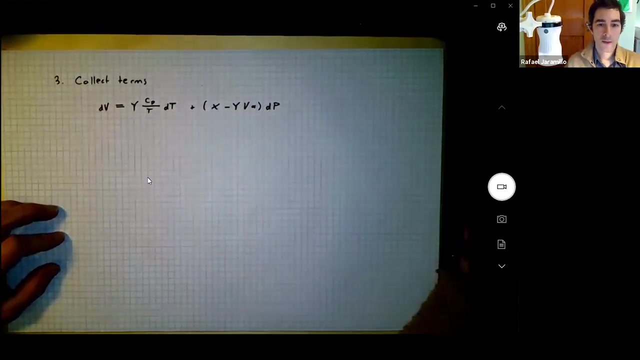 Then I'm going to collect terms. The third step is to collect terms. Collect terms. So I have the following: I have dv equals ycp over temperature dt plus x minus yv alpha dp. Okay, All right. All right, So I have dv equals ycp over temperature dt plus ycp over temperature dp. 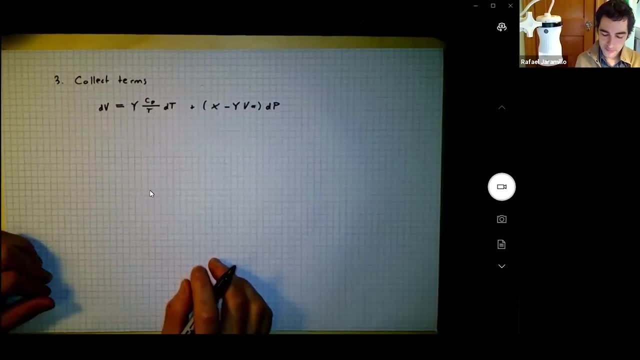 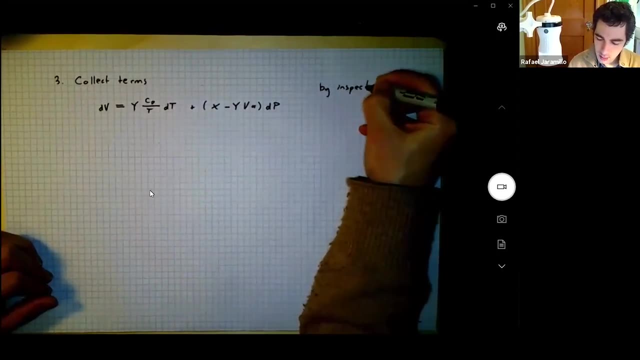 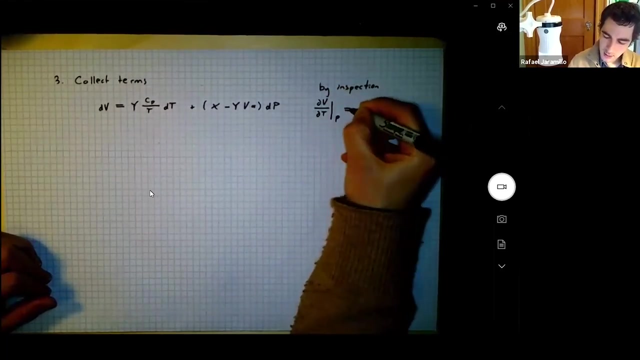 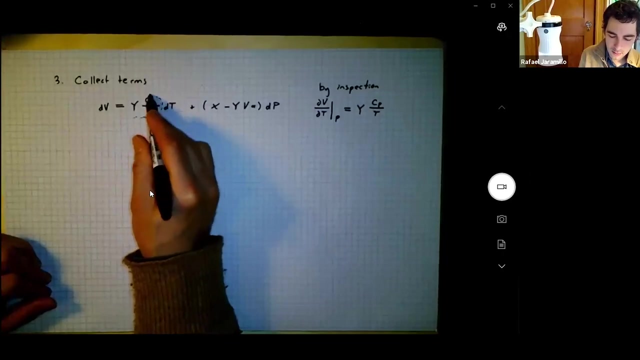 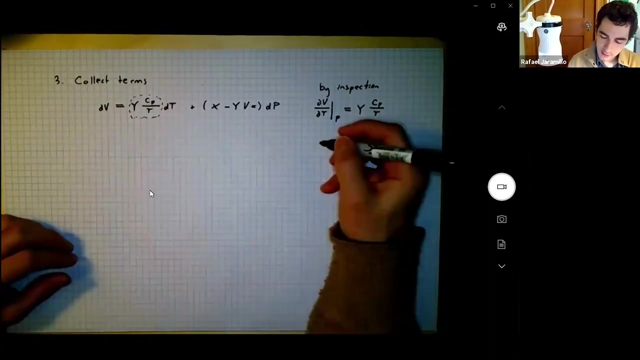 Okay, I still don't have x and y, I still don't know what they are, But I can say by inspection: dv dt at fixed pressure equals ycp over t. right, That's this coefficient? Okay, dv by temperature at fixed pressure- is that coefficient? and dv dp at fixed temperature. 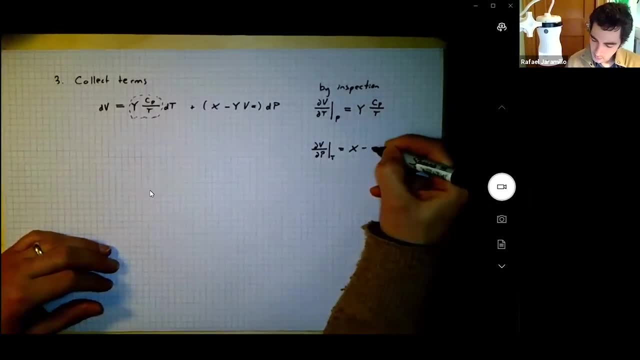 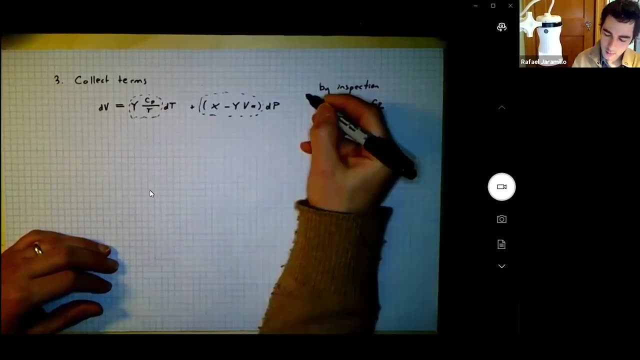 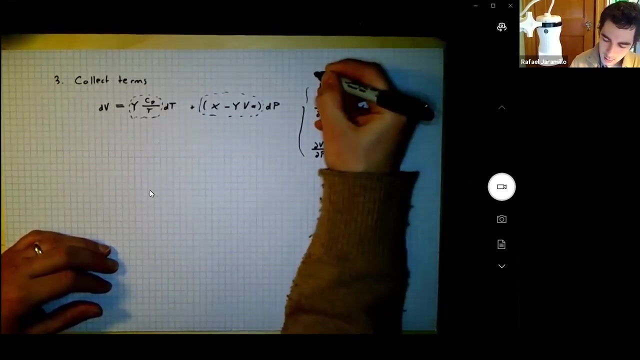 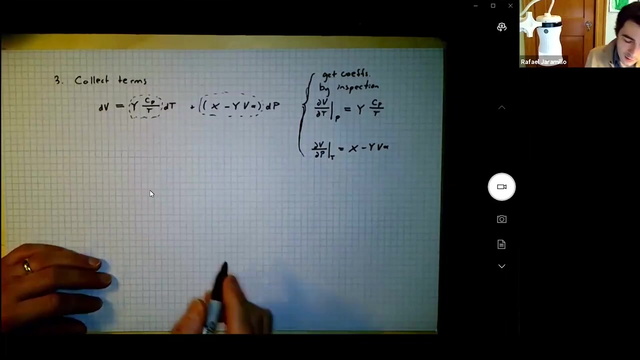 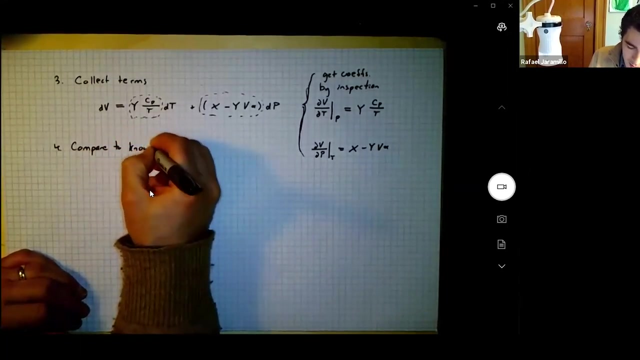 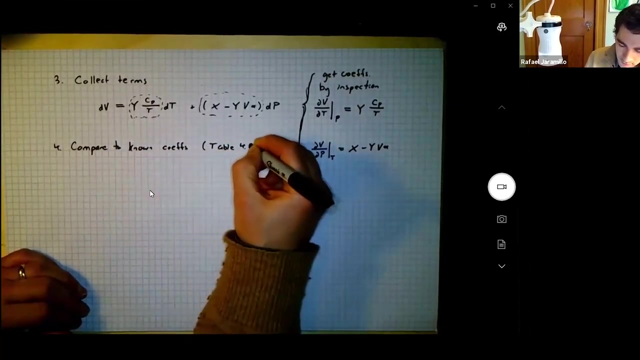 equals this coefficient x minus y, v, alpha. i say get, we get the coefficients by inspection. the fourth step is you compare to the known coefficients. so again referring to table 4.5. so in table 4.5 you will find the differential form of volume written as a function of temperature. 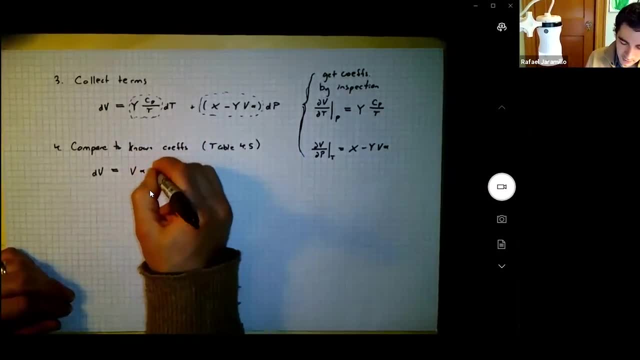 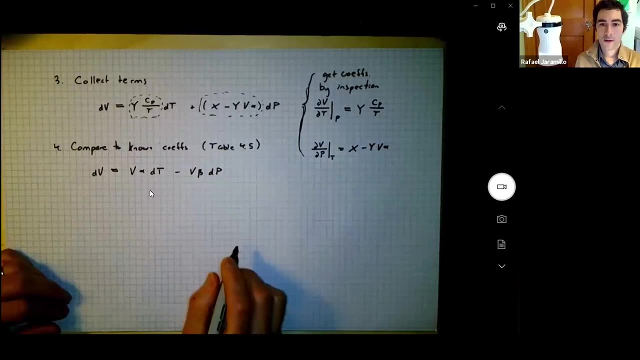 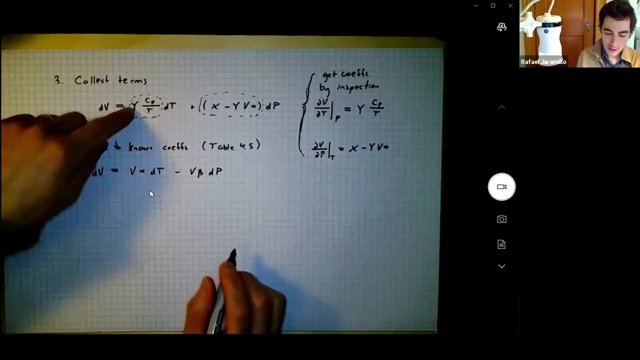 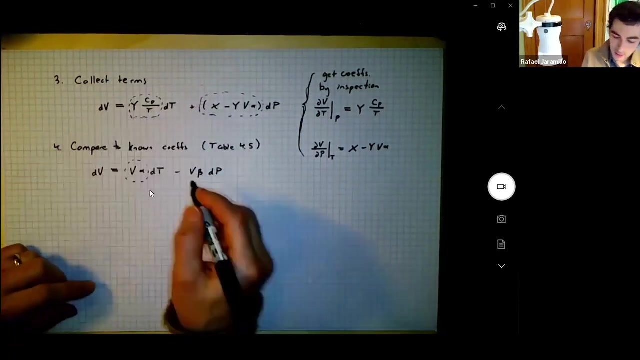 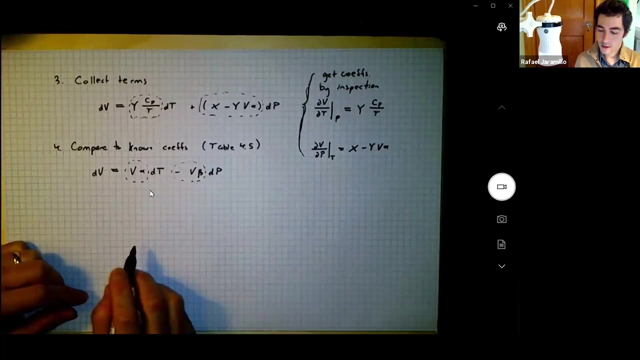 and pressure, and this is what you'll find: v alpha dt minus v beta dp. so here's the thing: this coefficient and this thing have to be equal, and this thing and this thing have to be equal because they're both the same mathematical objects. they're these partials. 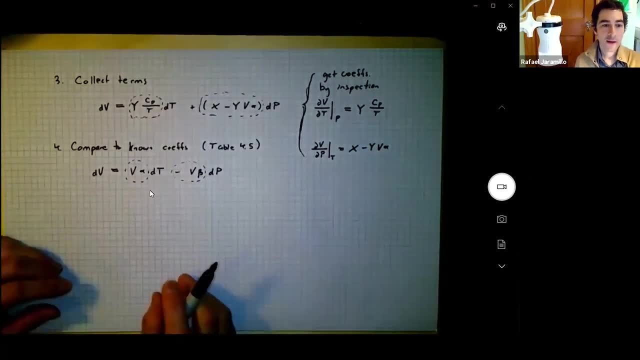 you can say it Talks like a Duck. talks like a duck. it's the same thing. so compare to known coefficients and equate. so we're going to equate and we're going to get the following dv dt at fixed pressure. well, that was this. right equals y cp over t, but it's also this: 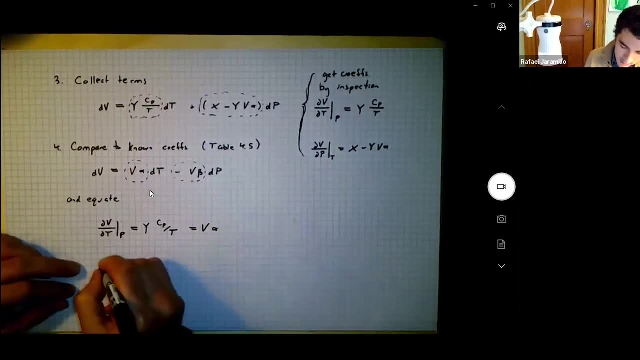 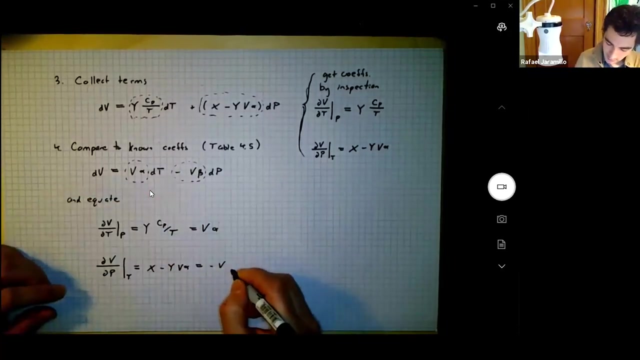 equals v alpha and dv dp at fixed temperature equals this x minus y v alpha. but it's also this equals minus v beta. so now we have our answer, how we have a system of two equations and two unknowns: x and y, two equations and two unknowns. 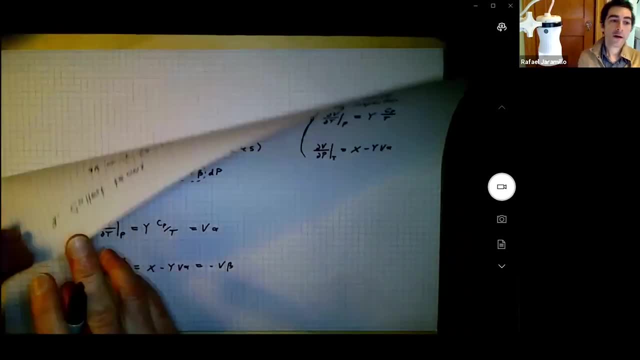 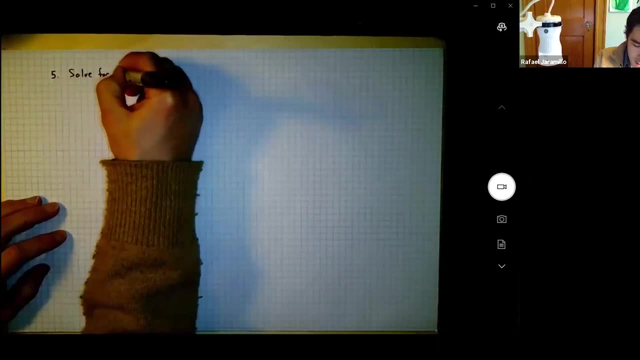 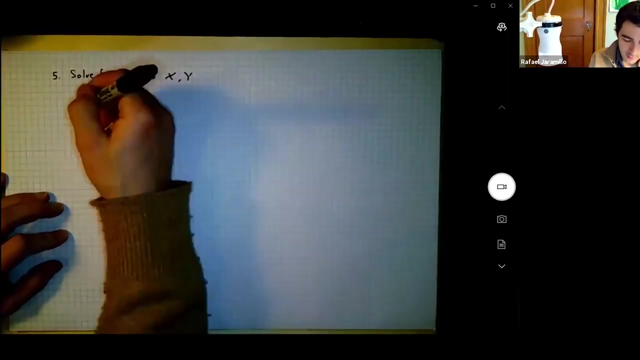 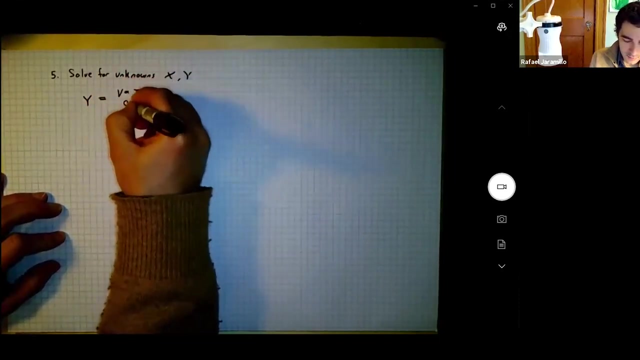 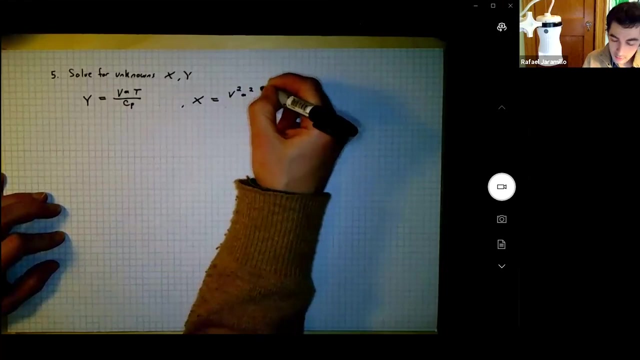 so now you can solve five, solve for unknowns. five solve for unknowns, and i'll spare you the the algebra there because it's pretty easy. solving for y, v, alpha, t over cp and solving for x equals v squared alpha, squared t over cp minus v beta. 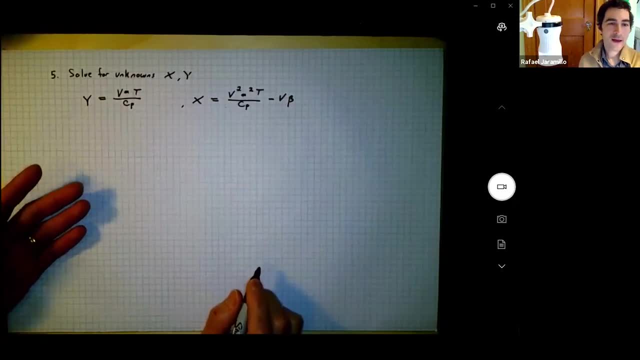 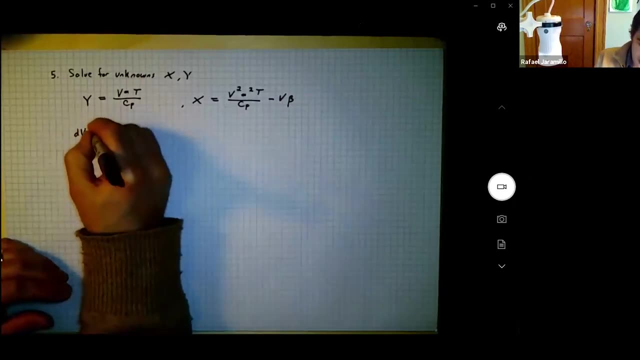 and these are complicated and are non-obvious, right, that's why you need a tactic, set of tactics- to get to these answers, because if you follow this approach, you will always get the right answer, even if it doesn't make sense to you. so here's the final answer: dv equals v squared, alpha squared. 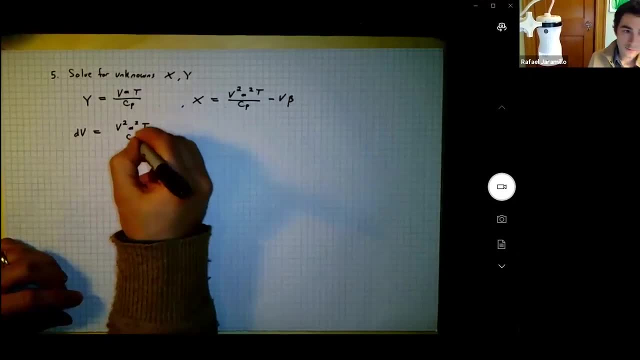 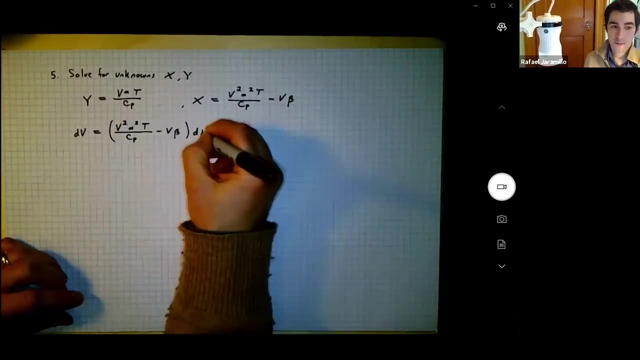 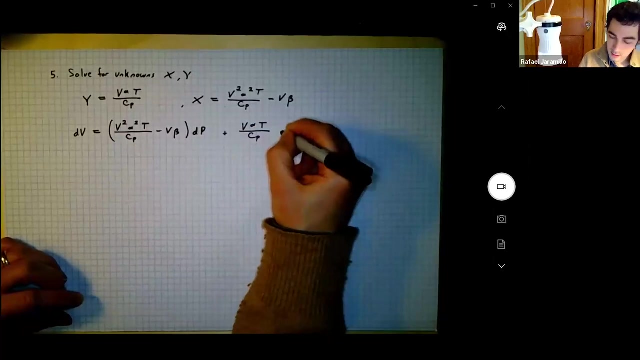 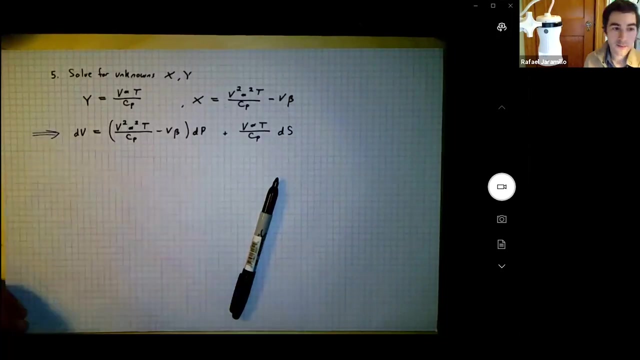 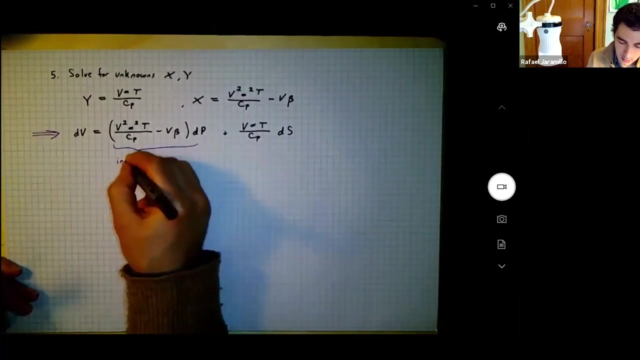 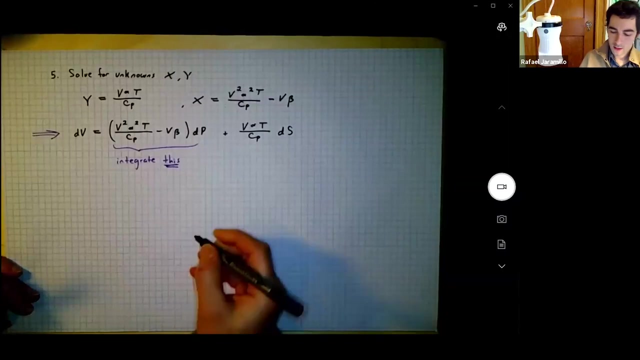 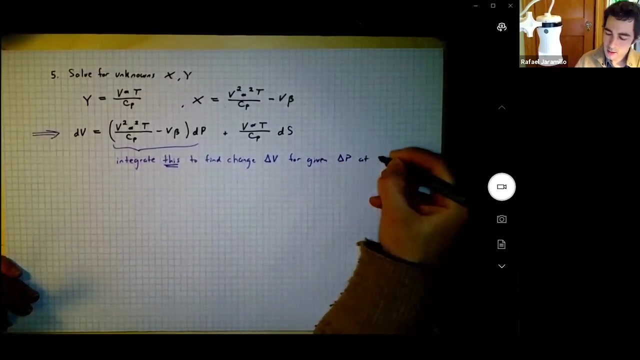 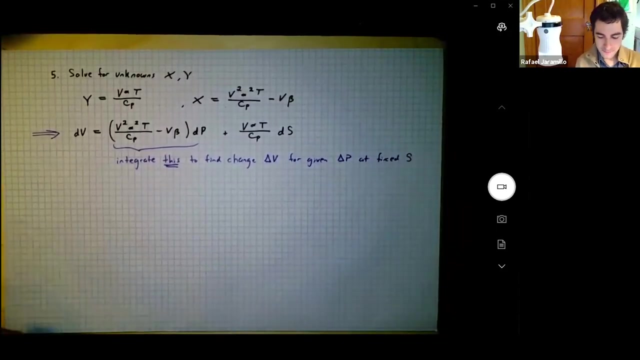 t over cp, minus v beta times, dp plus v alpha t over cp times d s. this is the thing we were looking for. that's it. we integrate this to find change delta v for given delta p at fixed entropy. again, this is mechanics right. this will work for you, even if if you don't. 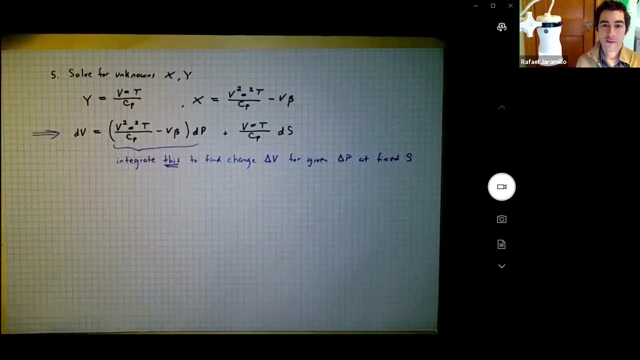 have a physical intuition for every step. this strategy works. question for a real material when you are okay, this is. this is very realistic. i mean, now we go from sort of multi-variable calculus to money on the line. right, you are calculating the effect of a pressure change on the volume of components. let's say you're going to send this into outer. 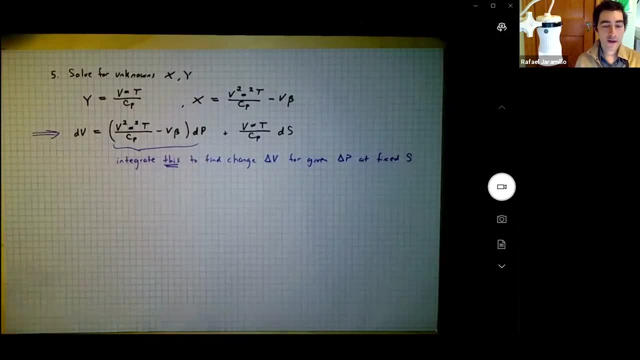 space and you have a system made out of components and the components are made out of materials and you want to make sure that the pressure change that your device experience isn't going to cause the thing to fall apart. so now this matters a lot. you need to know how to do that calculation. here's how question: where are you going to get these? this? 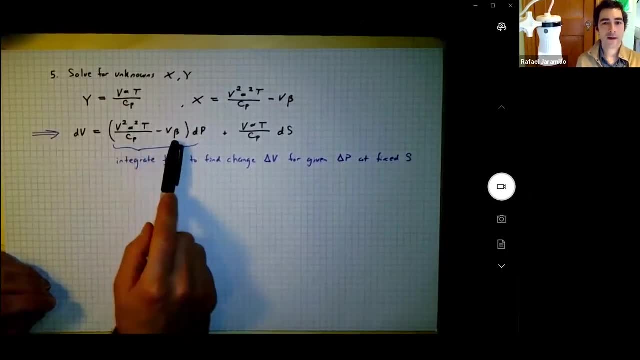 this is the integrand, right? how are you going to evaluate the integrand? how are you probably going to end up evaluating the integrand when you're working at spacex and you need the answer in five minutes? okay, let me set up a straw man. are you going to do density functional theory calculations to calculate? 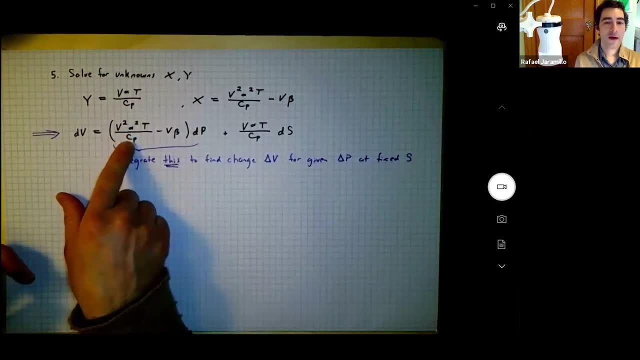 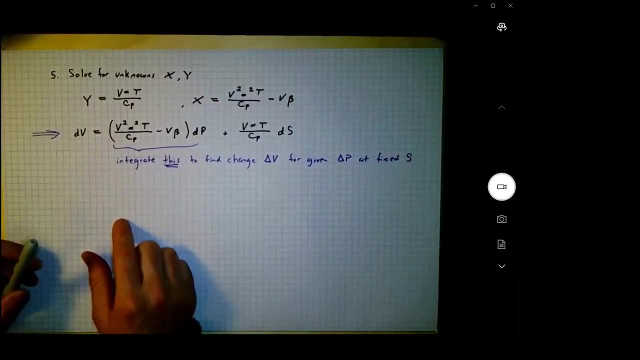 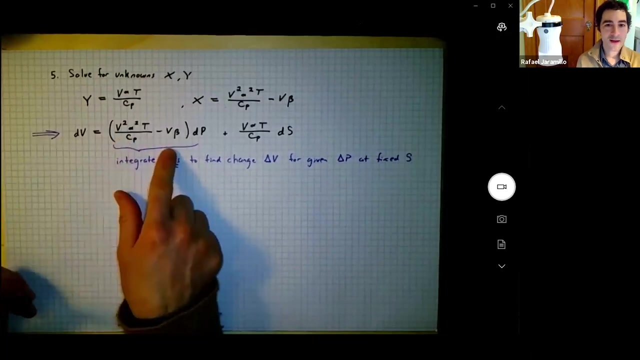 the thermal expansion coefficient and specific heat and volume and compressibility for your material. from first principles, you're going to probably look at databases. databases, thanks, that's like my favorite word. do you look at databases? this stuff is in databases. you're going to parameterize what you need. 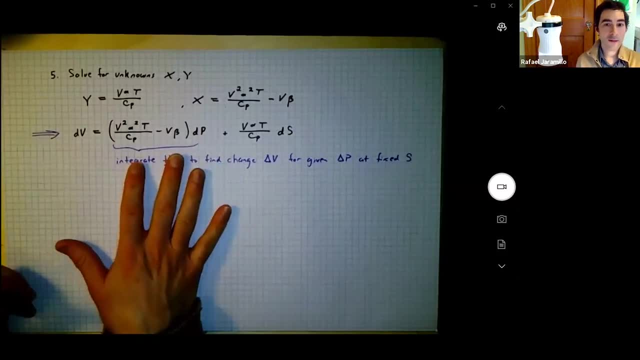 using databases. you're going to plug that in and you're going to do this integral, numerically. the computer is going to do it for you, right? you're going to make sure you have good sources of data. you're going to make sure the data is inputted correctly. you're going to make sure. 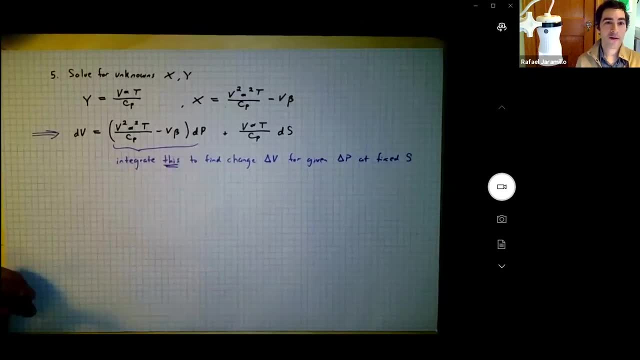 your units are right and then the computer is going to do this for you as a numerical integration. that's how it works in the real world. so so this is this sort of hairy looking challenge is why we hammer on this stuff in oto and we make you talk to you know, you get to meet the librarians and such, because being able to go 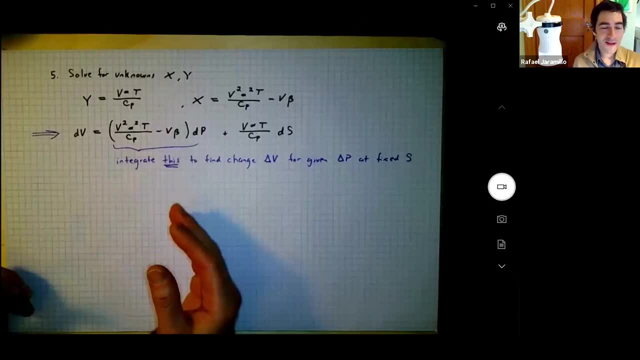 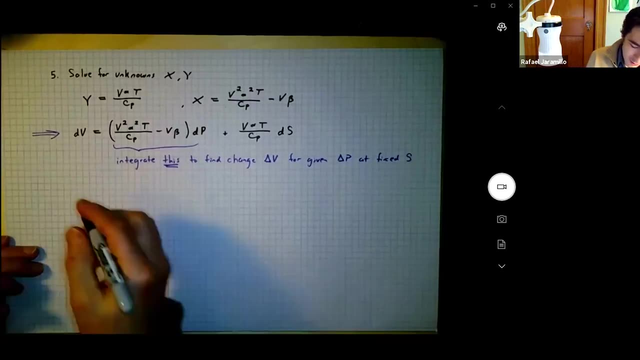 from those data resources to answers right is really an important skill. it's really an important skill. all right, there is one case where you don't need to do any of that and we'll discuss this a little more next lecture and you can work this out- uh, you know, on your own, for if you're curious, 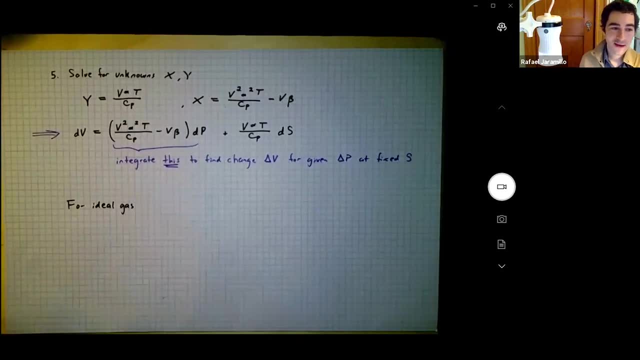 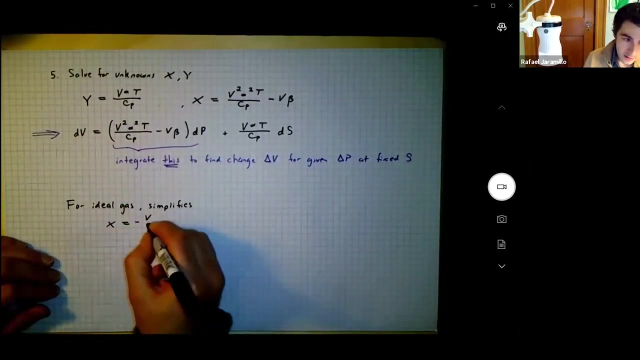 it's also worked out plenty in the textbook for an ideal gas, as with many things, it simplifies so you don't need any databases to evaluate this for an ideal gas. it simplifies to the following: x equals minus v over p times c, p minus r over c. p is also equal to v over p, c v over c p. 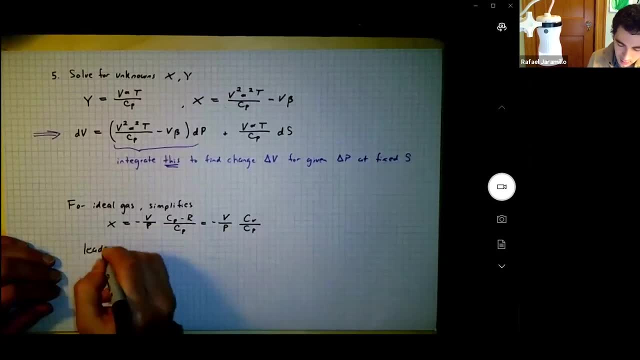 and this leads to an expression which, before we get to this, just gave you: P final over P initial equals V initial over V final. This is where that comes from. I've used this expression for adiabatic process, for an ideal gas. It comes. 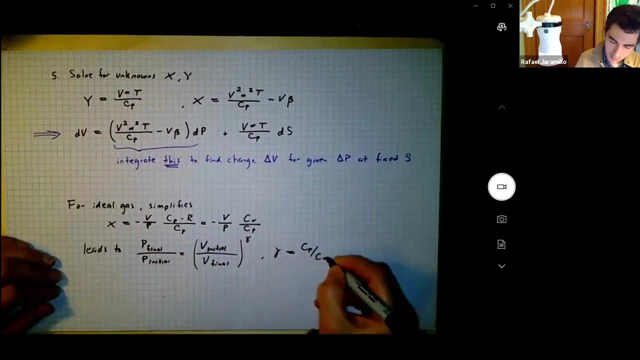 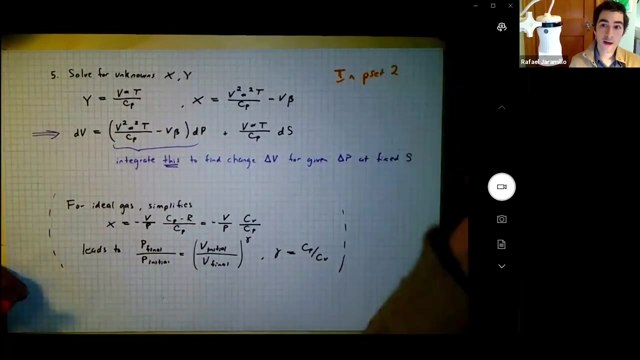 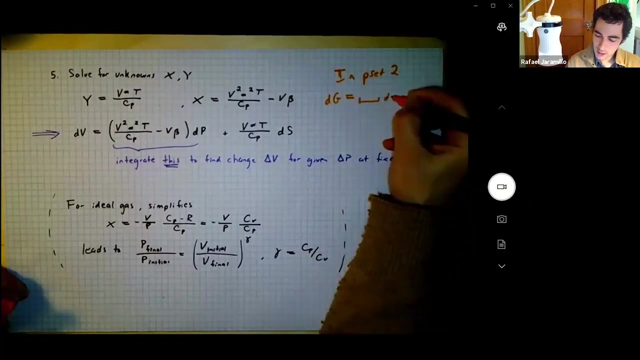 from this I'm not going to take time to derive that now. It's an interesting calculation. You can just evaluate all this stuff. I'll just mention that in Pset 2, you're doing a related problem, which is you're calculating change in Gibbs, free energy with pressure. 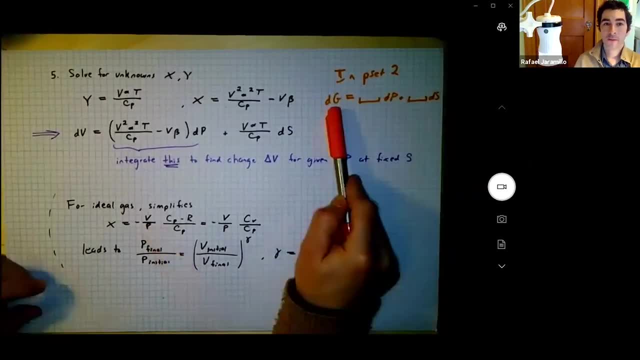 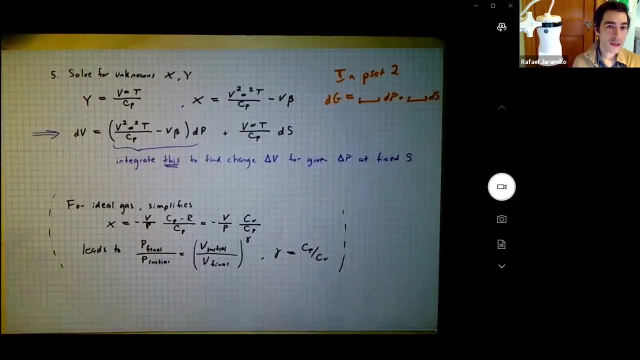 and entropy. We just did volume with pressure and entropy In Pset 2, you're going to do Gibbs with pressure and entropy. The overall- what they call the general strategy- is that it's the same For the remaining minutes. we're going to get a little bit specific and 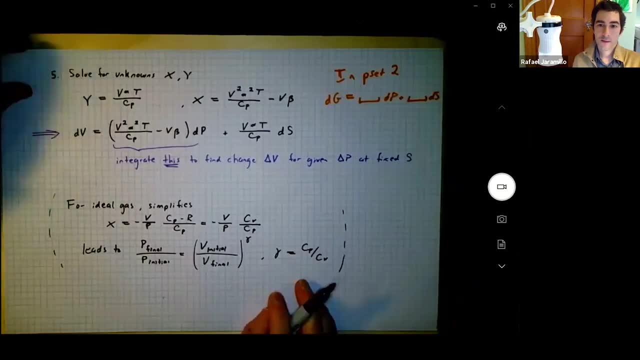 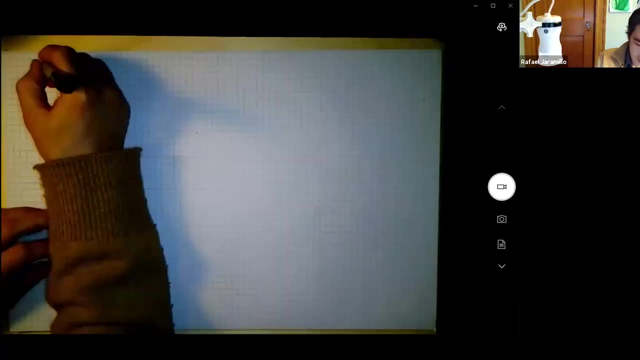 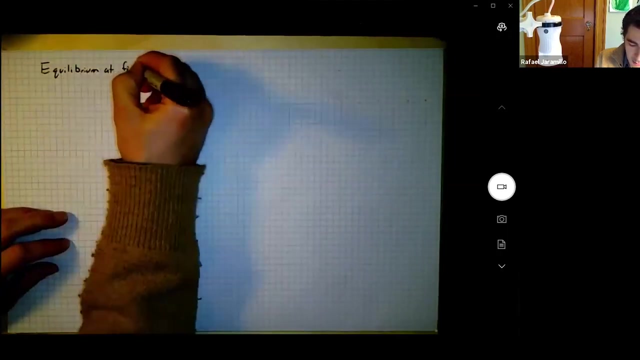 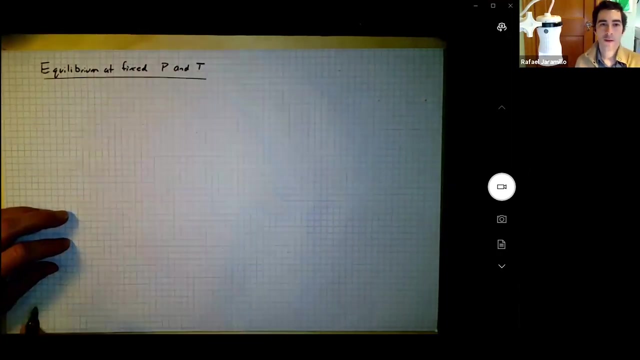 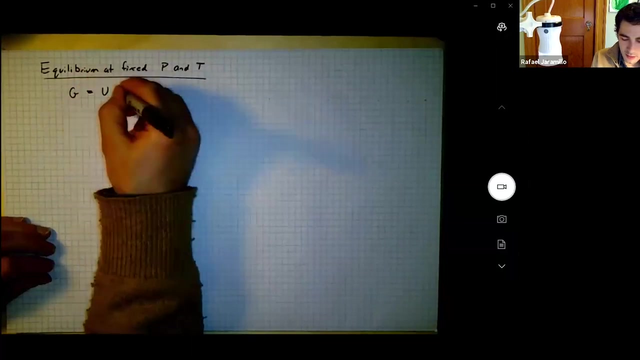 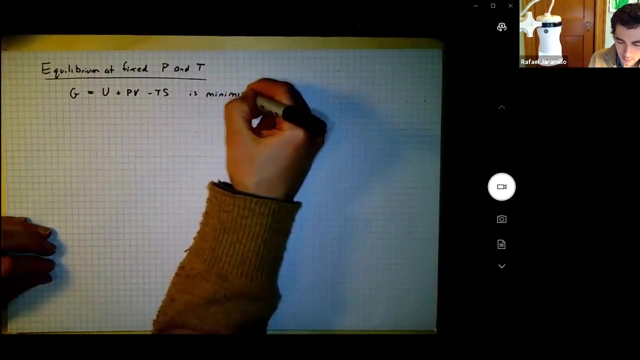 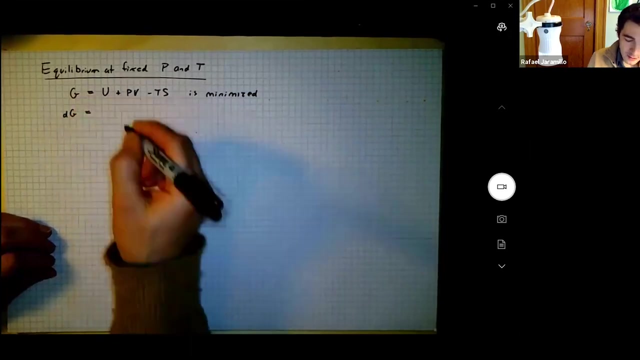 talk about Gibbs free energy. Let's talk about equilibrium, Fixed pressure and entropy. Now we're processing materials. Gibbs free energy equals U plus PV minus. TS is minimized. Let's play with the differential form DG. I'm going to use the chain rule. 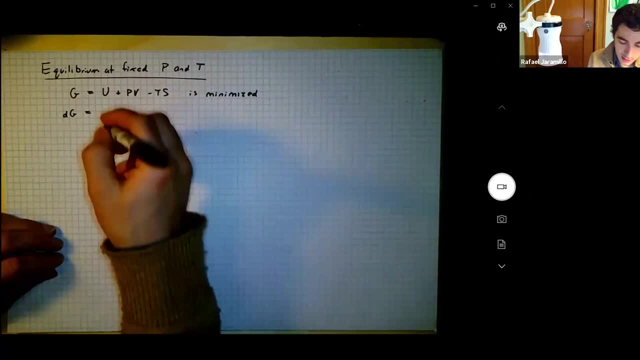 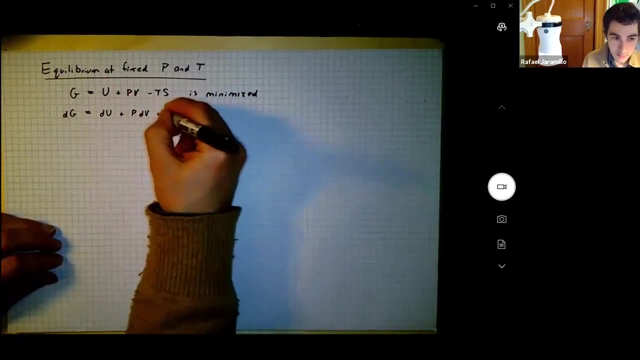 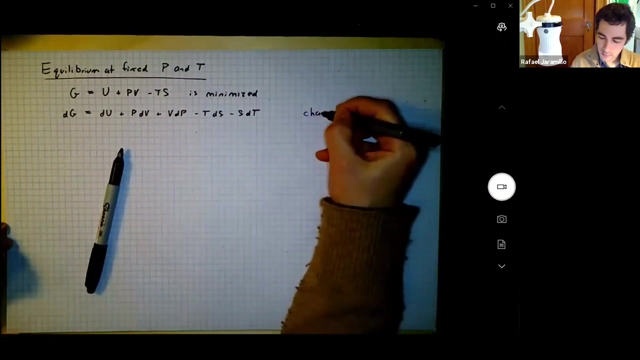 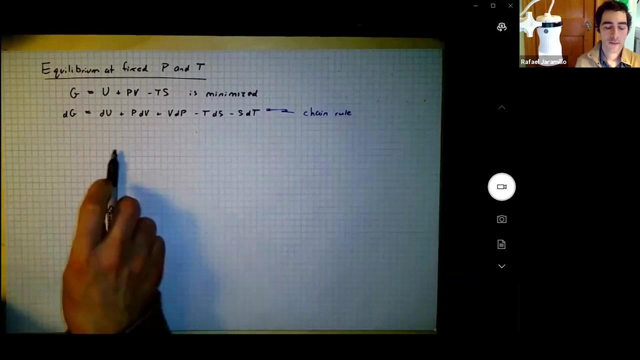 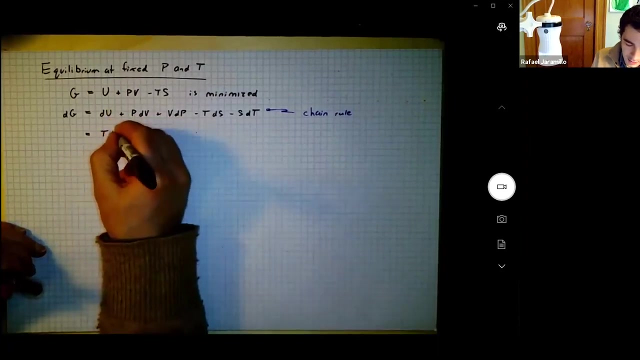 It's going to be DGS minus SDT, And that was just chain rule. Now I can use the combined statement: DU equals U, U equals U equals T, D, S minus P, D, V plus mu of I, D, N of I. 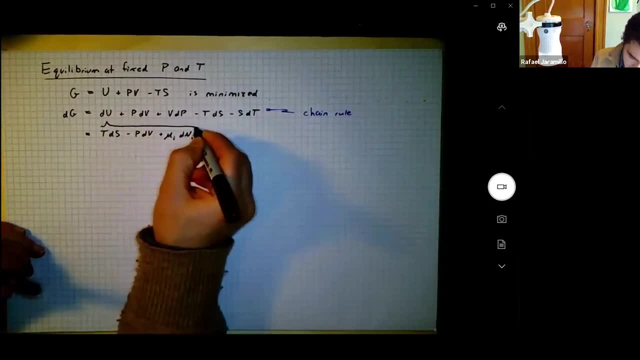 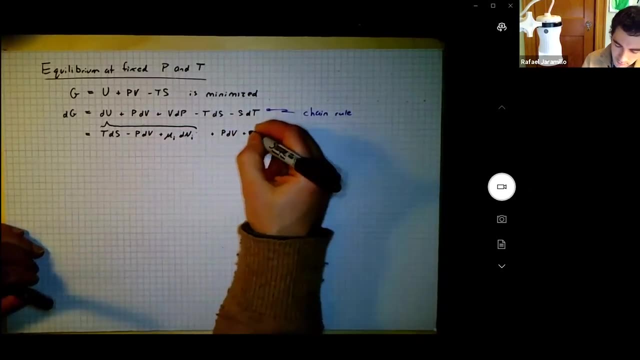 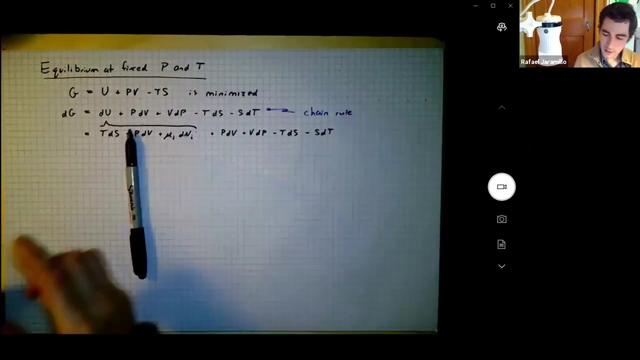 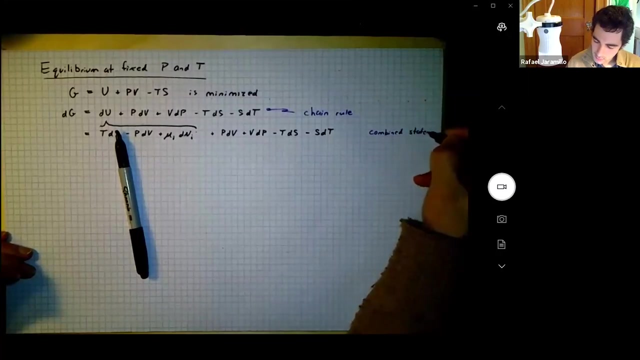 That is all D U. I carry the rest of the terms Plus P D V, plus V D P, minus T D S, minus S D T. So here I use combined statement And I'm going to see a bunch of things cancel right. 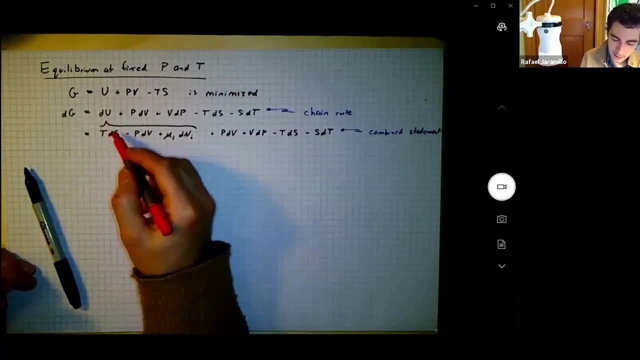 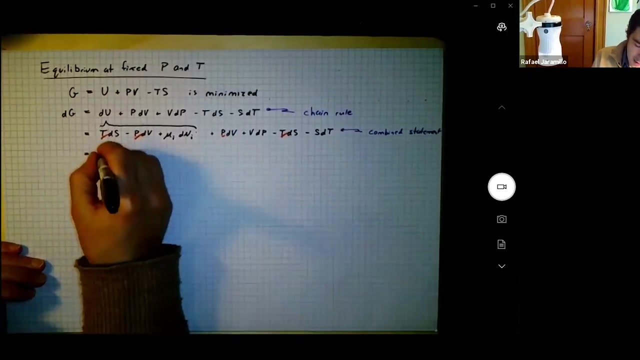 I'm going to see a bunch of things cancel. So we have T D S cancels T D S, minus P D V, cancels P D V, And so it simplifies a little bit and I get the following: equals minus S plus D T plus V D P plus mu I D N of I. 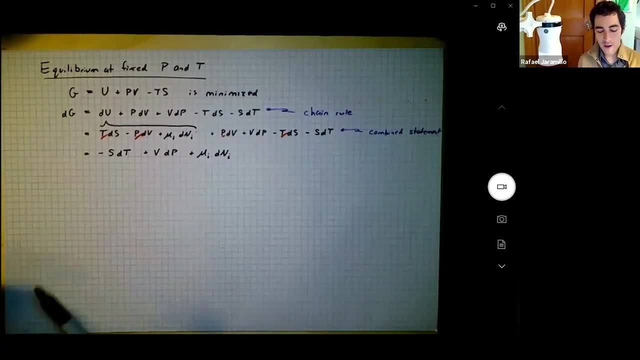 Good, This is what we wanted, Cause I told you the natural variables for Gibbs were temperature, pressure and particle number, And that's what we get, That's what the calculus gives us. So there's a little clue there into how the, the, the, the, 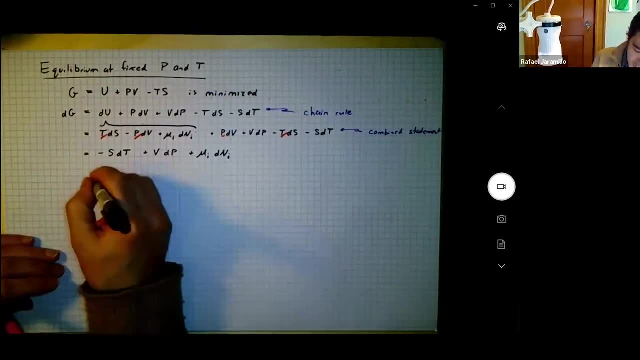 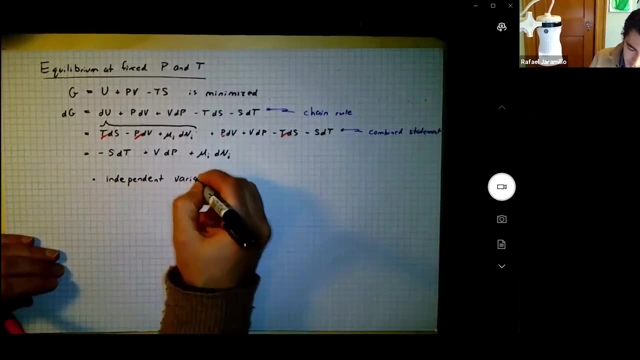 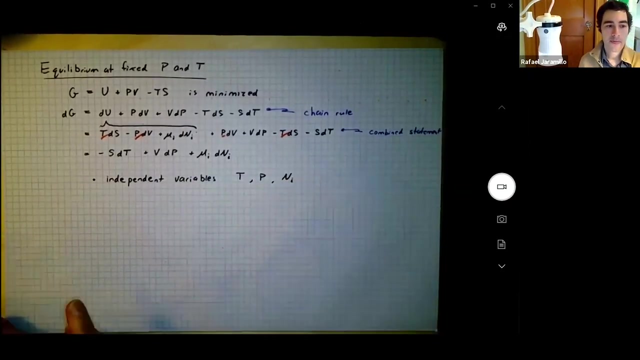 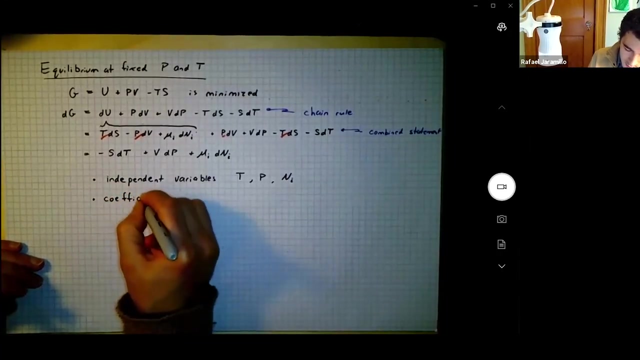 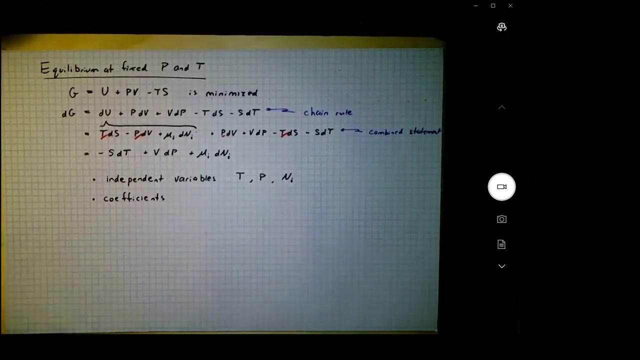 how to transform works. But again, we won't go there. So the independent variables are T, P and then somebody. And what are the coefficients? Somebody please? They're equal, Surely. that's V, V and mu of I, S, V and mu of I minus S, V and mu of I. 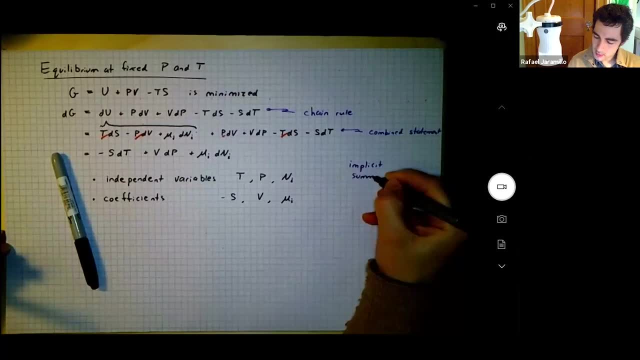 I'll make a note here. A lot of times in this class I used implicit summation, Correct. You probably picked up on that. But this implies i mu of i ni just a little bit more compact right. there's no i index on the left. 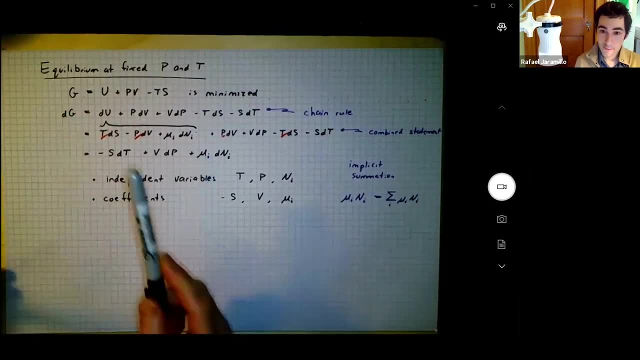 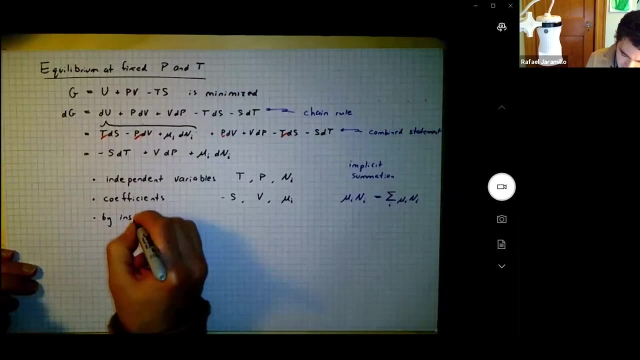 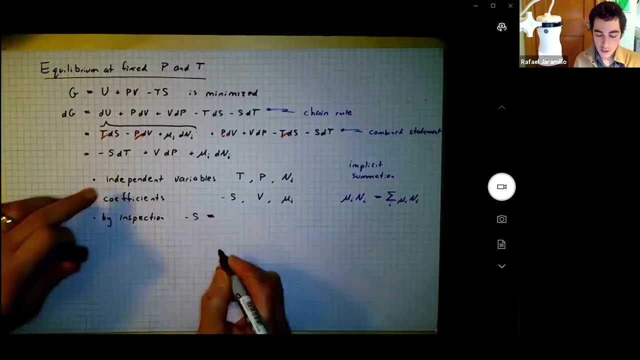 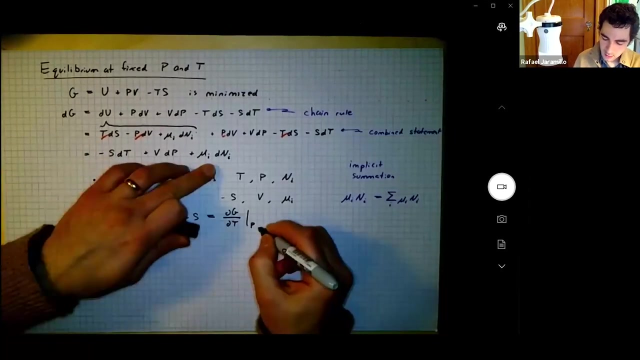 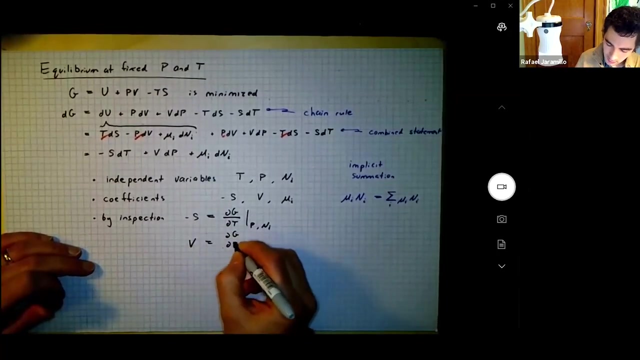 hand side, so that means it has to resolve on the right hand side, so you implicitly sound right. and by inspection. by inspection minus s describes the change of gibbs with temperature at fixed pressure and particle number. volume describes the change of gibbs with pressure at fixed temperature and particle number. 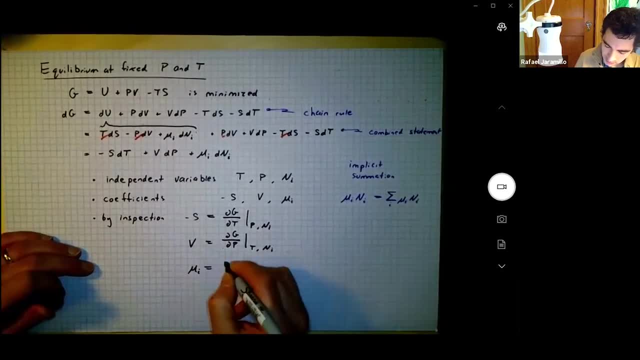 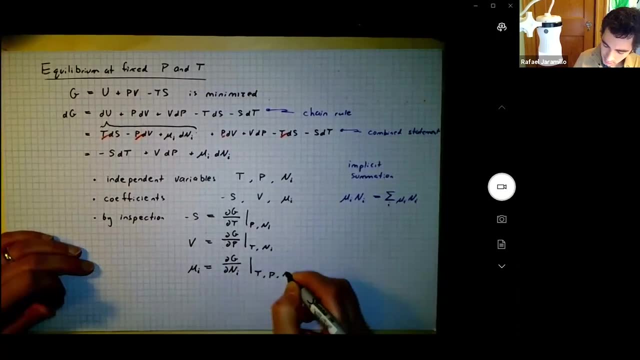 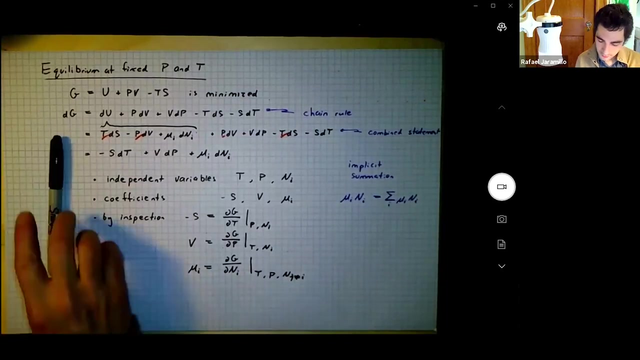 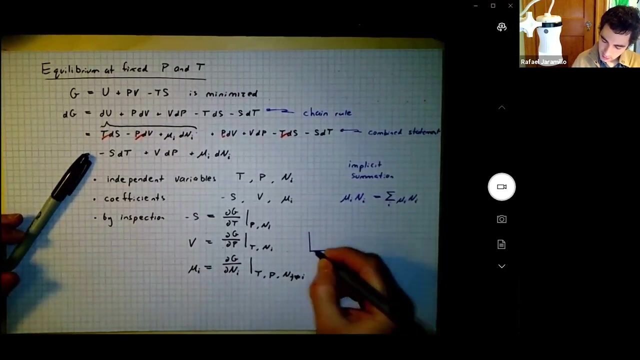 and finally, our favorite chemical potential describes the change of gibbs with particle number i at fixed temperature pressure, and particles j not i. so already we can say something about the slope of these things, on a slope of, let's see, here's pressure and here's gibbs, free energy, and we're fixing temperature and particle number. 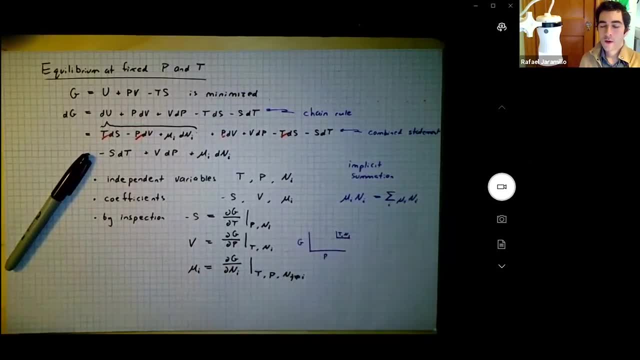 what's the slope? what's the slope? is it positive or negative? gibbs versus pressure for fixed temperature and particle number. what's the slope? is it positive or negative? gibbs versus pressure for fixed temperature and particle number? it's positive. positive because volume is always positive. can't have negative volume. 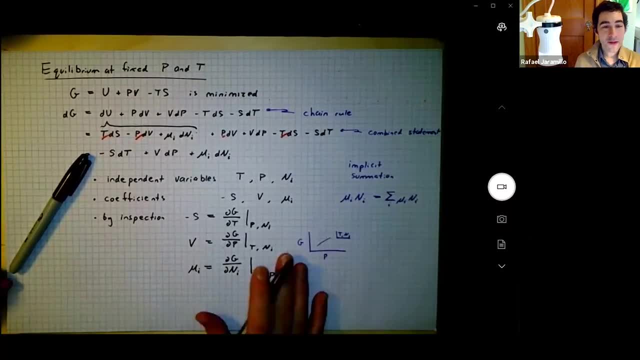 right. so that's good. being able to pick off the slope and the curvature of these things is really useful. It's really really useful, as you'll see. What about this? What about temperature Change of Gibbs with temperature for fixed pressure and particle number? 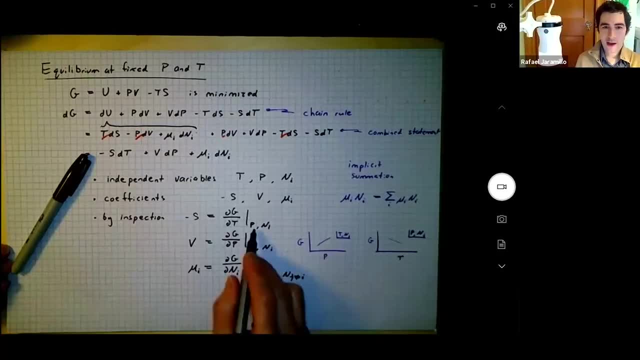 Negative. Yeah, it's negative Because entropy is strictly positive. So negative entropy is strictly negative. You gotta think about these slopes, The Gibbs. free energy increases when we squeeze. That's related to the enthalpy. That's related to the enthalpy. 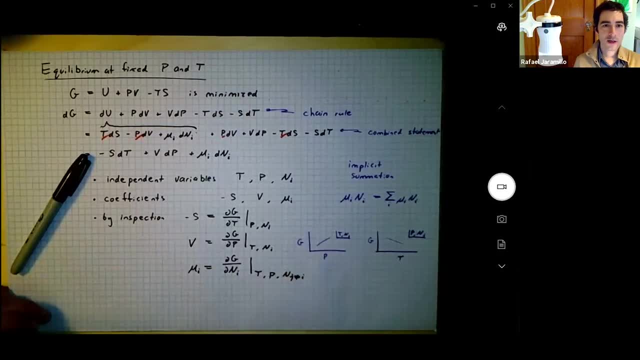 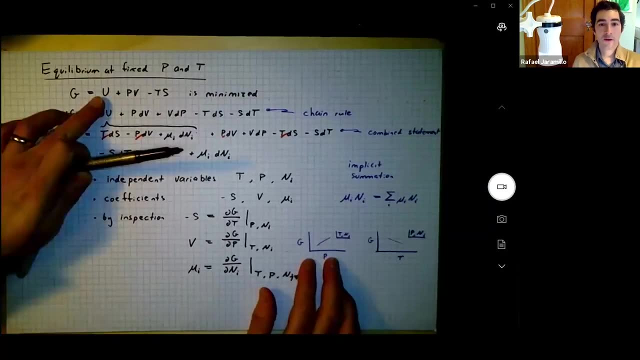 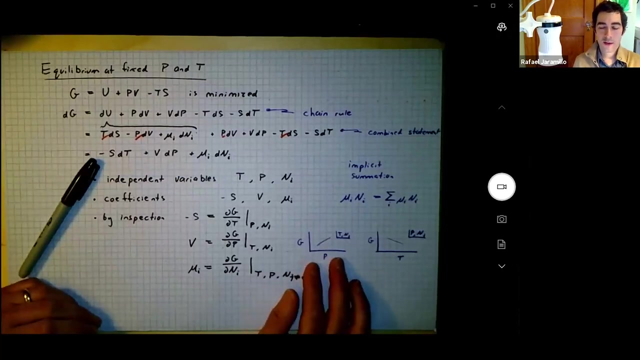 When we squeeze something, we're increasing the energy content of all the bonds that make up that thing. When we squeeze something, we're increasing the entropy content of all the bonds that make up that thing. So this is Gibbs: free energy getting higher as we squeeze. 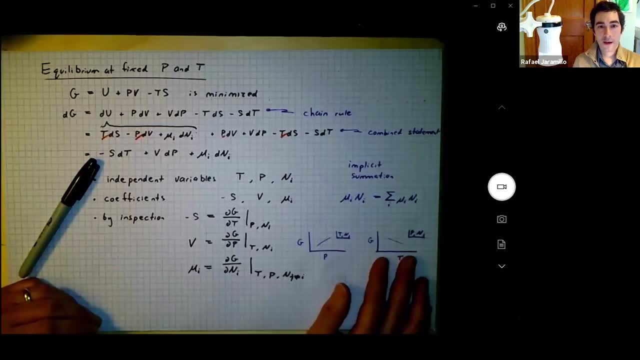 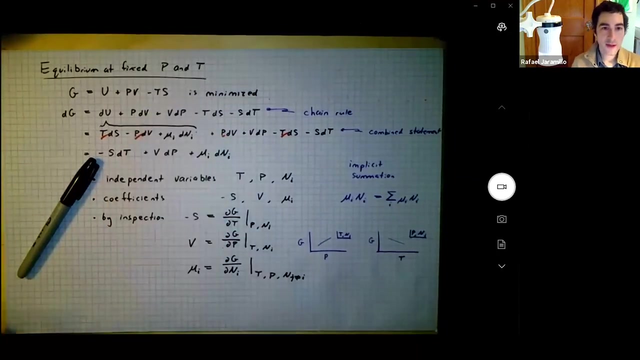 When we heat something, Gibbs decreases. When we heat something, we're increasing the entropy, We're increasing the amount of mixed up-ness And Gibbs depends negatively with entropy. We'll see this in many examples. Okay, So up with pressure, down with temperature. 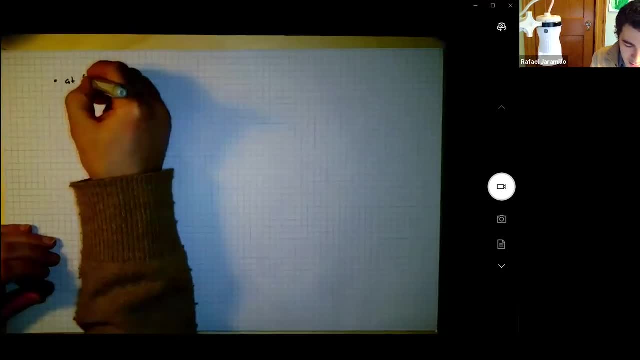 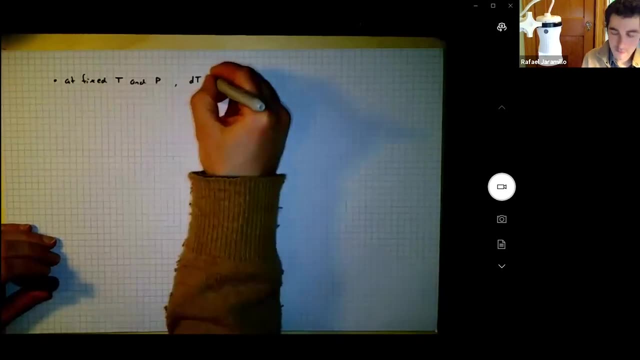 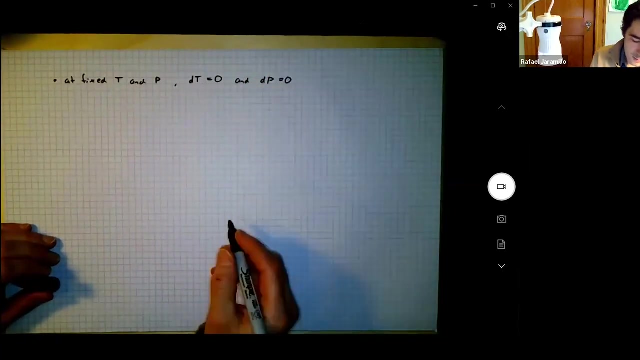 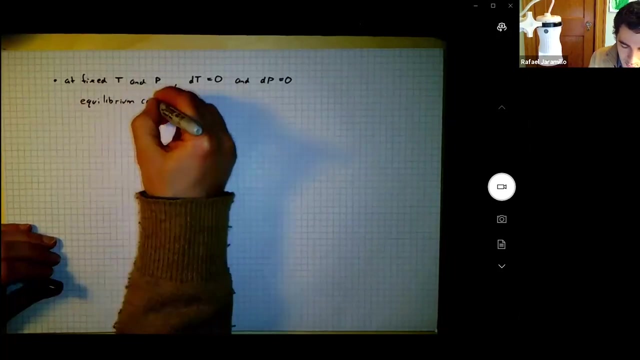 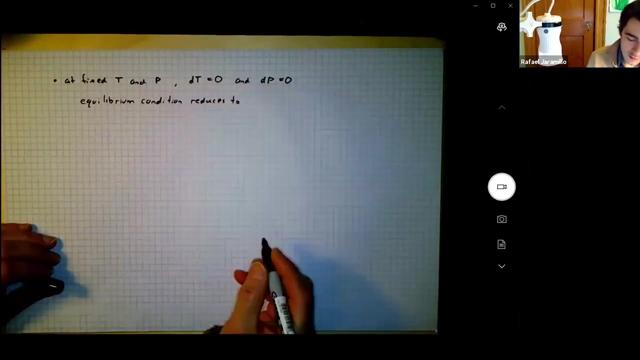 What about conditions that we're interested in? At fixed temperature, T, At fixed temperature and pressure, DT equals zero. That's pretty easy. And BP equals zero. That means the equilibrium, the equilibrium condition reduces to DG, equals zero. Let's see. 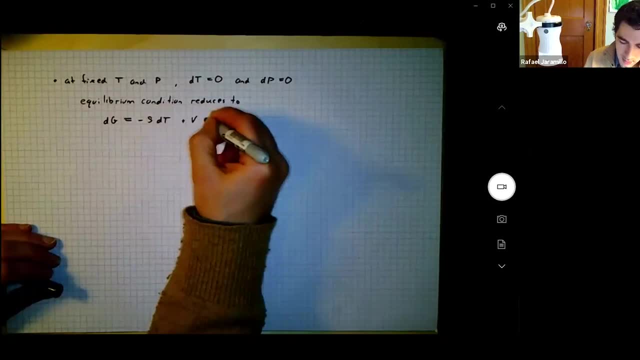 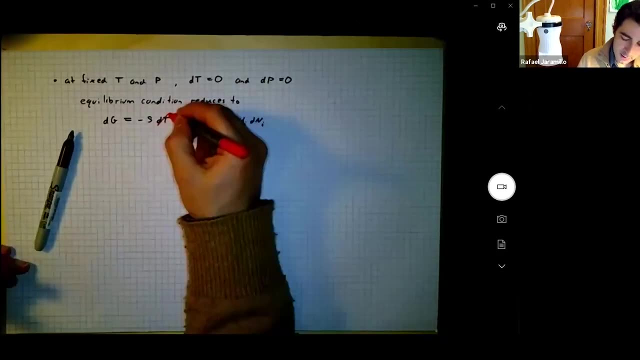 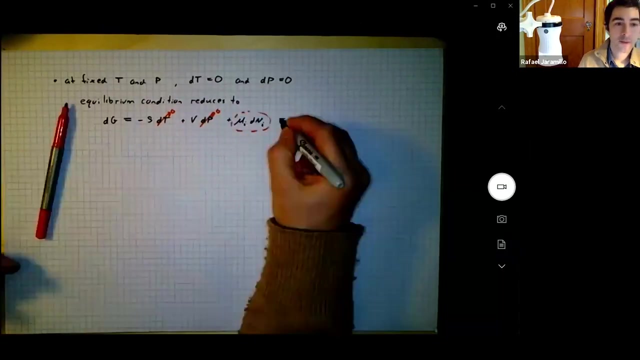 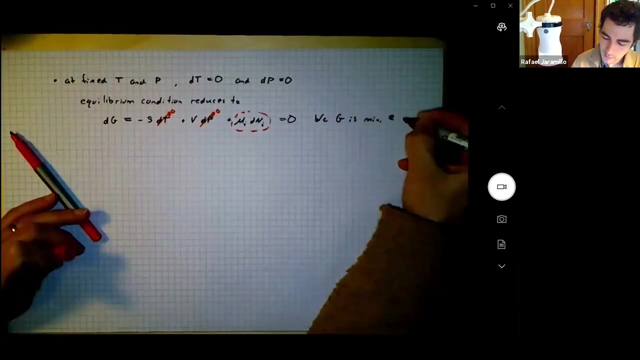 Minus SDT, plus VDP, plus mu, by T and of I, And we're holding that fixed. And we're holding that fixed. That means it basically reduces to this equals zero, Because G is min at equilibrium. So we think back to calculus. when you would calculate, 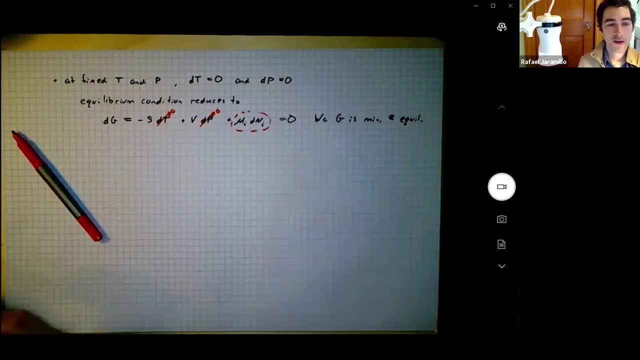 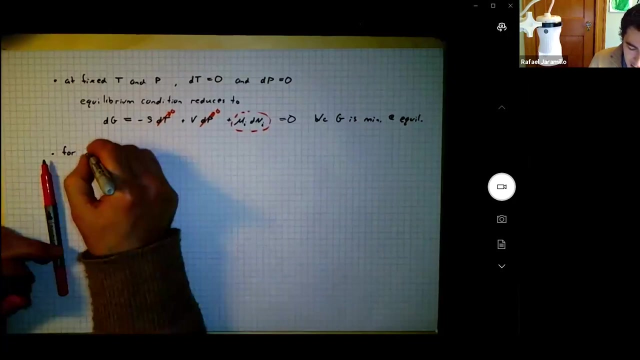 Calculate extrema right. The extrema positions of a function are where its slope is zero. So equilibrium condition is that the change of Gibbs with particle number i is zero. So for most of the cases of interest to us as practicing material scientists, that is multi-component. 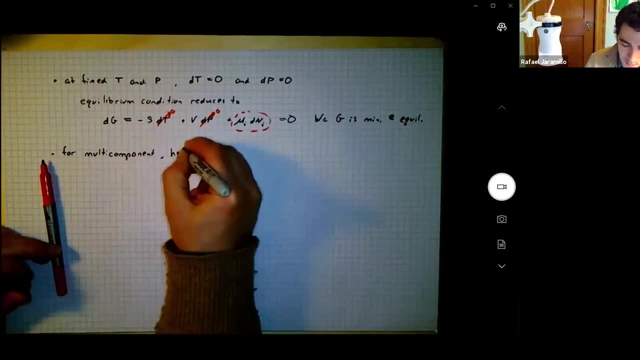 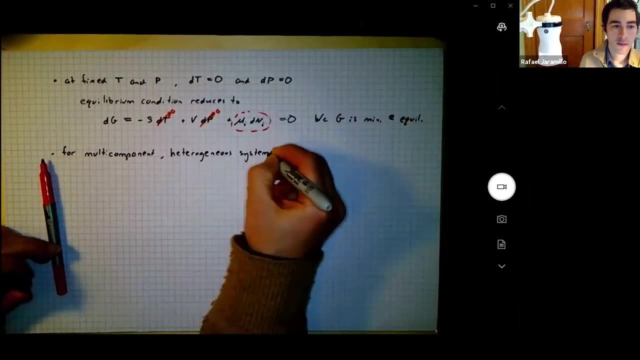 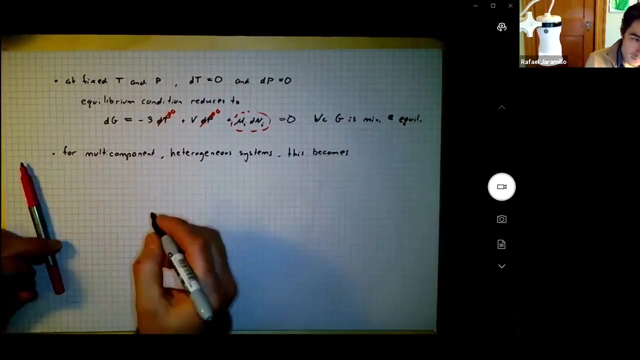 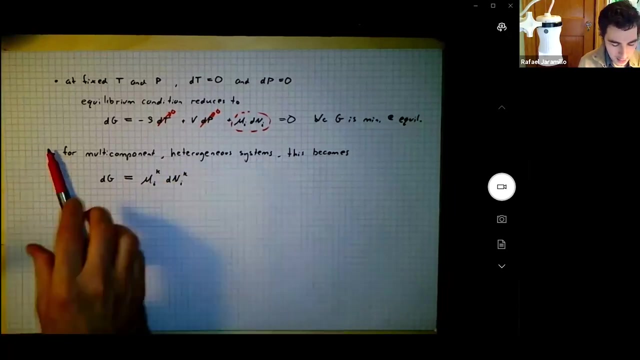 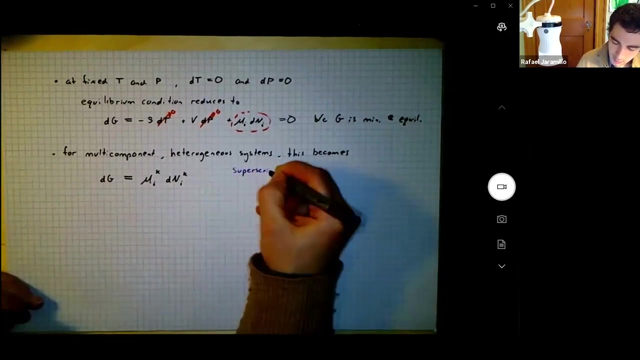 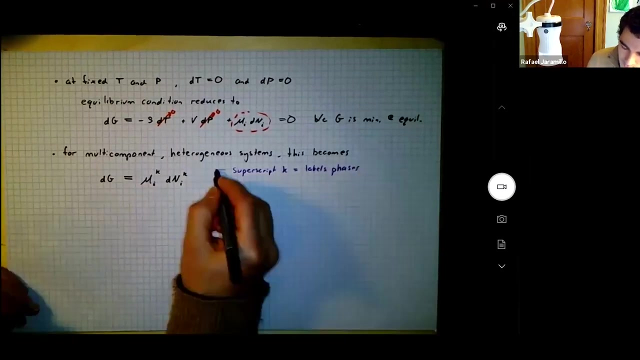 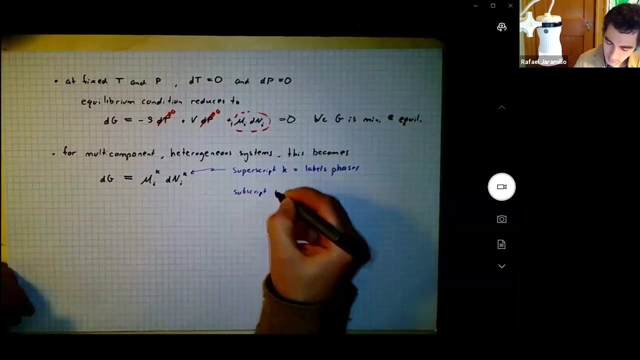 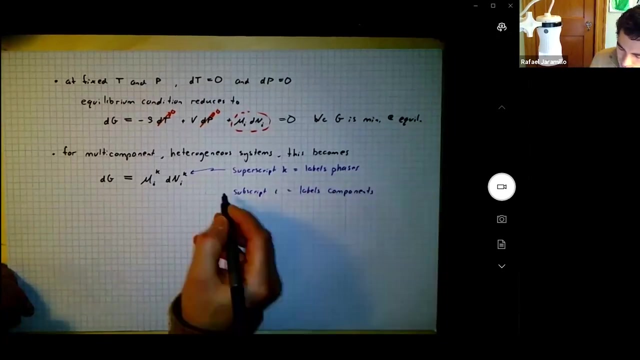 heterogeneous systems. This becomes dg sum over i component k, dn, i component a, Introducing a new notation here: Superscript labels phases And a subscript labels components. So now we can picture something in our minds. We have a phase boundary here. 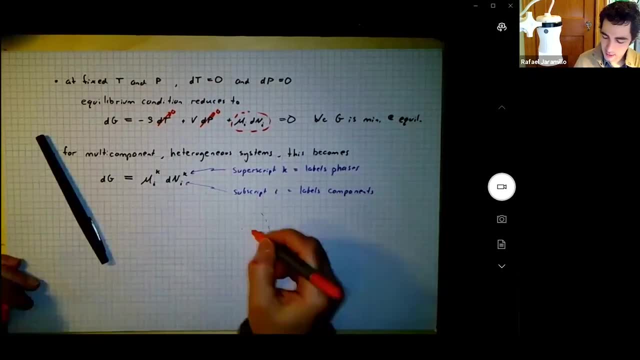 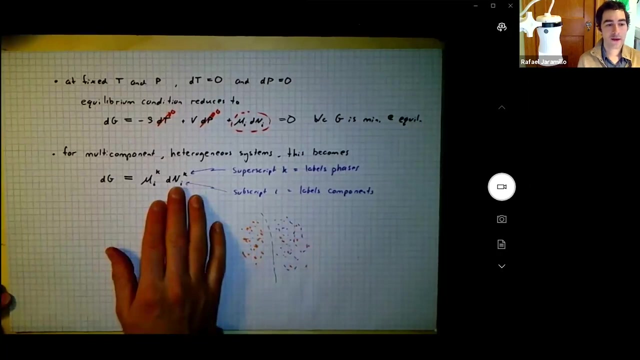 Two phases And each phase has two components. This was a purple-red phase and this was an orange-red phase- And evaluating the equilibrium condition is going to come down to knowing how the components can exchange between phases And what the effect of that exchange is on a chemical potential. Let me write that out. 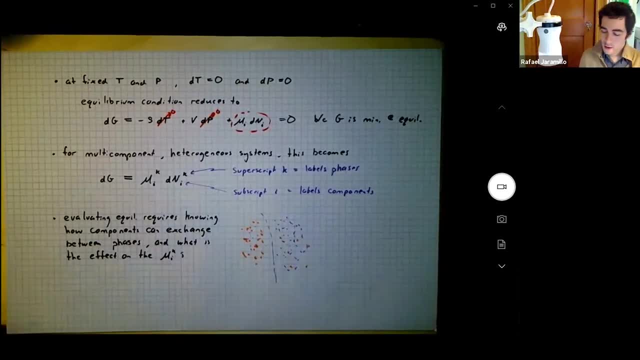 Okay, what determines whether or not components can exchange between the phases? It's the boundary. So the property of the boundary tells us what components can exchange between phases, And that can be engineered. So there's a lot of engineering around choosing boundaries to get the desired equilibrium condition. 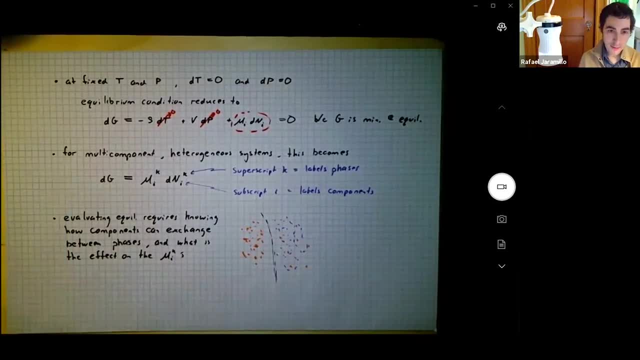 So much of what comes later in this class is calculating composition dependence, Calculating composition dependence of those chemical potentials, and we're going to develop models for that and graphs and formulas in a way. So there's a lot of work going on here. graphical tools for that. 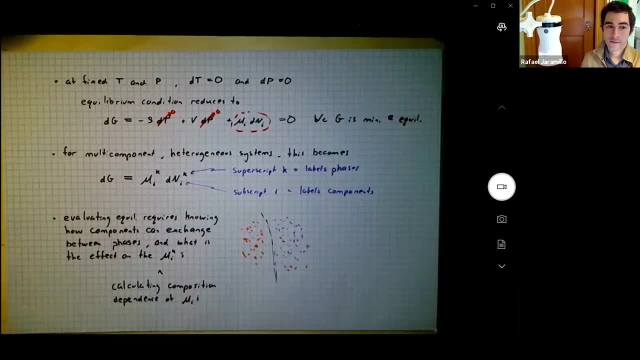 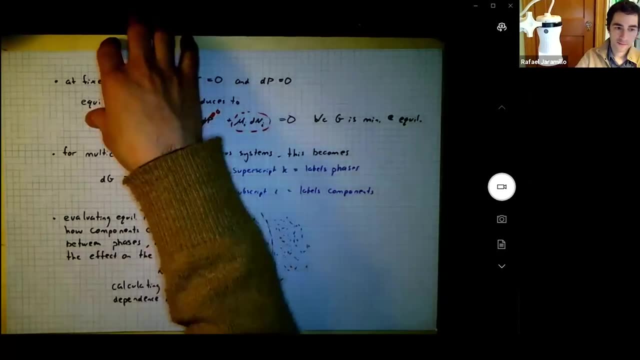 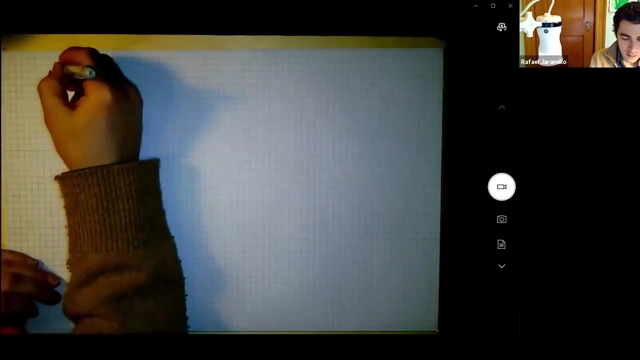 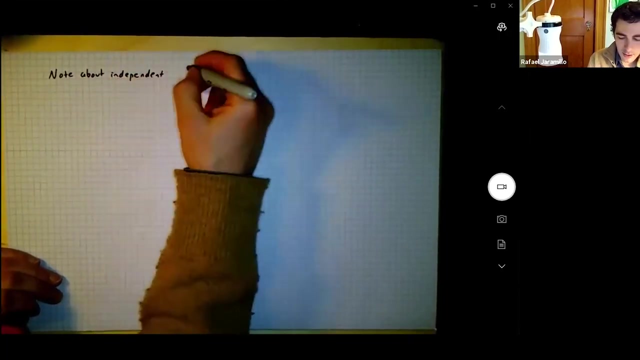 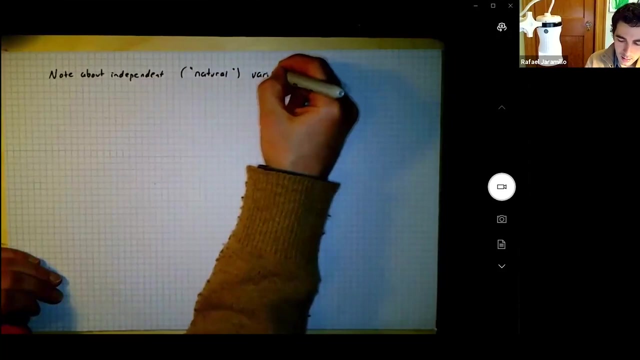 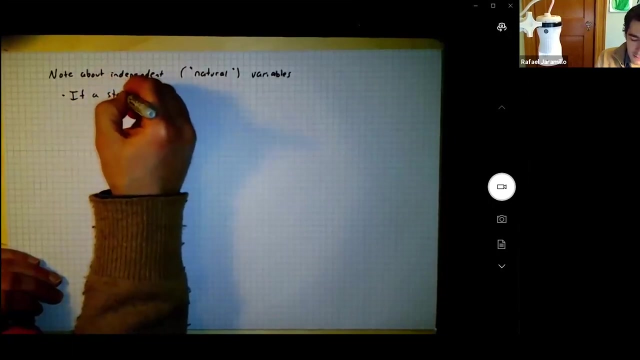 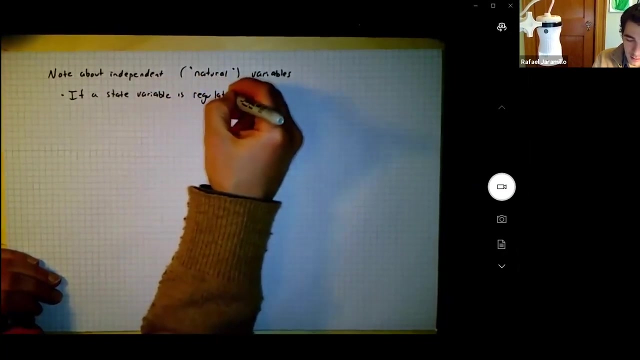 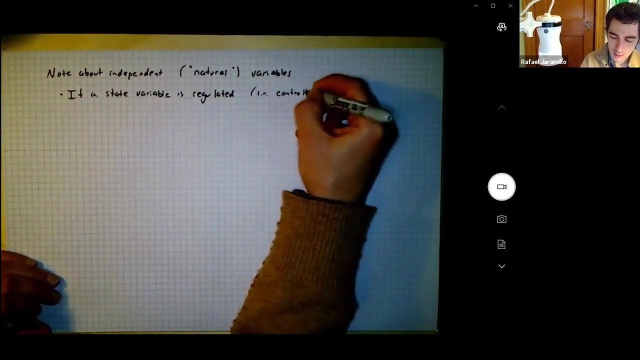 finally leading to binary phase diagrams. All right, one last note. I'll do one last note about independent variables, Sometimes called natural. If a state variable is regulated, Regulated, what does that mean? Controlled Regulations or controls? If you go to a McMaster car, 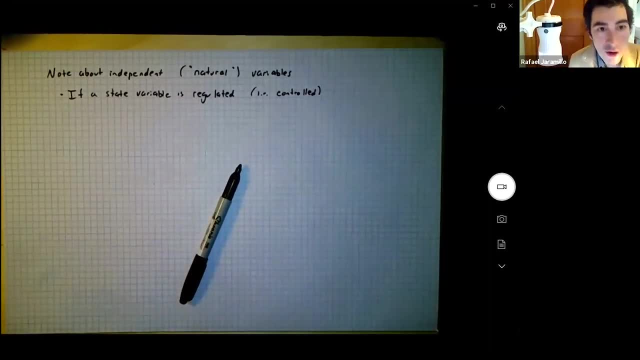 you can buy a regulator for pressure If you go to Home Depot. you can get a regulator for temperature- we call it a thermostat- And those things that you would buy of analogs in not the real world, but in R&D and material science as well. 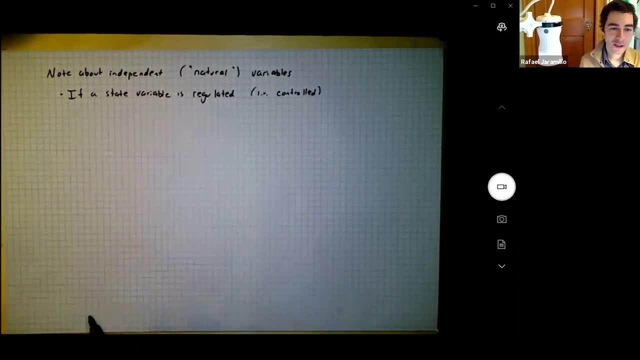 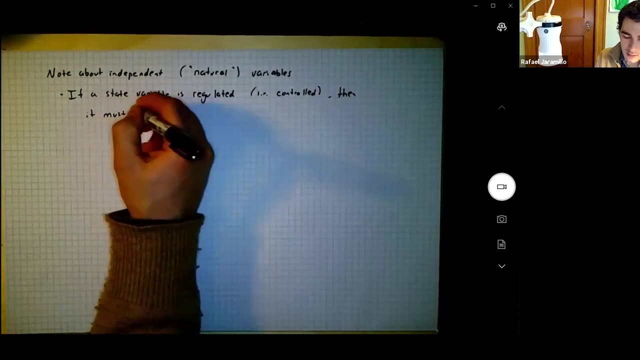 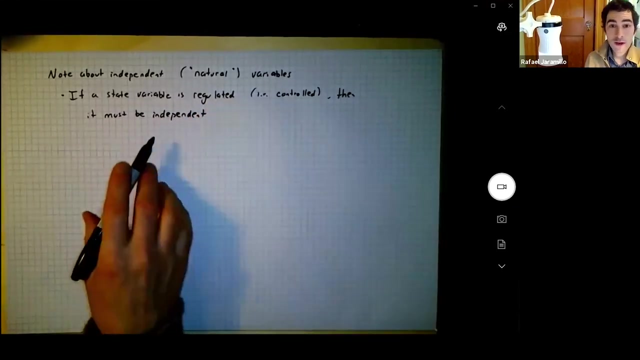 If a state variable is regulated- that's why I'm using that term, because it'll help you in the future- If it's regulated, then it must be independent. So choosing your independent variables is one of the major intellectual challenges of Thermo. 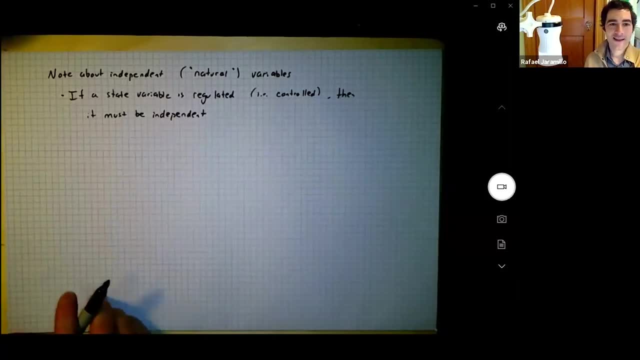 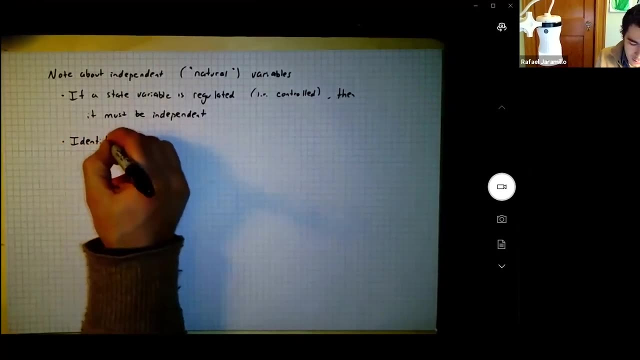 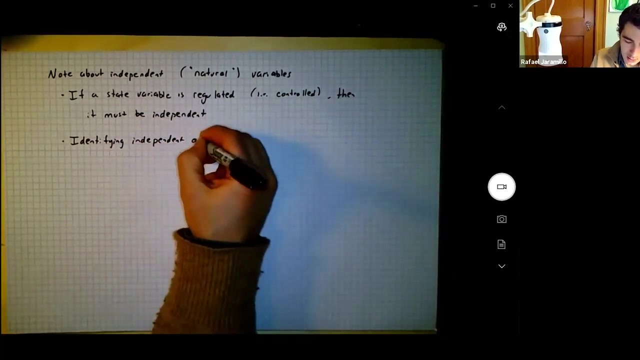 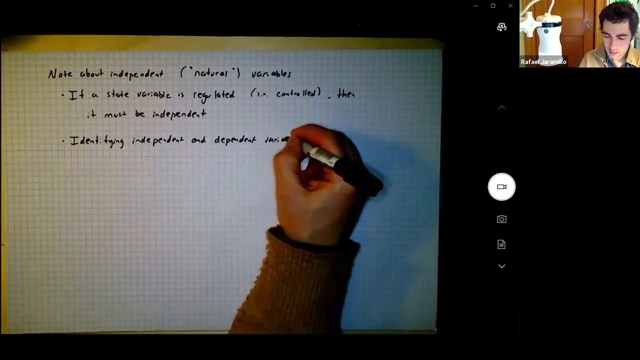 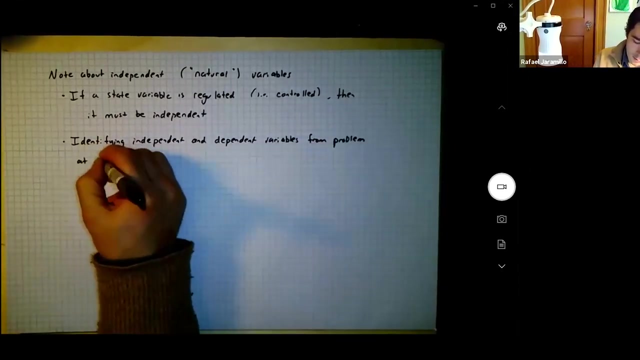 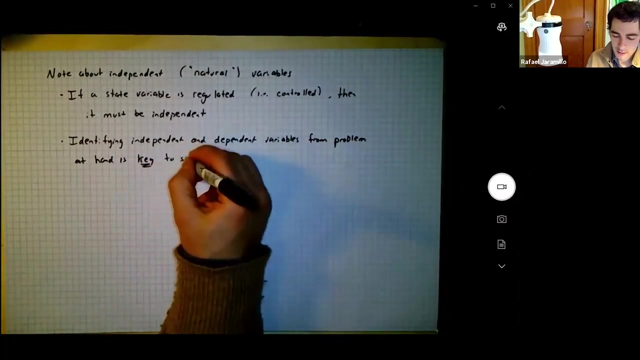 It helps even know that that's the challenge you're facing. Knowing that that's the challenge you're facing, it gives you a good start, Identifying independent variables and dependent variables from the problem I hand. that's key to success. So, for example, 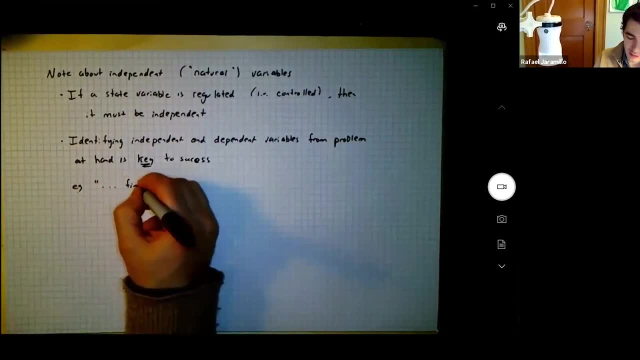 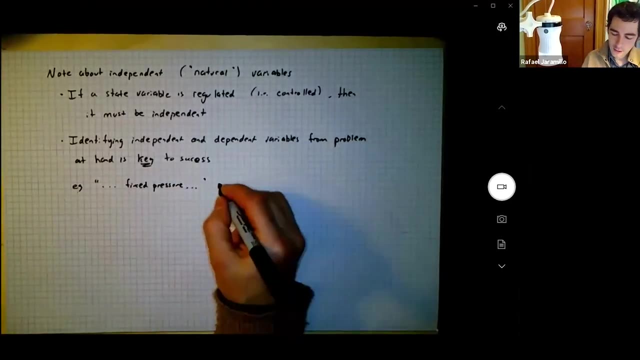 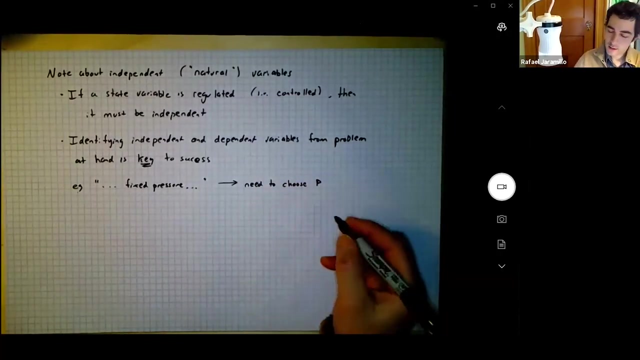 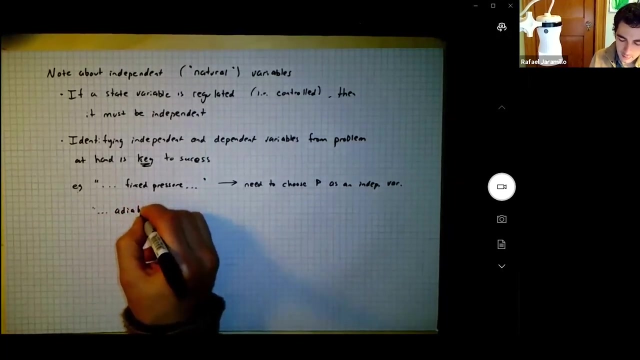 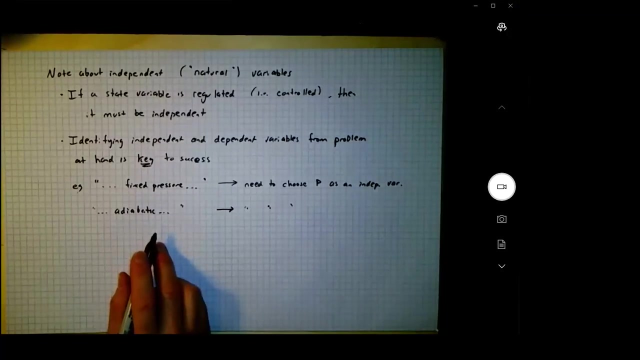 if the problem statement says something about fixed pressure pressure, then you need to choose pressure as an independent variable. If the problem says adiabatic, you need to choose what. What should be your independent variable? if the problem statement said adiabatic, What should be one of your two independent variables? Entropy, Yeah. 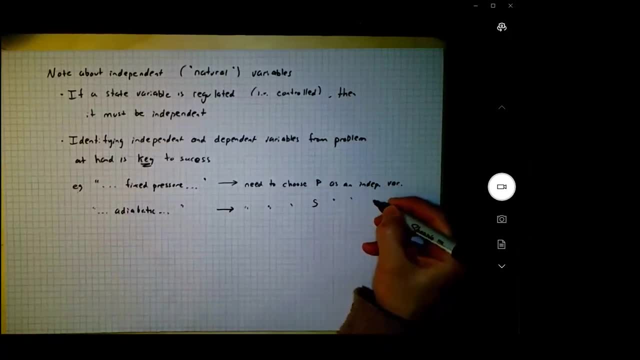 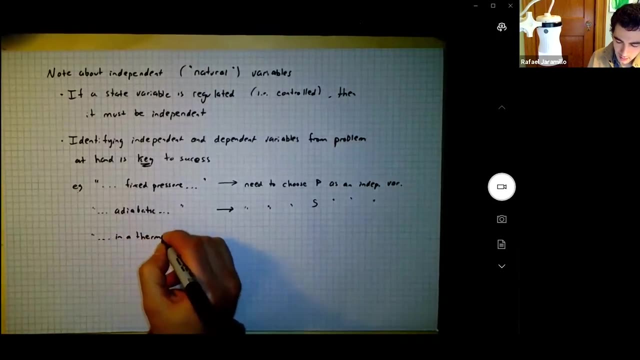 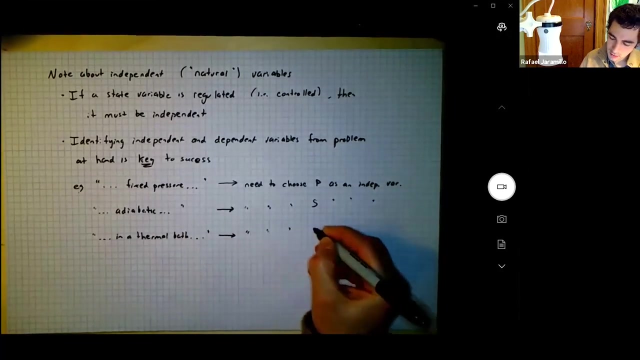 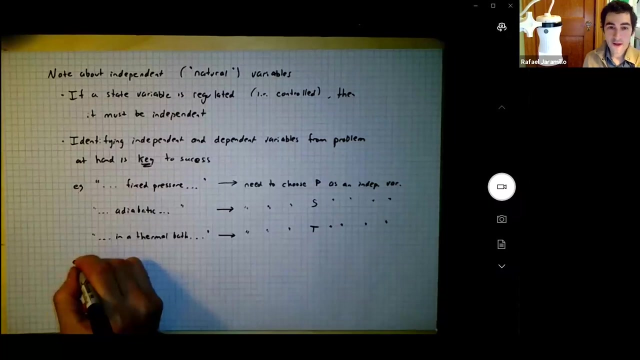 entropy, And if the problem statement says in a thermal bath, then you need to choose temperature as one of your independent variables, and so on. So this is like a key for turning problems that you encounter in problem sets or in the real world into things you can solve using thermal.